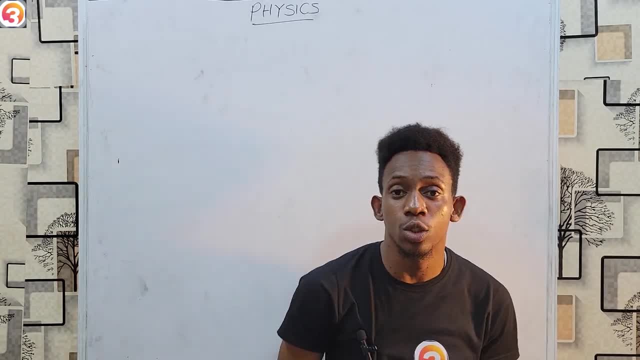 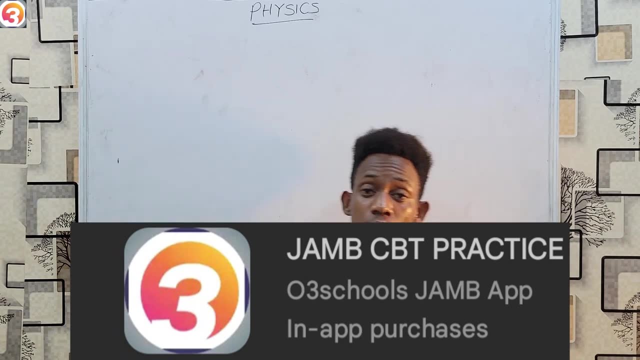 Hello and welcome to this class presented to you by O3Schools Jam App. Now, O3Schools Jam App is simply an application which you can install on your Android phones or your Windows laptops, And what it does is that it gives you access to a bunch of features and a variety of options which you can use while preparing for your Jam. 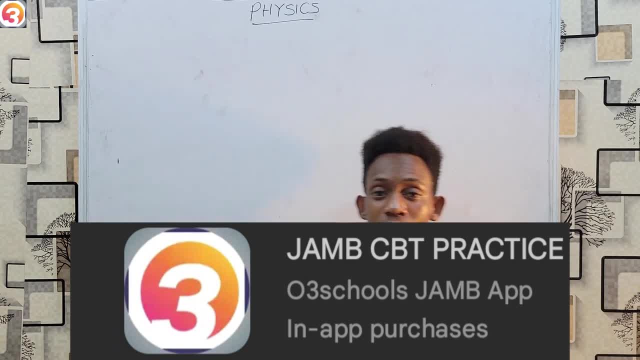 For instance, it has the mock exam feature in which you can set your system and it appears just as it would when you are writing the UTMA examination. That means for those of you who are not sure how your computer software will look like when writing Jam. 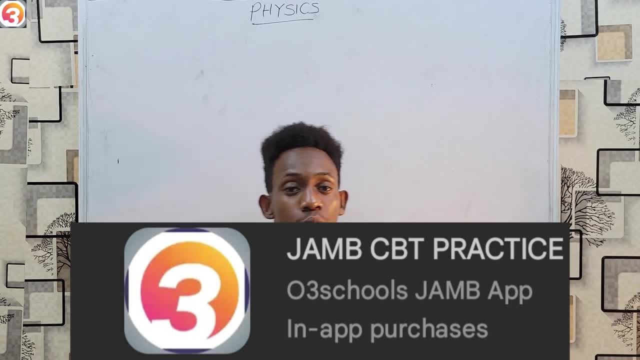 using your O3Schools Jam App, you can actually get an accurate picture of that and can then try practice writing your exams to see how your score would be, And you can try to be able to guess or measure your improvement as you read and read and get better. 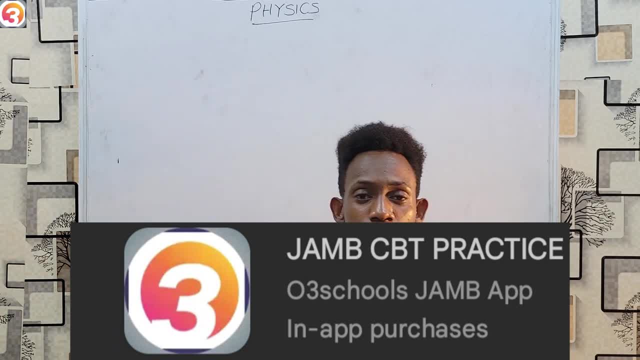 It also has other features, like it has the places where it can advise you on what subjects to take for a particular course or whether different universities offer different courses, And my personal favorite is the feature in which you can try to search for questions by topic. 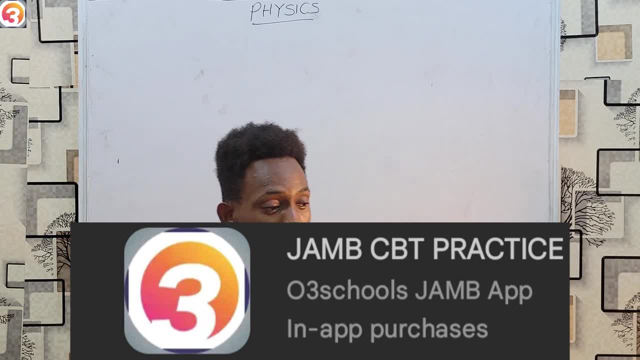 That simply means that once you finish reading up a subject or a topic, rather in a particular subject, you can just go to the app And search for that topic, Such that it will give you all the questions Jam has set on that topic, And so you can actually read, answer and be able to know how well prepared you are per topic, not just per subject. 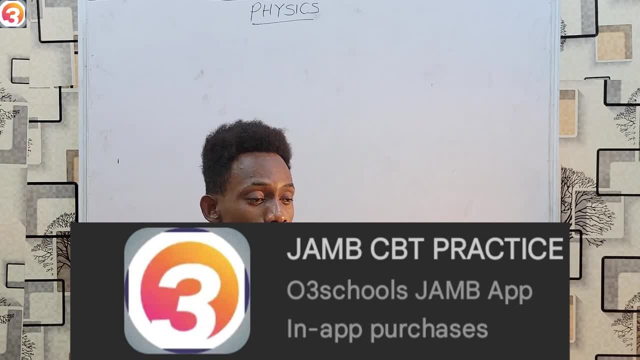 So, as you begin to finish each topic, you can actually go there, see all the questions, read them up and actually be able to improve. Now, how do you get your app? You can simply download it, But after downloading you will need to activate this app. The activation fee costs $2.00.. $2,500 only, And it is very, very simple and easy to do. Simply follow the steps there. There are three different methods of payment. Pick the one suitable for you And simply proceed with your payment. 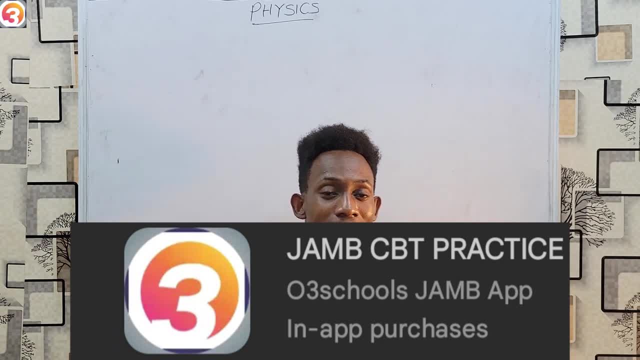 Once you can complete your payment, your app will be activated. You can be 100% sure of that. We do not fail when it comes to that. So that's how it works, And without much ado, let's go back to today's topic. 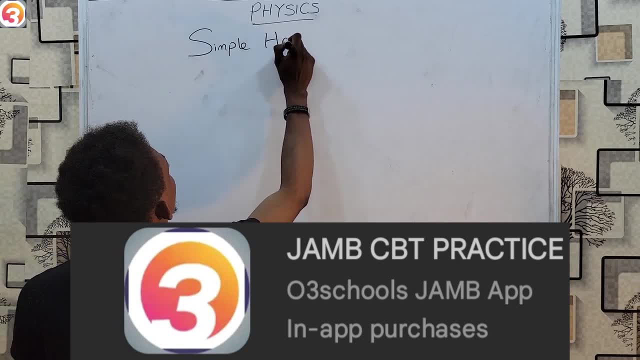 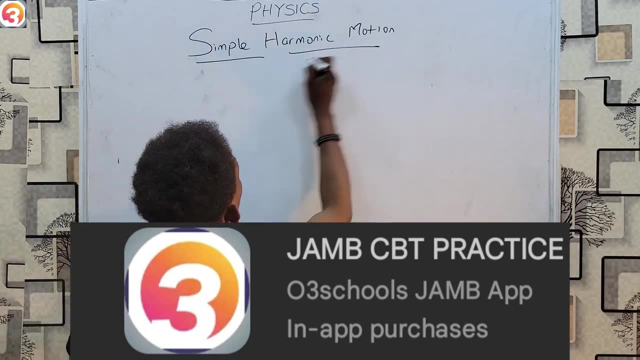 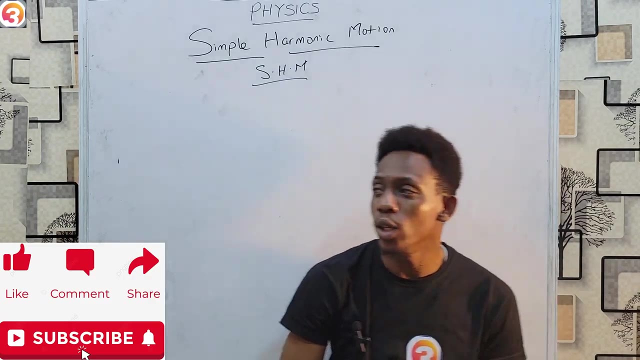 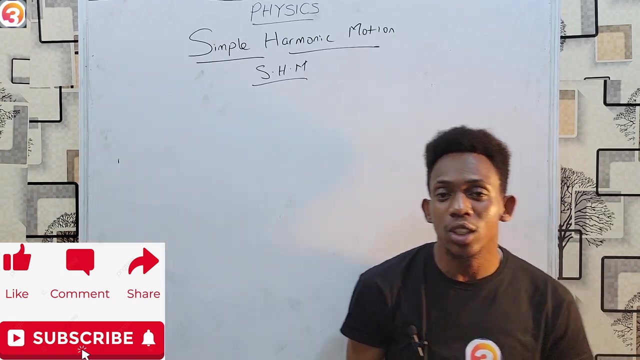 You should be looking at simple harmonic motion, Also popularly known as SHM. Now in simple harmonic motion. what is going on In simple harmonic motion? this is simply the motion of an object, Or you may call it the periodic to and fro repeating motion of an object. 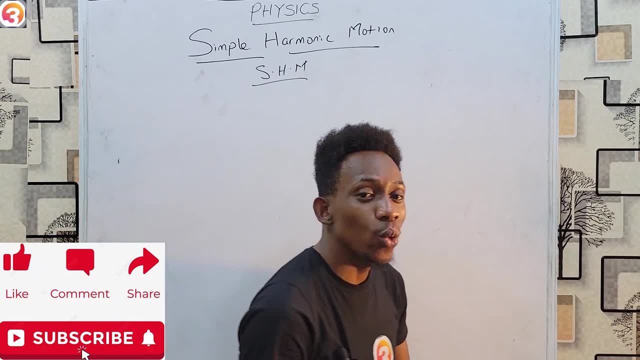 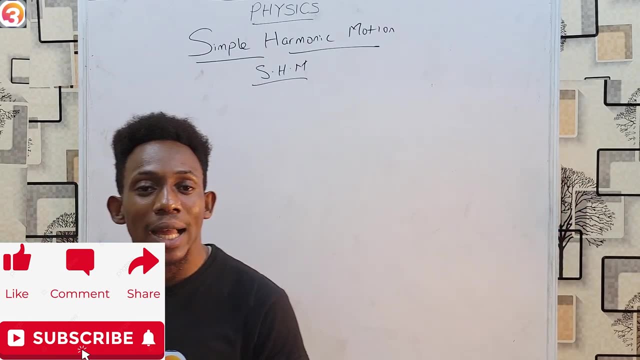 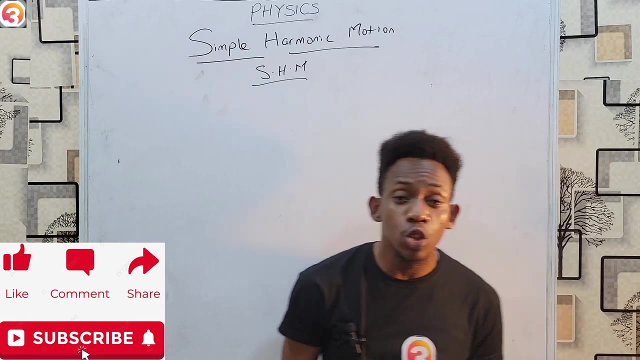 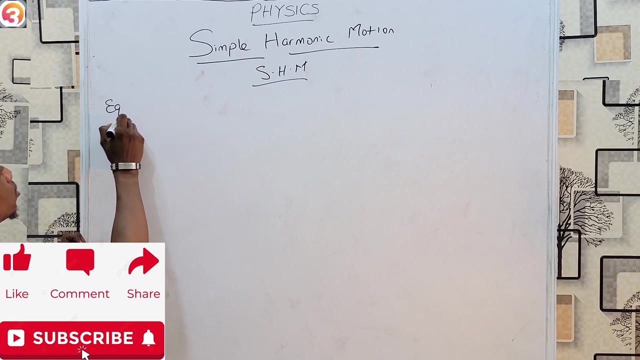 Such that its acceleration is always directed towards a fixed point And is proportional to the displacement from that point. One more time: Acceleration is proportional to the displacement from a fixed point And it is also directed towards that point. That point is referred to as the equilibrium position. 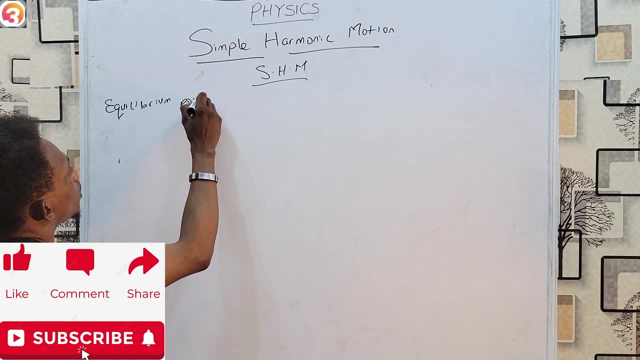 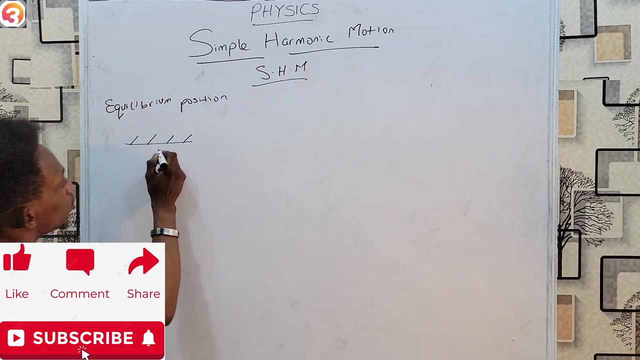 Equilibrium position. Now, the easiest way to describe this pictorially is by using a simple pendulum. This is the natural state of my pendulum If I was to take it and let it swing or slid freely. these are different stages in flight. 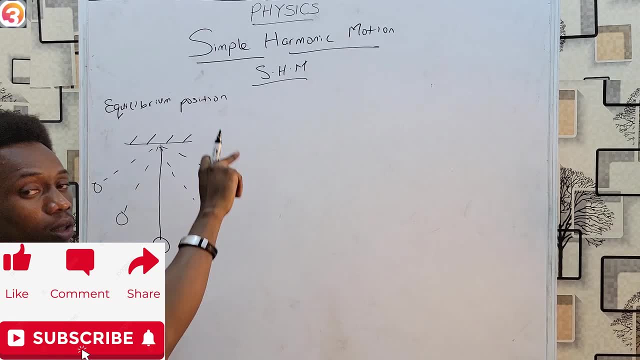 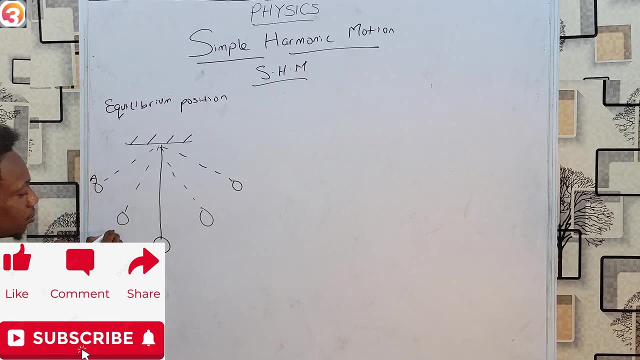 Now, as my pendulum is swinging to and fro, what's happening, Please note. let's start from year A, B, C, D and E, As it is at year A. one thing you must please notice is that it is not yet moving. 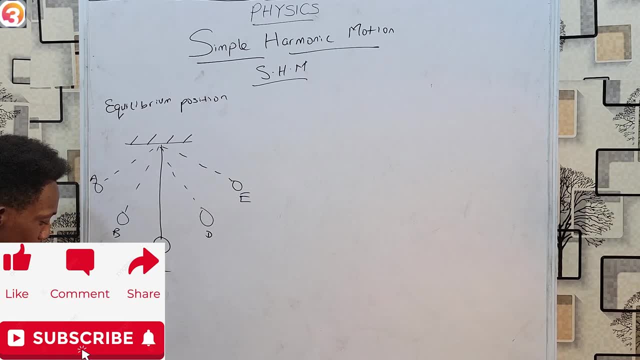 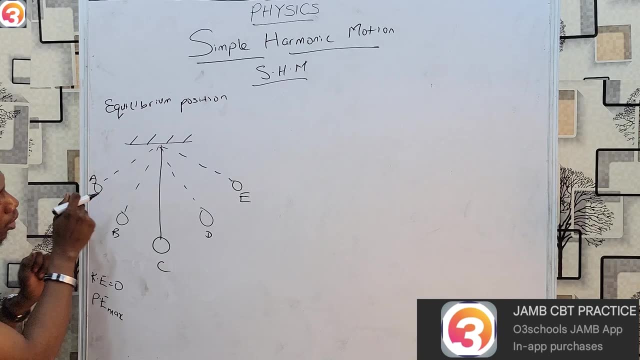 So the kinetic energy will be zeroed, While the potential energy is maximum. So what happens to this? As it is at this point, it always wants to come to this equilibrium point, So the acceleration is directed towards that point. 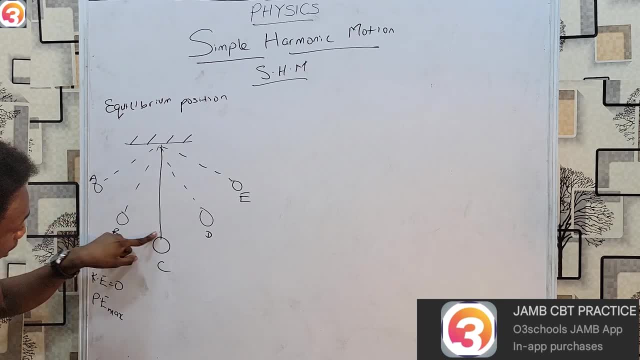 And proportional to the displacement from that point It is facing the air And is proportional to how far it is from here. So the farther it is, the more the acceleration, Which it means simply that the acceleration is maximum at this point. 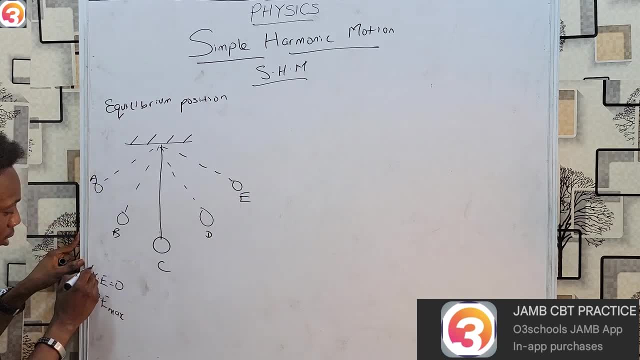 So A and E have similar properties. So please note, A and E have similar properties, both ends. So what happens? Once this object is free to move, it begins to move. this way, The potential energy starts getting converted into kinetic energy. 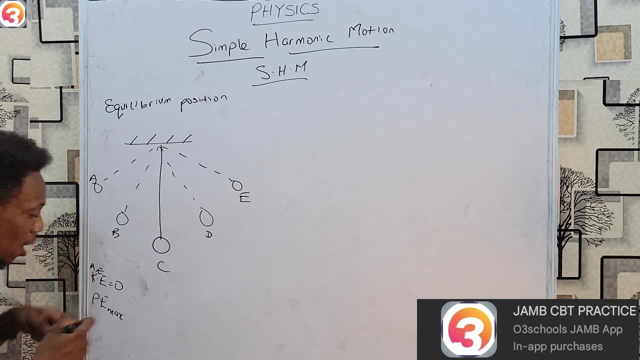 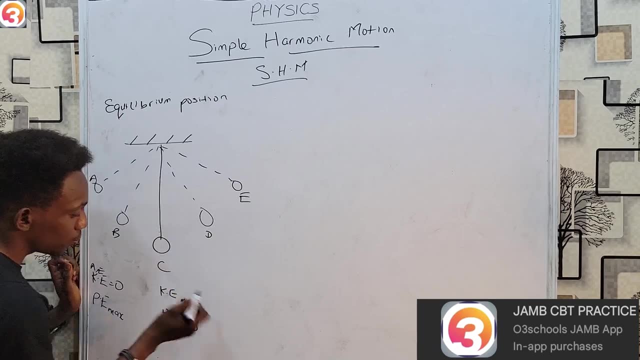 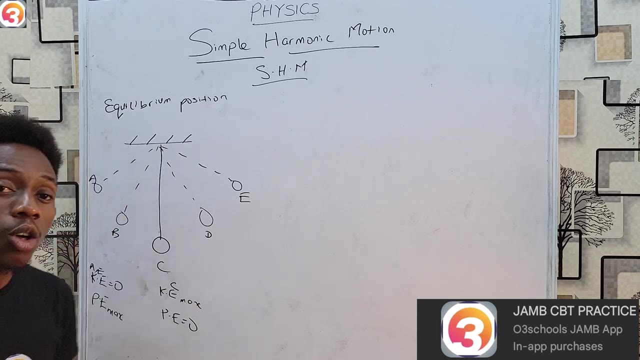 until it gets to this point here. At this point kinetic energy is maximum And potential energy is zero. This is at C. Ke is maximum. Now what happens when kinetic energy is maximum? That also means that the velocity must be maximum. 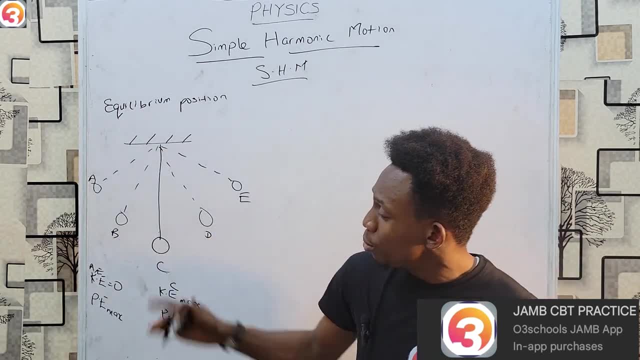 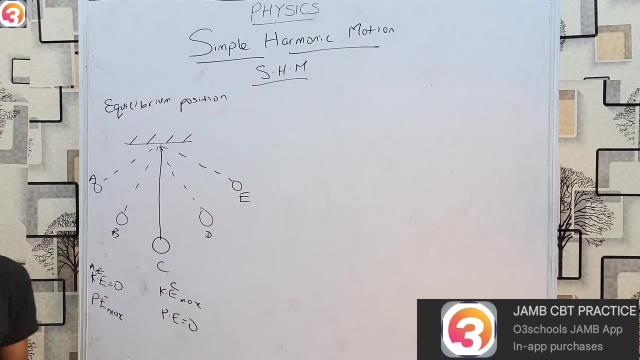 But now here is the point: Because velocity is maximum, this object wanted to get to this point, So once it gets here it seems to want to stop. But maximum velocity is not easy to do, so You have to decelerate. 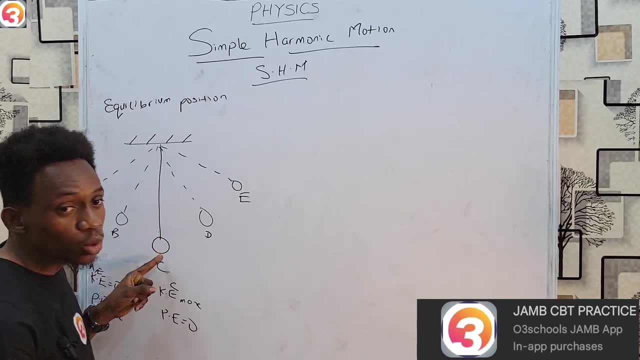 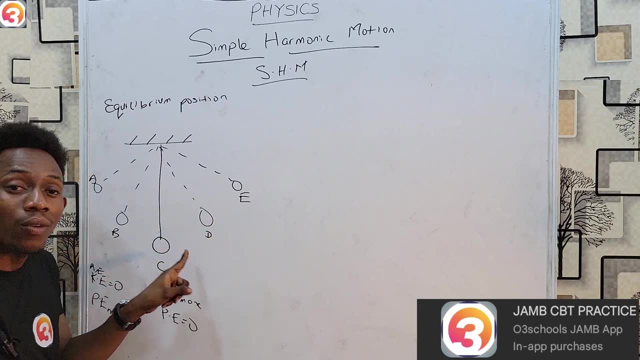 You have to decelerate first. That means, as this body begins to pass here, because it cannot stop instantly, the acceleration begins to tell it: no, come back here. Which means the acceleration is now, instead of acceleration, moving it faster. 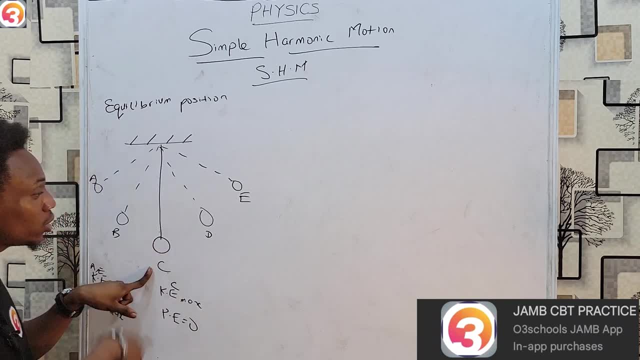 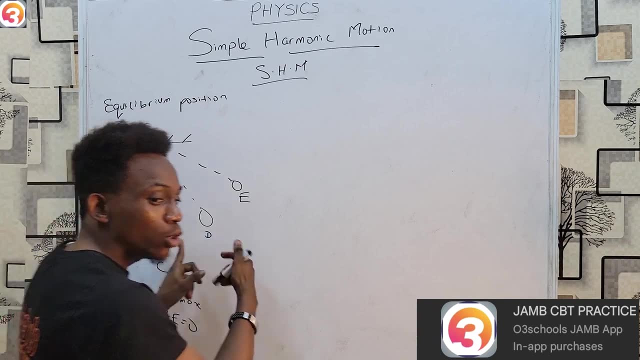 is now retardation trying to stop it. So the acceleration will act on it and try and stop it, but doesn't quite succeed Until this body passes all the way from here and until it finally succeeds in stopping him. 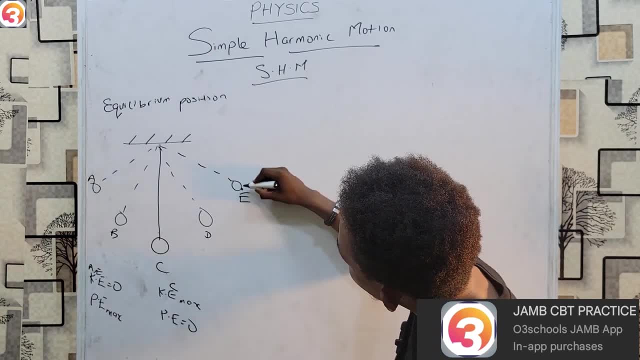 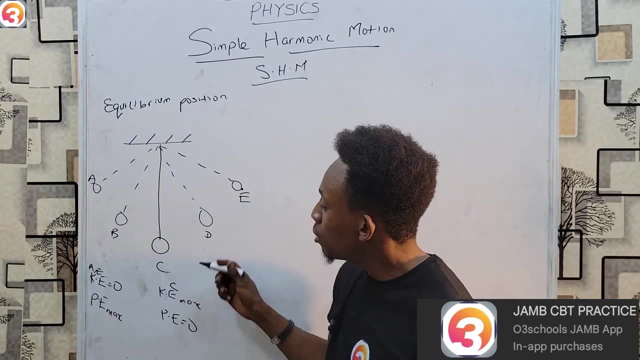 after it has gotten to this point. at this point the velocity becomes zero again and the body stops. But once it stops, remember, the acceleration is always facing this equivalent position, which means instantly it tells it. 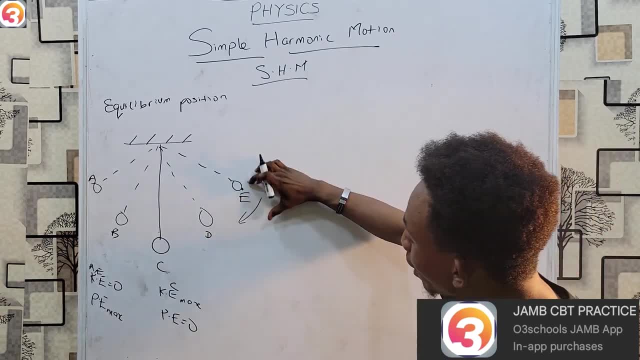 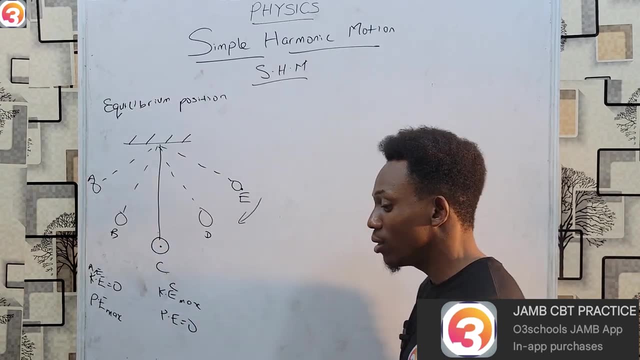 please come back here. This is where we want you. So again, the body tries to move. The more it moves, the faster it gets, until it gets here again. Once it gets here again, it attempts to stop. 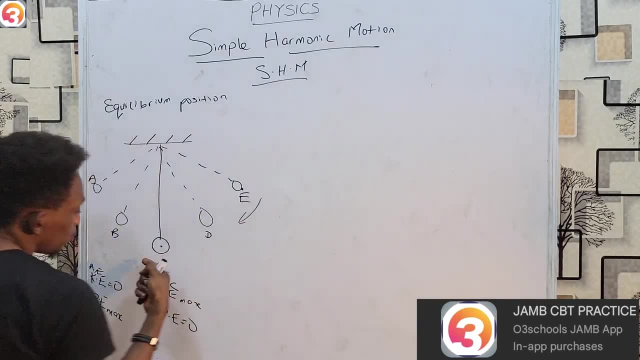 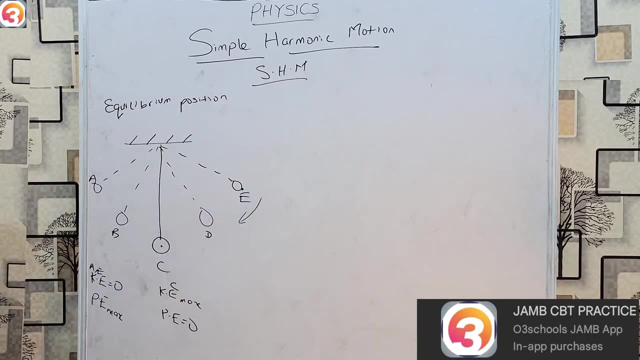 But again, stopping is not that easy, So it overshoots it until it is able to stop at here And it keeps on doing that, ideally forever and ever, Which means, please note, there are three types of vibration. 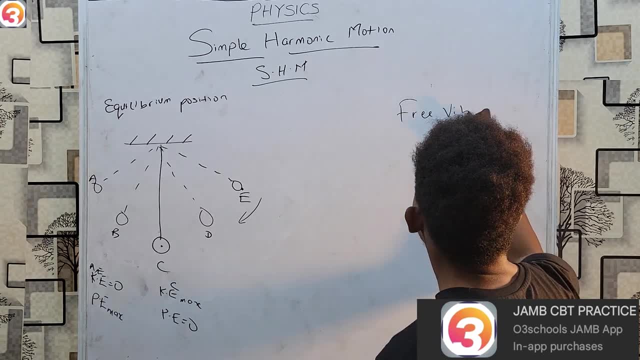 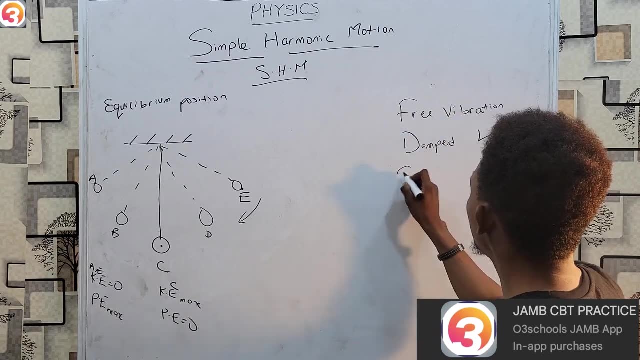 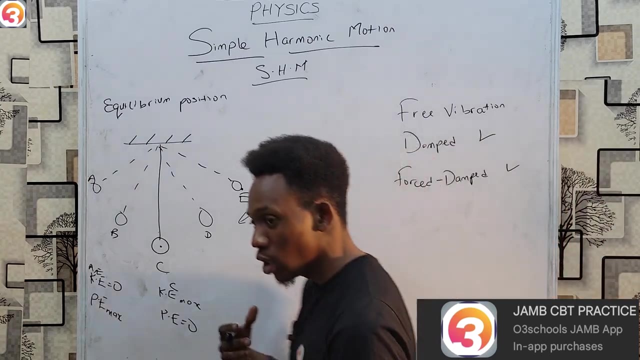 There's what we call free vibration. It's also known as undamped vibration. Then there is damped vibration And there's what is now also called forced damped vibration. Now, what are the differences In free vibration? this object doesn't express frictional force. 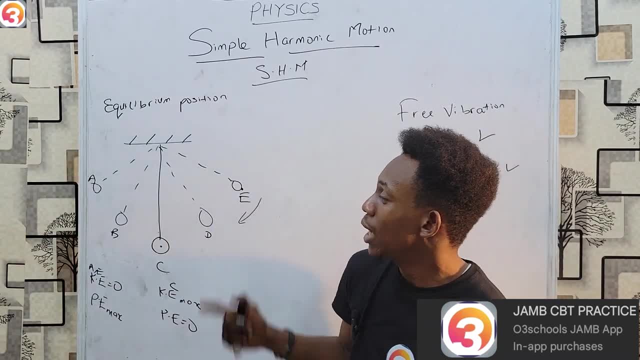 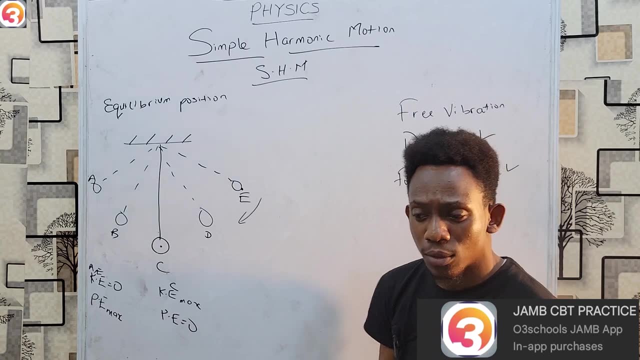 So there's nothing going to stop it. That means this pendulum ideally should move forever and ever without stop. But in real life you'll notice, that doesn't happen. You don't have any object oscillating forever. 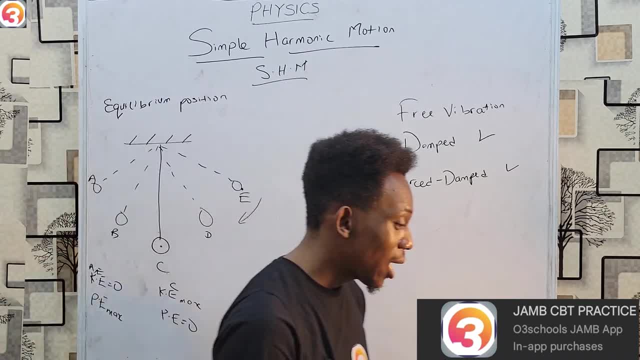 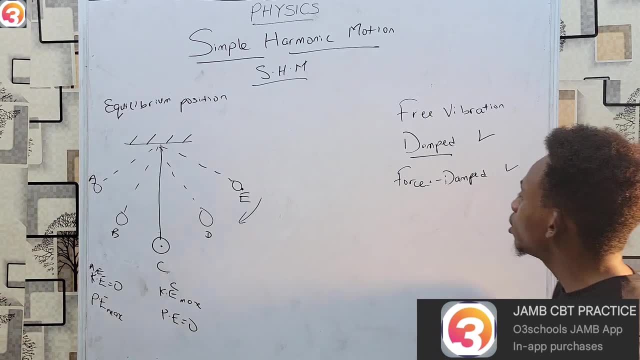 What stops it? Things like air resistance and frictional force, And that's what brings us to damped vibration. In damped vibration, there's a stopping force, which means that my object cannot move forever, but instead gradually begins to slow down. 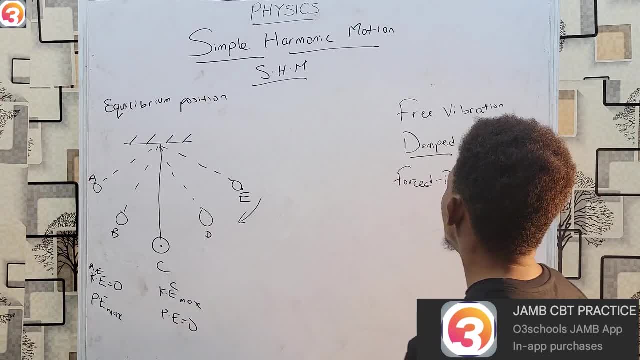 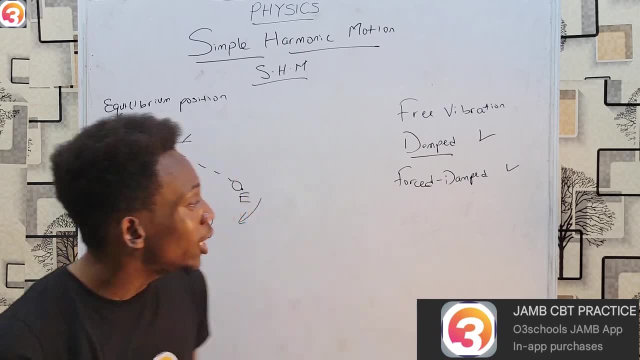 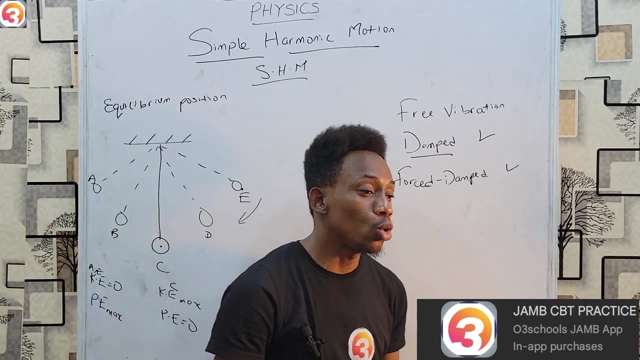 Which is what we observe normally in real life. But then we now have forced damped vibration. In forced damped vibration the aim is to keep it in harmonic motion, just like free vibration, But it does this by applying a periodic force to the object. 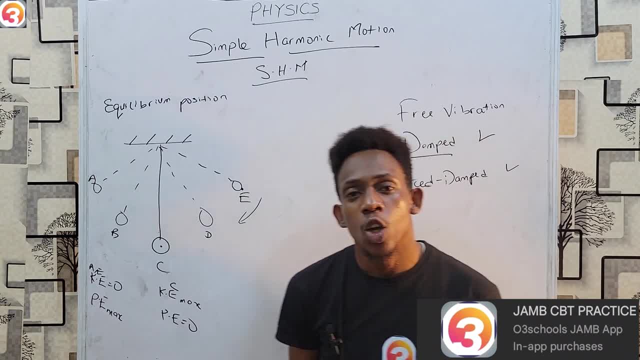 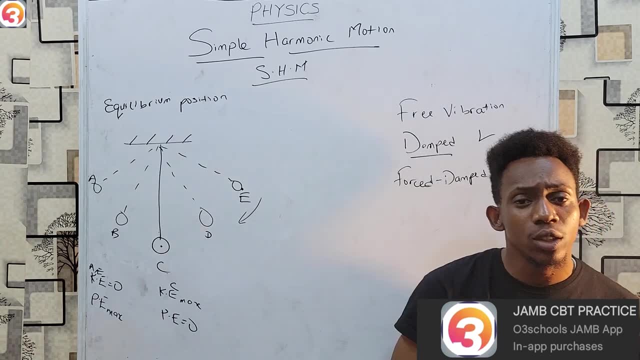 Think about it kind of like your swing. When you're on a swing, initially you can push yourself off and begin to swing, But eventually you must stop. How do you avoid stopping? By having someone behind you who pushes you. 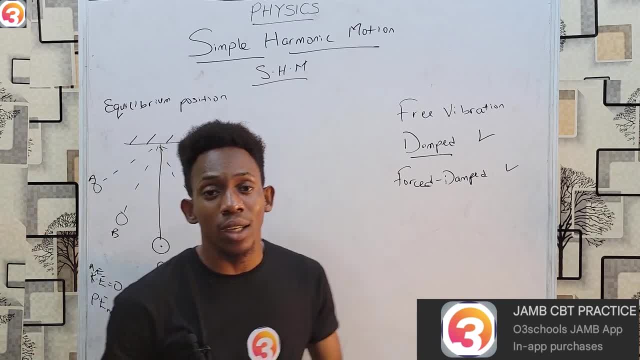 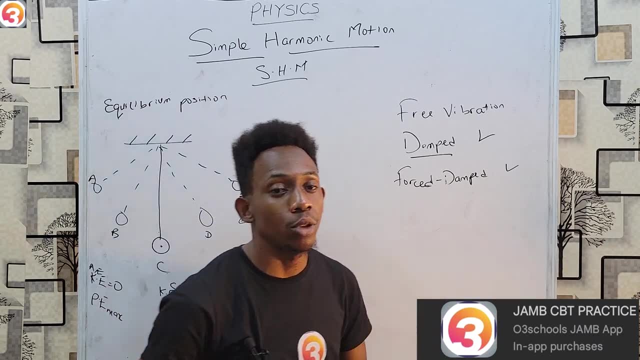 every time you get there. By so doing, you're trying to never end up stopping. Instead, you begin to oscillate over and over again as soon as the patient keeps on applying that periodic force. Now at the level for jump. 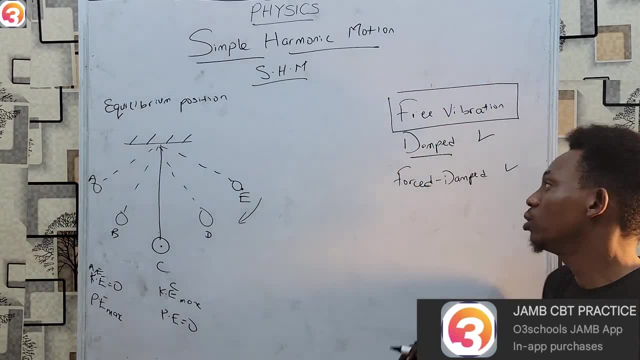 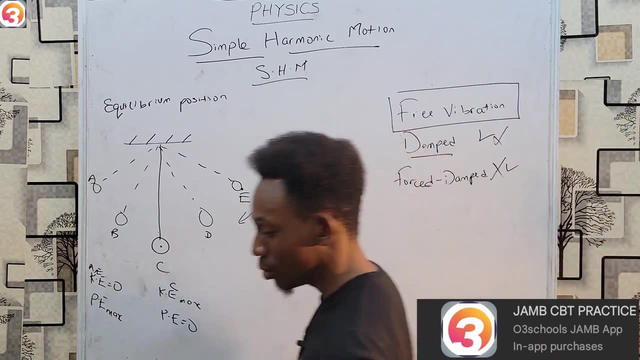 we're paying attention only to free vibration and totally neglecting damped and forced damped. We're able to focus on free vibration Now. before we can do much analysis on free vibration, we must first of all remember certain terms. 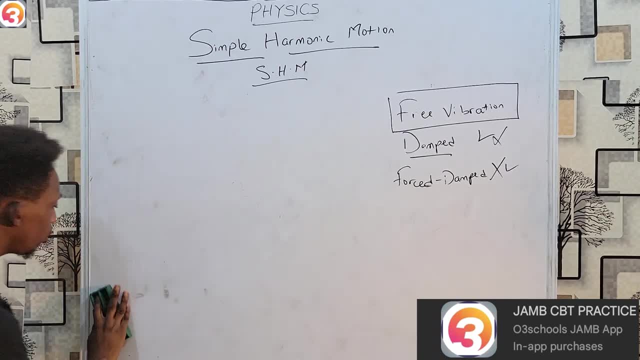 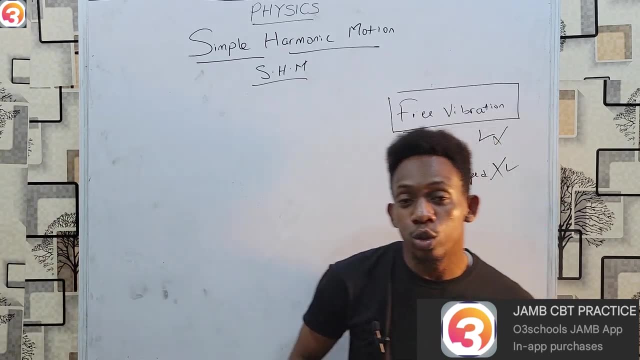 that will get used a lot in this topic And a lot of these terms have things to do in common with waves. So if you know waves, these terms should not be familiar to you, And if you are to do these before you do waves. 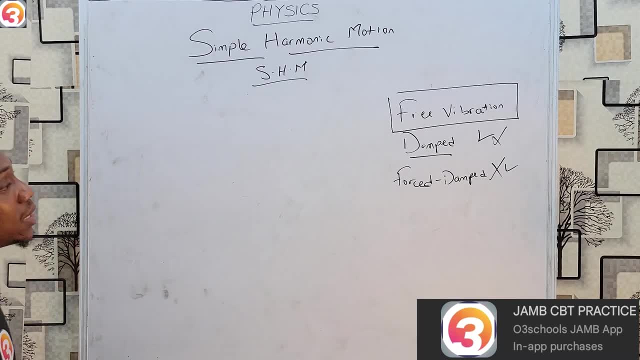 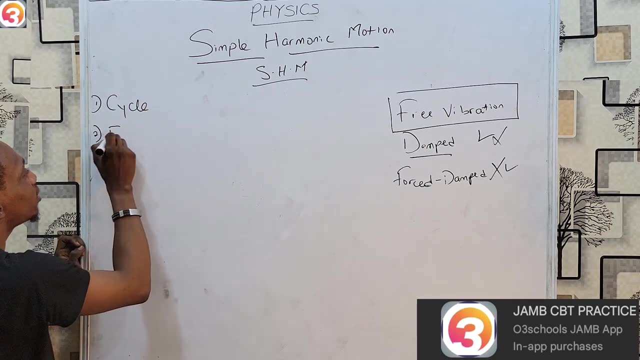 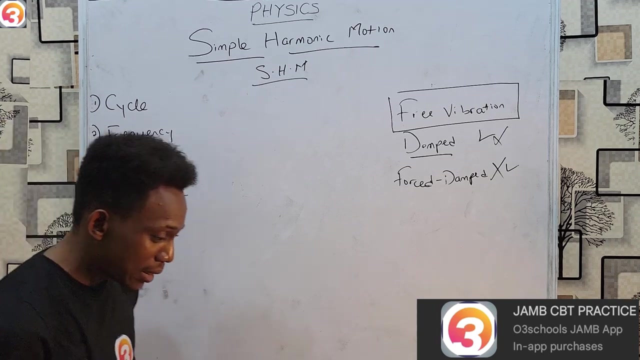 when you get to waves, those terms will also not be unfamiliar to you. For example, we have a term known as cycle. We have frequency, We have period, We also have amplitude. Now, what is a cycle? Basically, in a cycle, 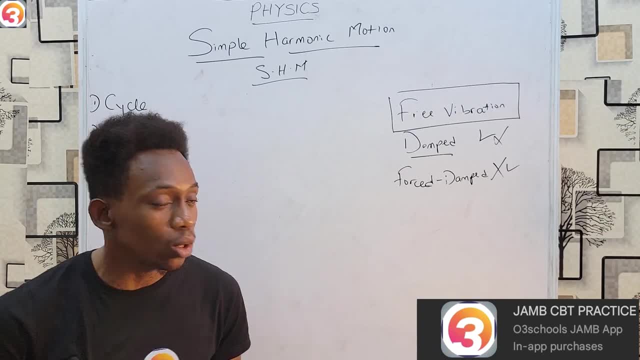 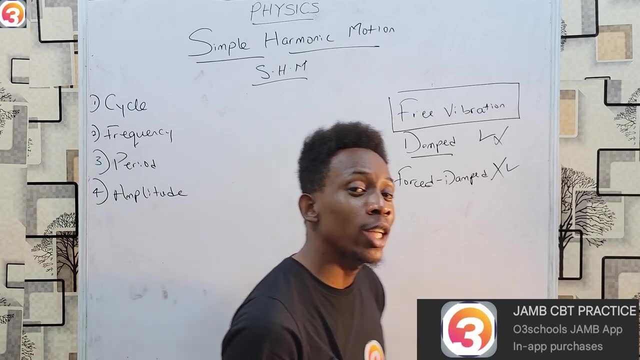 a cycle is one complete toe and foot movement of the oscillating body, Which means, please note, a cycle is not the same as a circle, But a cycle can actually be a circle One more time. There is a cycle and then there is a circle with the shape. 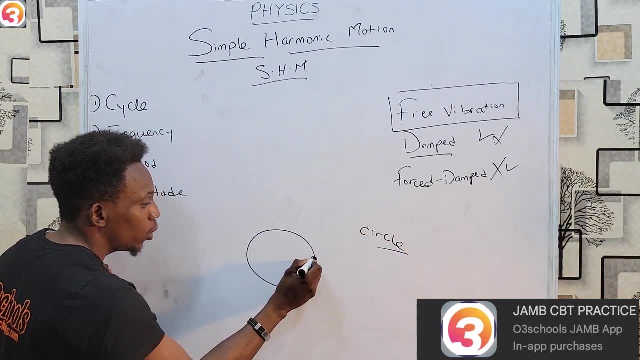 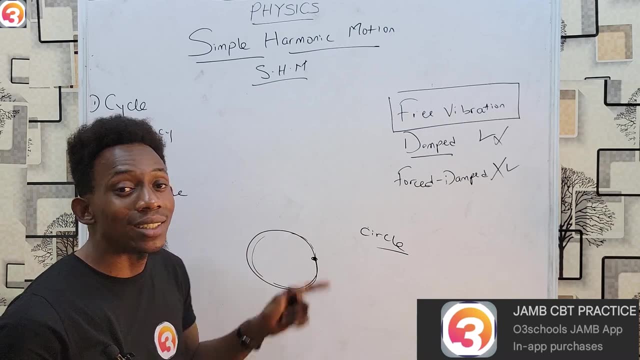 If we have an object moving around in a circular path when it has gone around once, that is a cycle, yes, But however, it doesn't always have to be going around in a circle to give you a cycle. If I have my oscillation, like we saw, of the pendulum, 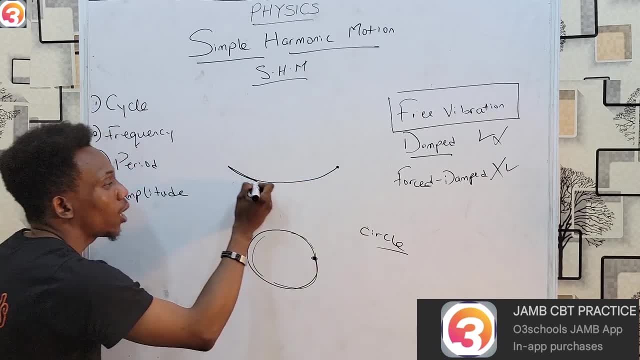 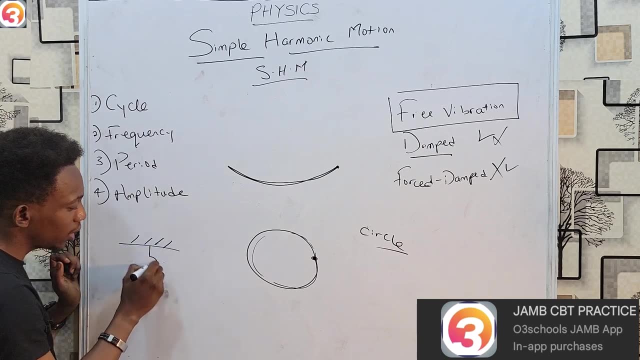 if it starts from here, if it goes this way and comes back. that is also a cycle. If I'm to use a mass, a spring, and the loaded mass, for example, if I was to drag this body and release it. 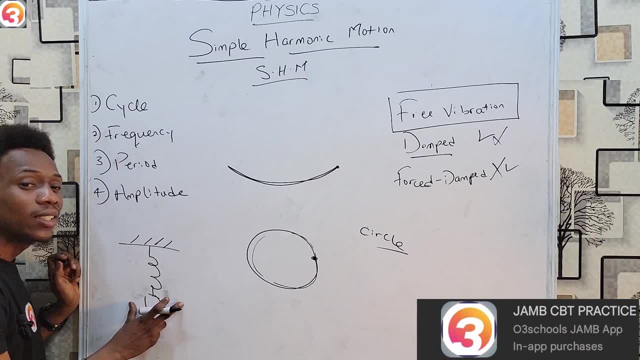 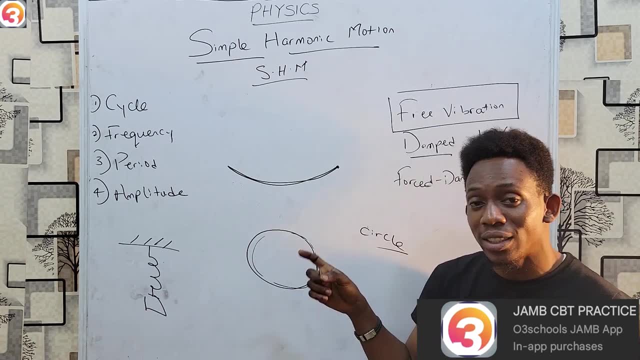 it needs to go up and down. When it goes up and down once, that is also a cycle. So one more time: a cycle can be a circle, but a cycle doesn't have to be a circle. It could also be this: 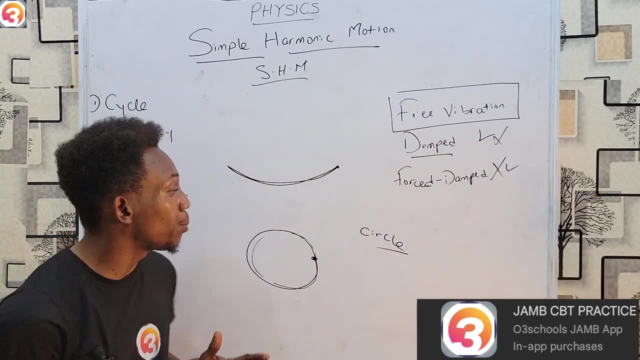 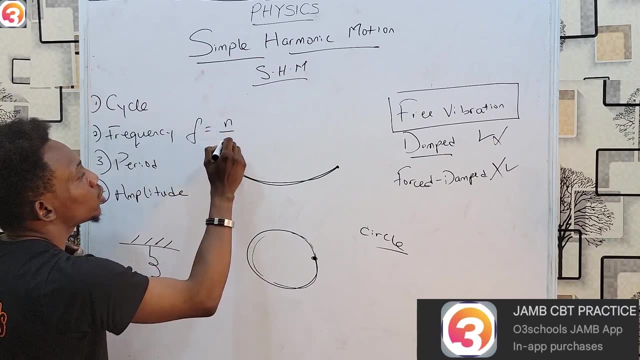 So let's start going around the oscillation path. once we have a complete cycle, Then next we have frequency. Frequency simply measures how many cycles you can complete in one second. The number of cycles over time. 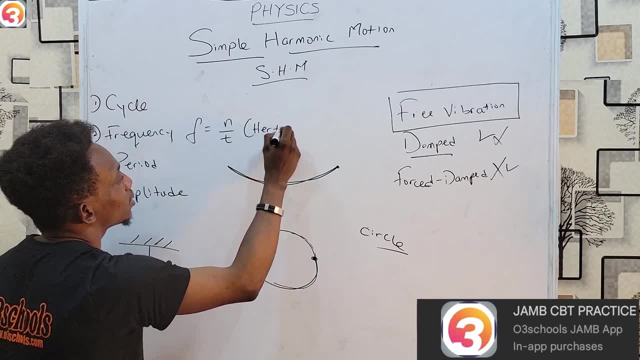 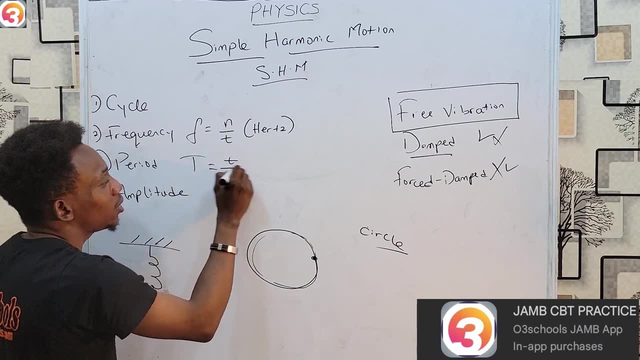 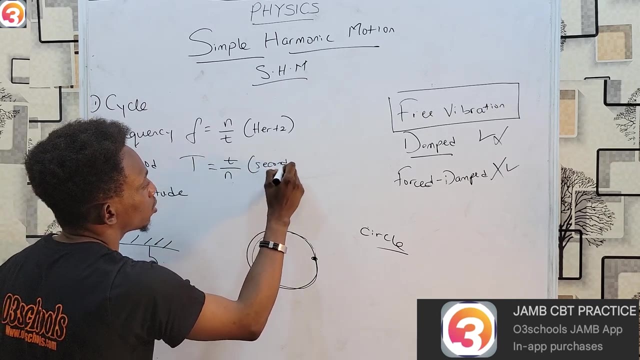 And frequency is measured in hertz. Then next we have period. Period is simply the time taken to complete one cycle- Time taken for one cycle- and is measured in seconds. Now, with a little bit of observation. 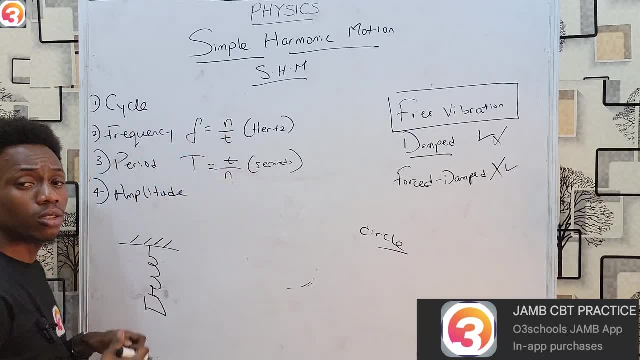 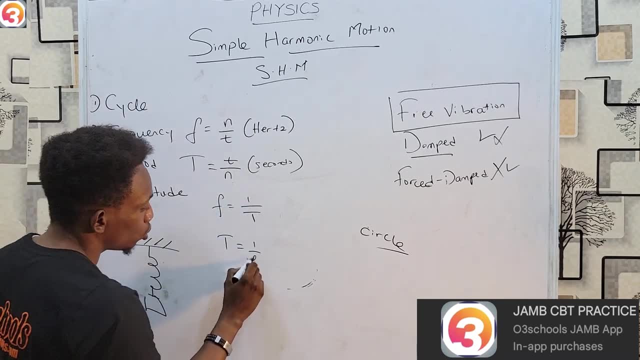 realize that these two are almost the same, just reciprocals of each other, Which means that f equals one over period and period is also equals to one over f. Then the last term we are going to look at here. 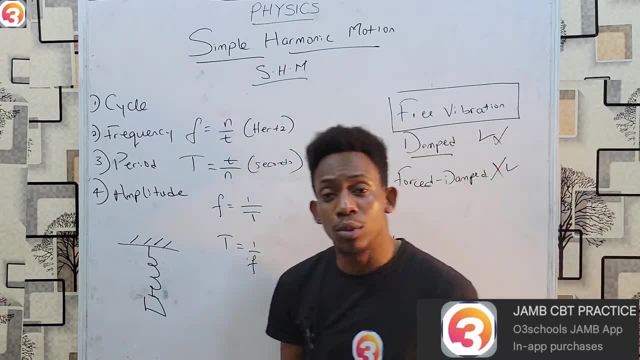 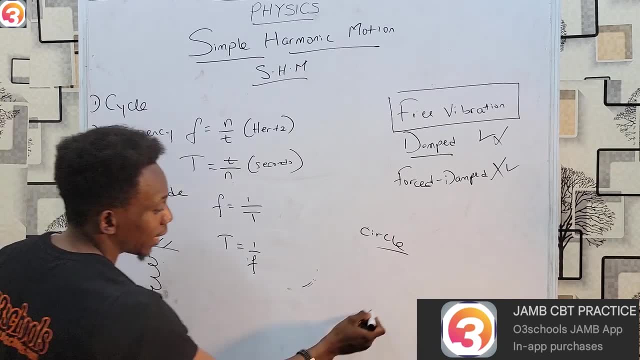 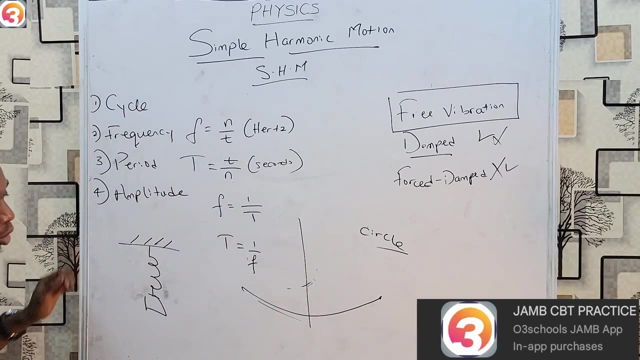 which is amplitude. Amplitude is the maximum displacement of the body performing SHM from its equilibrium position. Like in the case of a pendulum going to the ends, the equilibrium position is this middle. 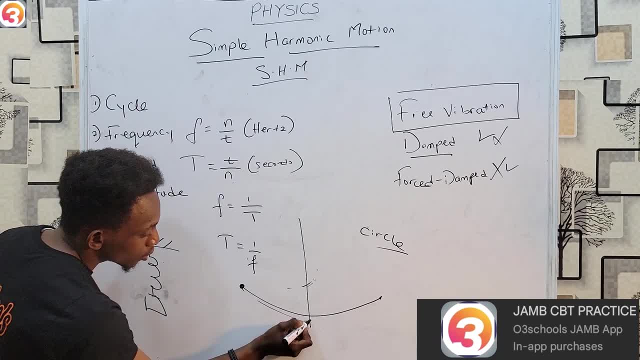 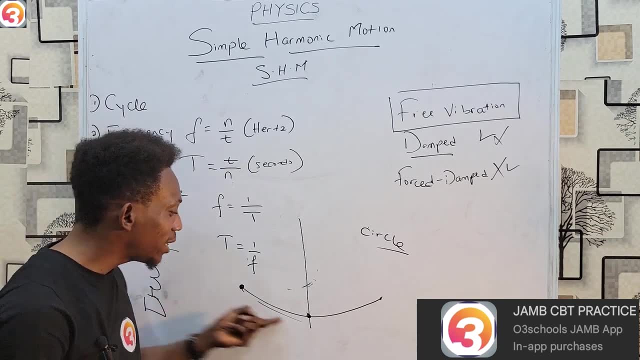 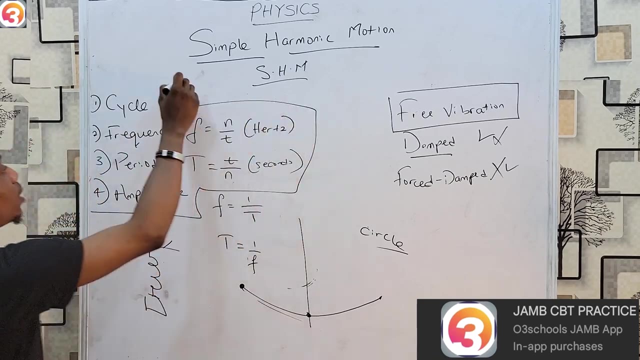 So the maximum displacement from the extreme to this middle gives us the amplitude. It's that simple. Amplitude is always the farthest it can go away from the equilibrium position. So these four key concepts. 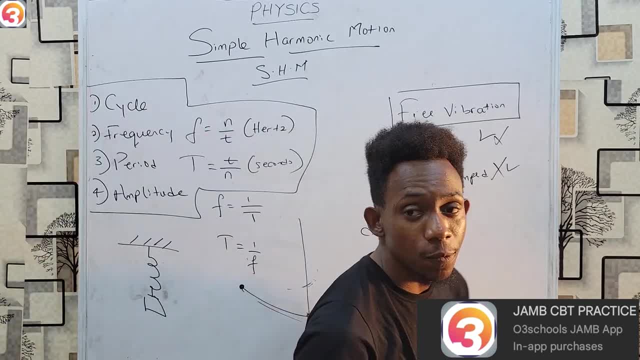 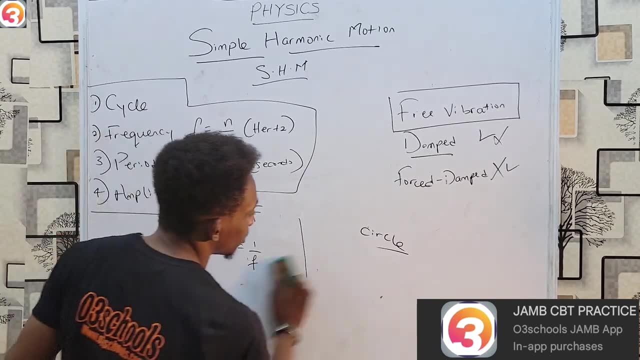 are the things we are going to be using a lot in this topic. And now, to start off, the first type of analysis we can, or we shall do, rather, is the analysis of circular motion. 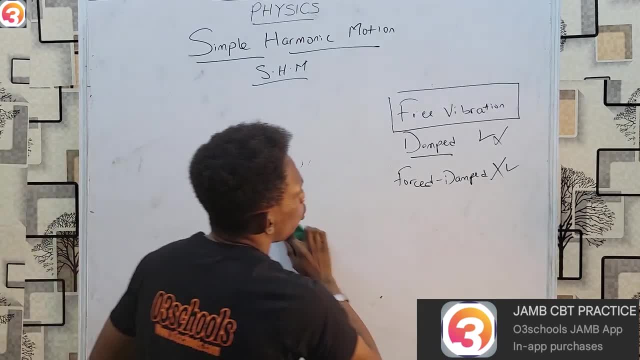 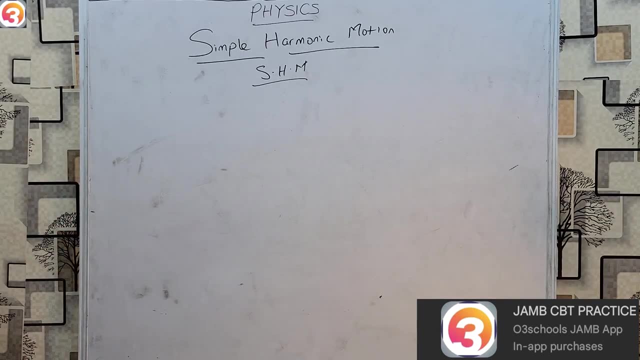 If an object is moving around in a circle, what is going on there? Because it's an easy way to analyze our cycle. Now, the first thing you should know is that when we are moving in a circle, 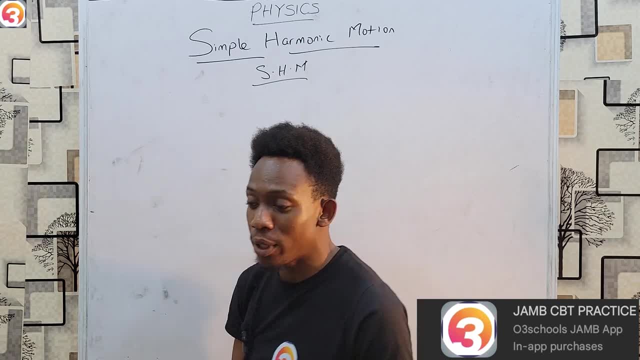 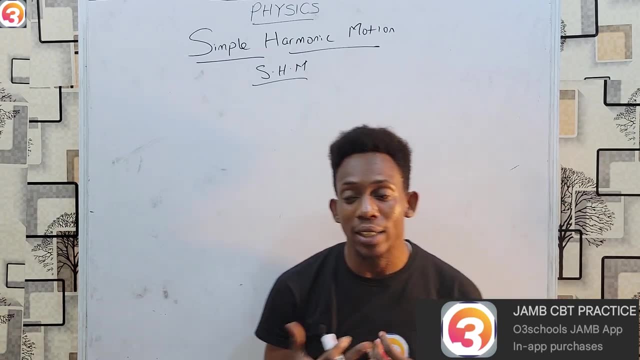 there are angular versions of our normal linear parameters. What do I mean? Normally, an object is moving in a straight line. it has velocity, it has displacement, it has time. Now, if I am moving in a cycle, 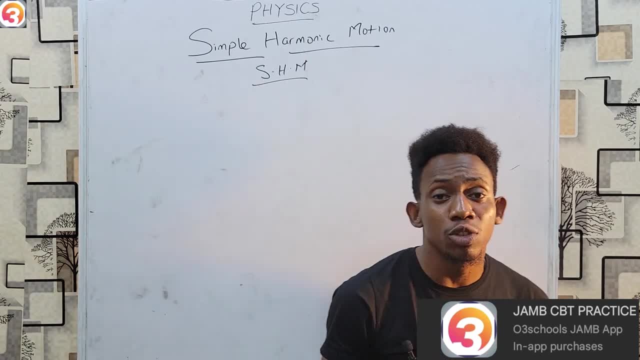 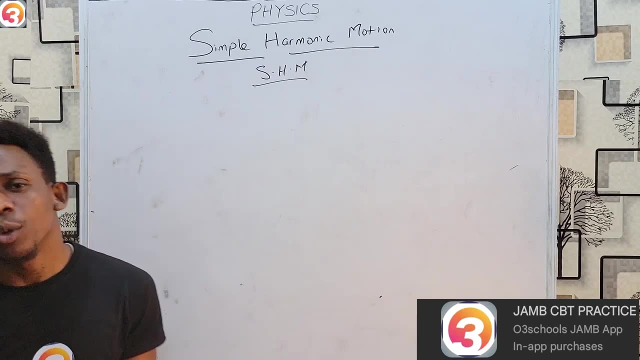 or in a circle, then I am going to now have an angular version of each of those movements. I will have angular velocity, then angular displacement is simply angle-tuned or at an angle. But time doesn't have anything to do with space. 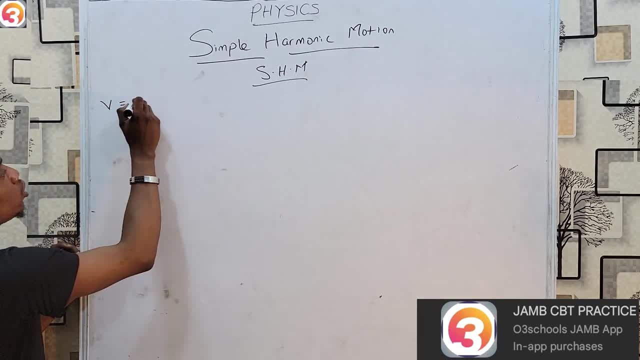 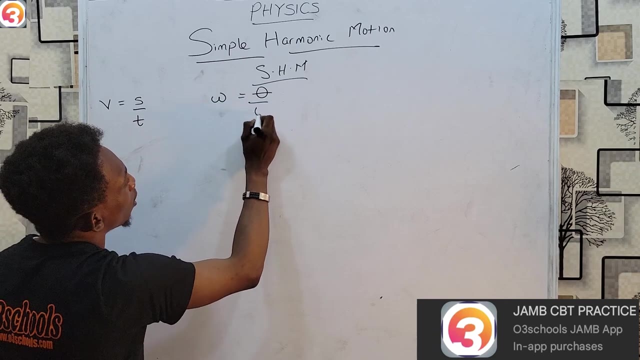 Time remains. time V equals to displacement over time. Then the angular version becomes angular velocity, represented by a simulator. omega equals to the angle-tuned, which is theta represented in displacement over. 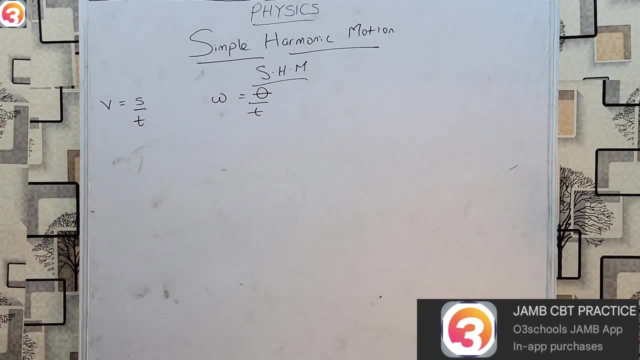 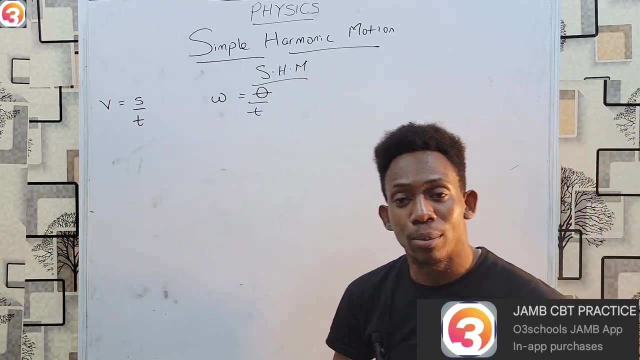 time. It's that simple. This is the formula for angular velocity. Now you may say: okay, after angular velocity, what's next? Let's do a bit of imagination and say so, assuming this body is completing one cycle. 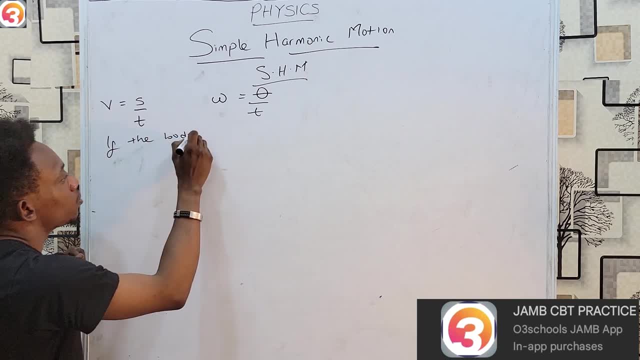 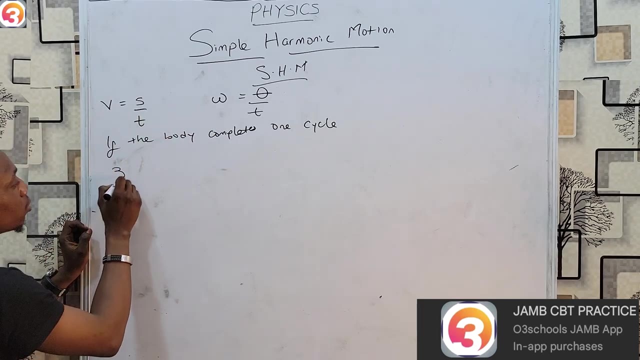 if the body completes one cycle. Now, before we look at one cycle, we should have to look at what makes a cycle a circle. A cycle is .360 degrees, But in this topic we prefer to use 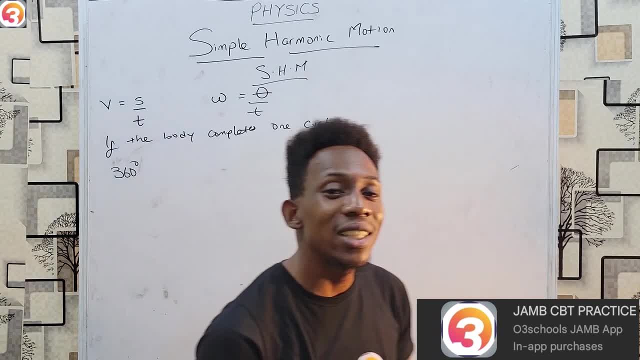 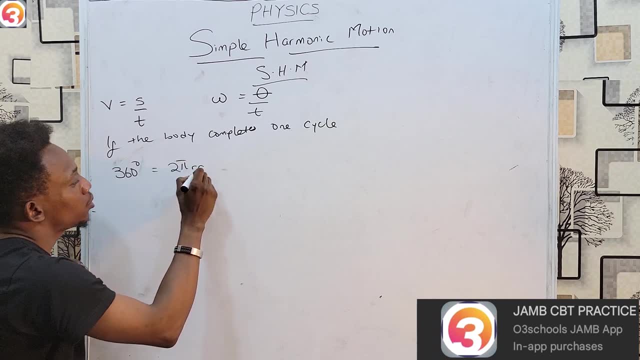 the SI unit of angle, which is not degrees but instead is radiant, probably called rad. So we should do that. 360 degrees equals to 2 pi radiance. So one cycle is one cycle is the same thing as saying: 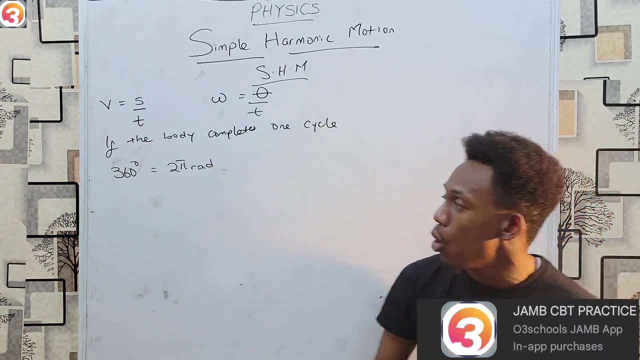 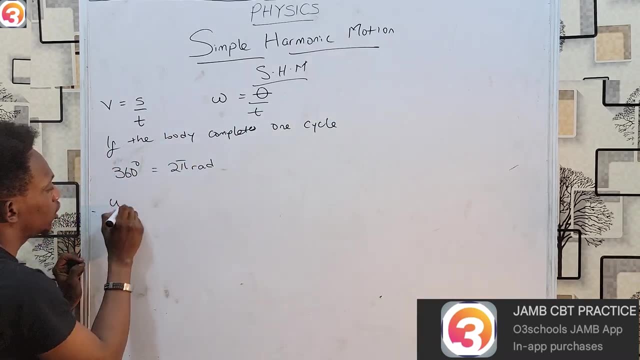 one revolution: .360 degrees, or .2 pi in radians, .2 pi rad. Therefore, I can say that my angular velocity will be equal to, like we said, it's completing one cycle. In one cycle, the angle is: 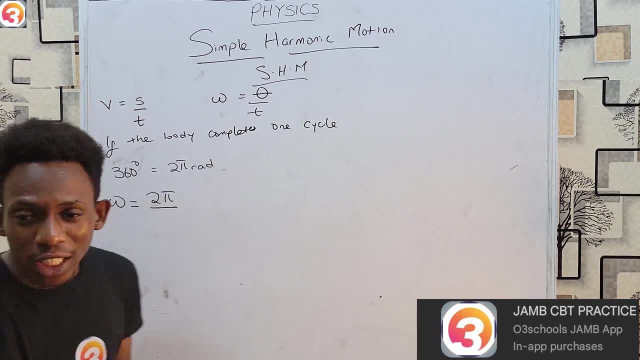 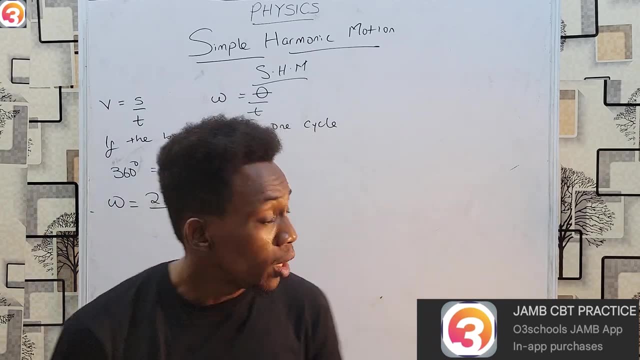 .2 pi in radian, And how long does it take you to complete one cycle? If you remember the parameters we just said, we said period is the time taken to complete one cycle And if one cycle is getting completed. 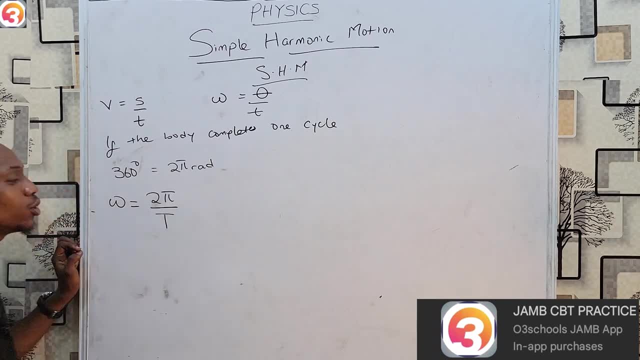 then my time must be equals to the period, And this gives us a very important formula that we shall use. However, after knowing this formula, is there something else I can do with the formula? Yes, I can remember that. 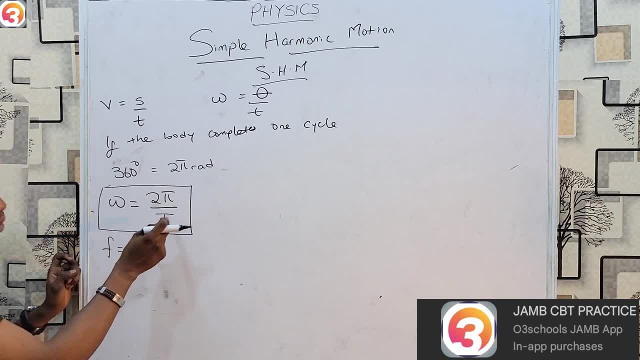 f equals 1. over t. And look at this formula. It's the same thing as saying: omega equals to 2 pi times 1 over t. Therefore I can replace 1 over t. 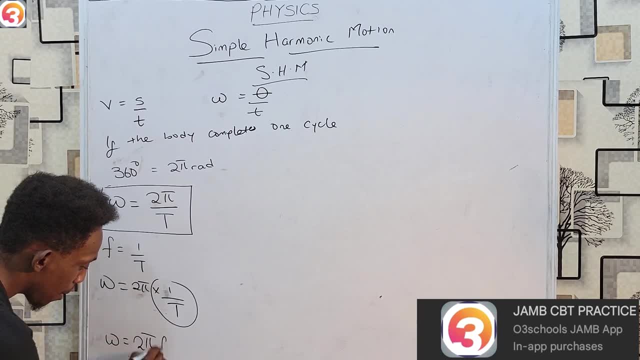 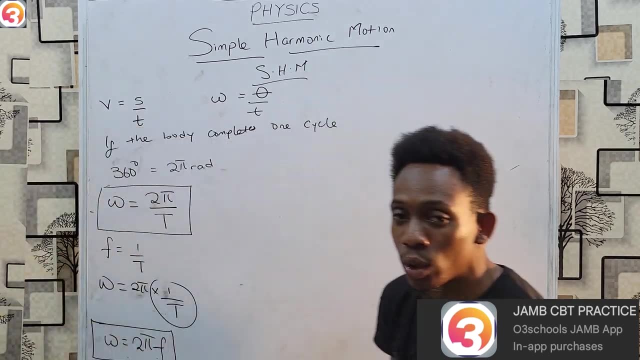 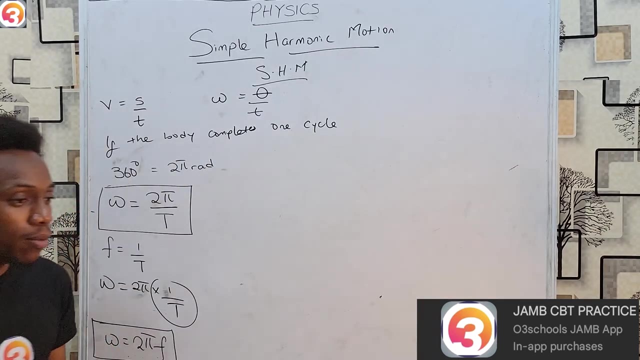 by saying: omega equals to 2 pi f. So you see, these are two of my formulas to solve for angular velocity. Now, with this in mind, the next thing we must remember is that what if we want to? 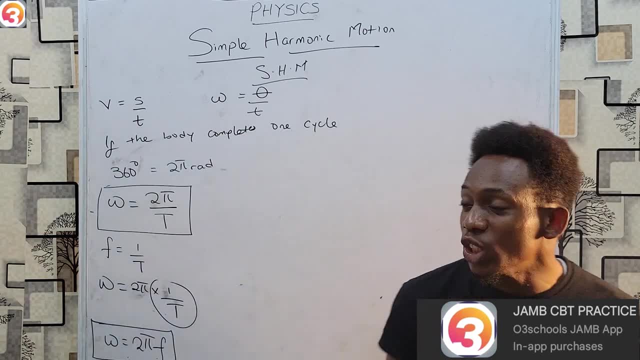 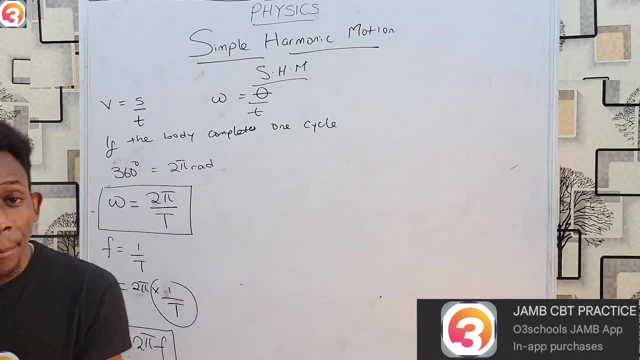 get the linear velocity parallel. for each of these I know angular velocity. What if I want to transfer this angular velocity from being angular into being purely linear? Then there's a general formula for it in SHM. 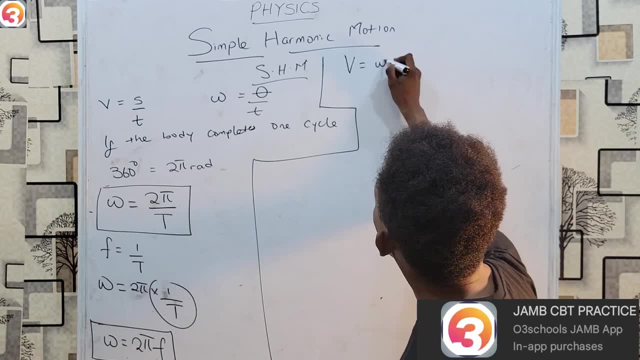 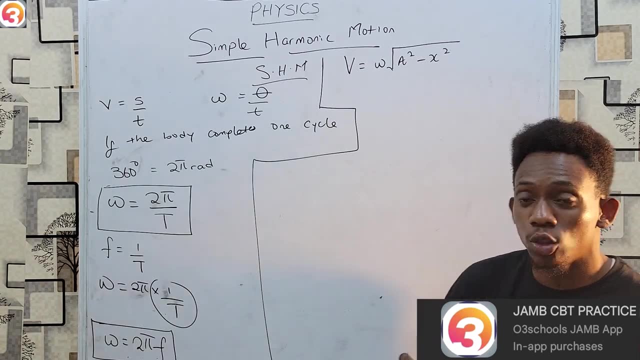 The general formula is that v equals to omega square root of a squared minus x squared. And now, before we get to parameters, try and just keep in mind: how do we get a and x? 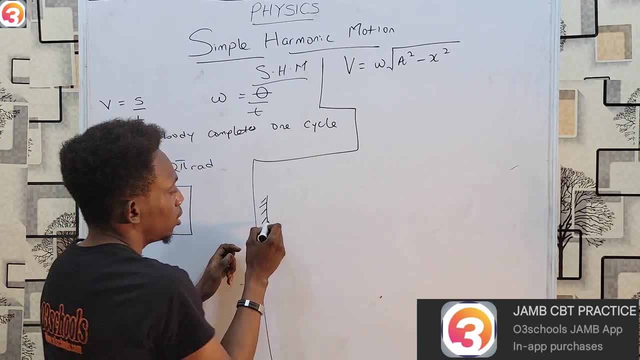 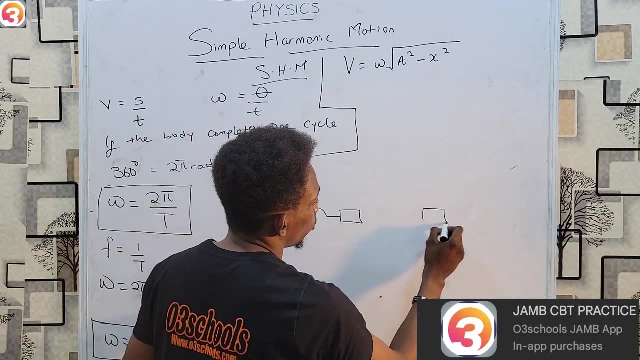 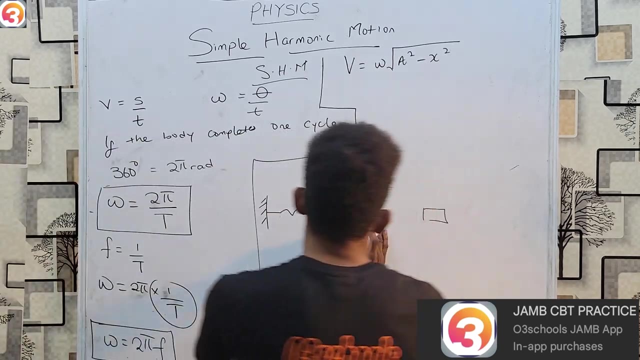 Let's assume I have a spring on this horizontal ground here and then there's a body here and let's call this place the maximum displacement. Therefore, remember for this spring to work. 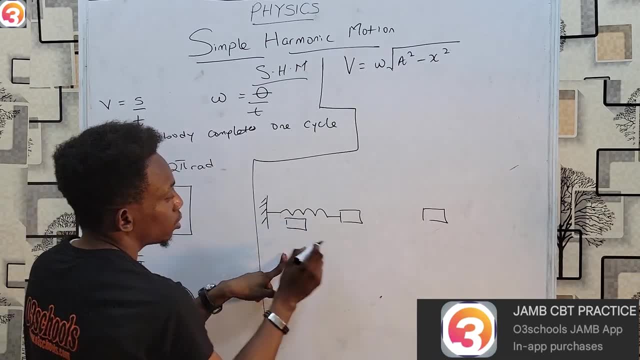 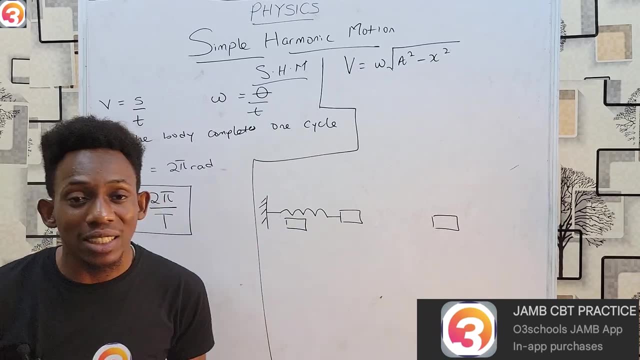 I must have compressed this spring to a certain point here, and then this is the maximum displacement, which means this middle where the spring wants to rest. it's my equilibrium position from here. 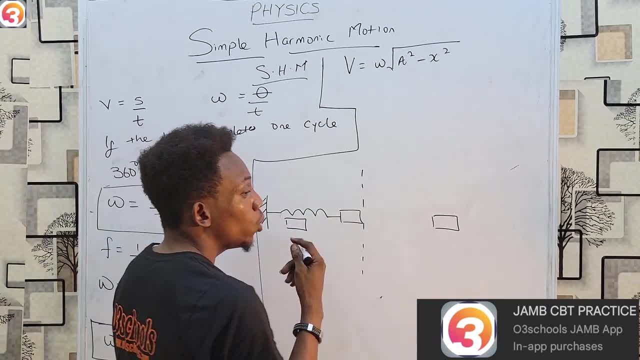 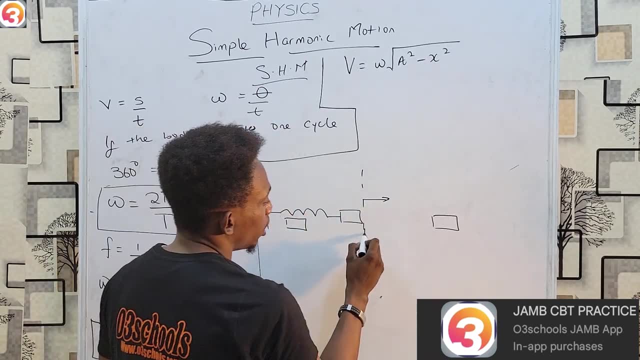 Now, how do we measure x? First of all, please note, we measure outwards from the equilibrium position. equilibrium From here we measure outwards. That means from here to here is my amplitude. 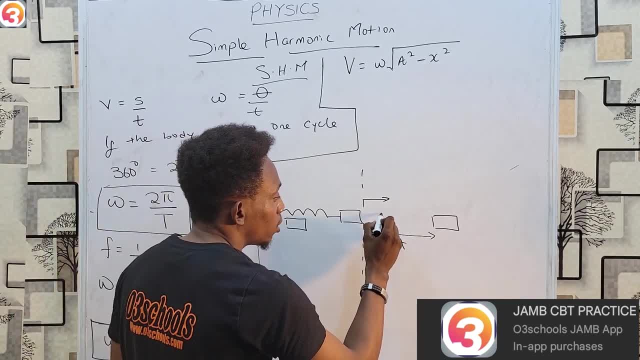 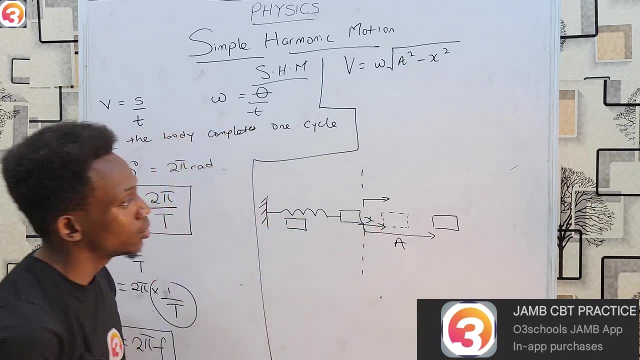 Well, what if it has not gone through the amplitude yet? What if it is somewhere here? Then in that case, from here to here is my x. So x represents the displacement from equilibrium position. how far you have moved from it? 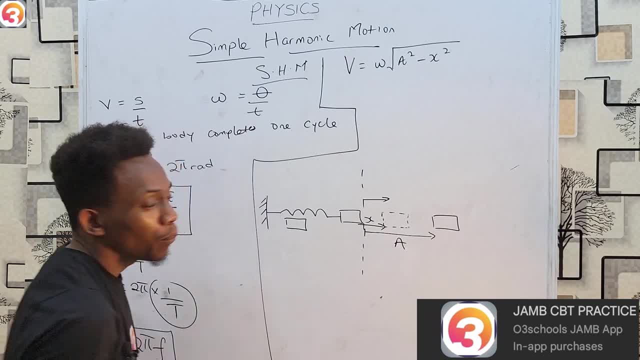 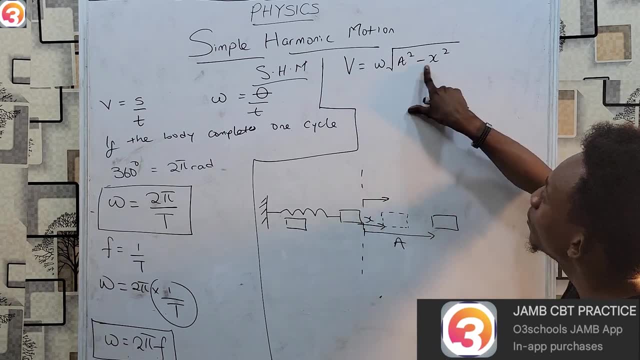 So here to here is my x, this is my amplitude. Therefore, the velocity v is simply equal to omega square root of amplitude squared minus x squared. Well, that means a couple things for me. 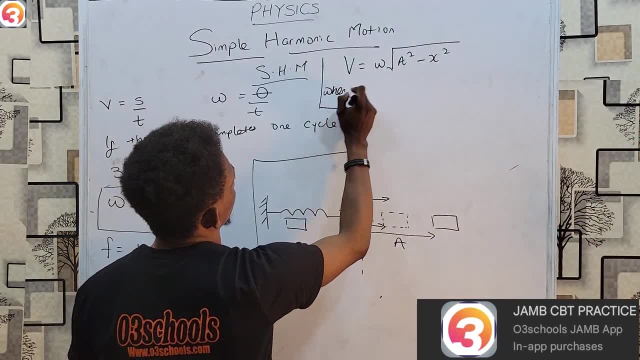 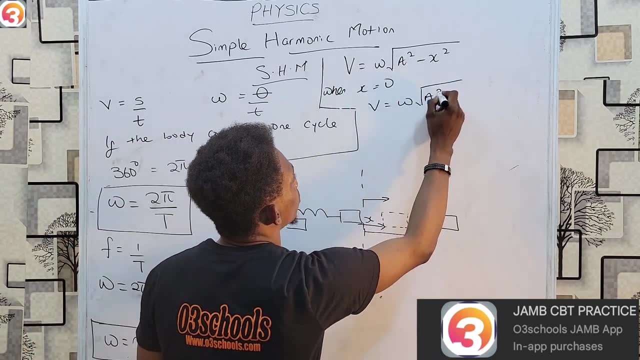 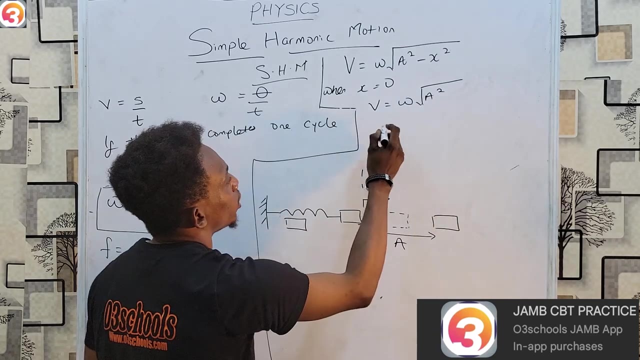 That means, when x is zero, when x equals to zero, then v must be omega, square root of a squared minus zero. squared Zero, squared is zero, obviously, and a squared minus zero must be a squared. 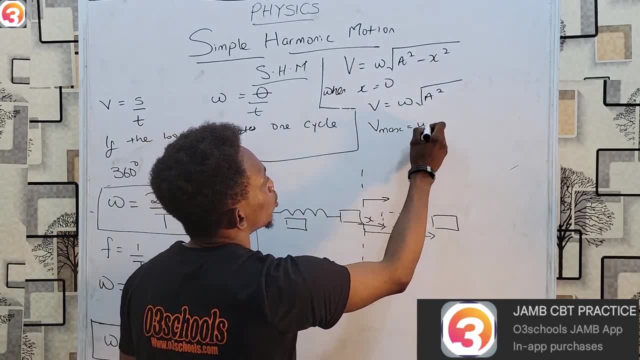 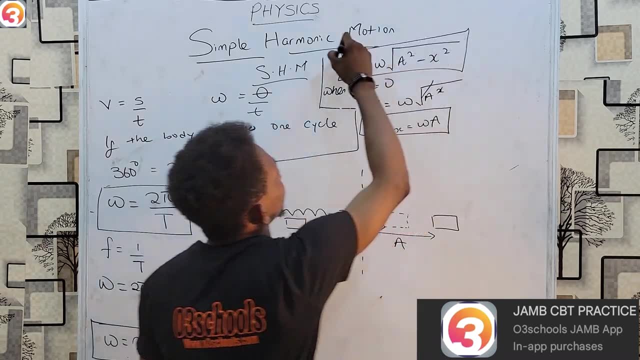 That means that the maximum velocity, v max, equals to omega square cancel square root of a. So this is the general formula for velocity, While the maximum velocity you can get in SHM is always. 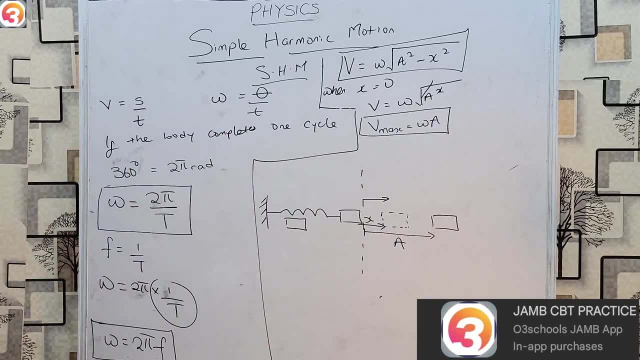 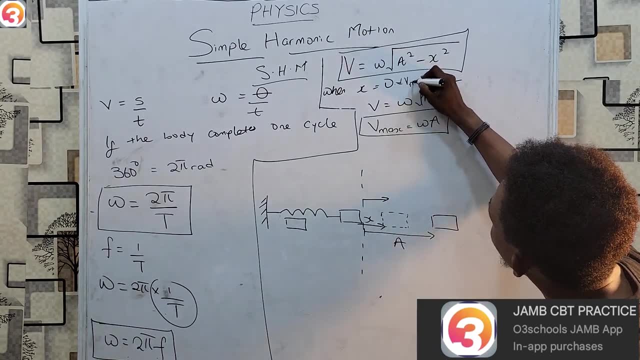 omega times a. That's very, very simple, Then. for the velocity to be minimum simply means- take note when x is maximum, when x is zero, rather v is maximum, but when x equals to. 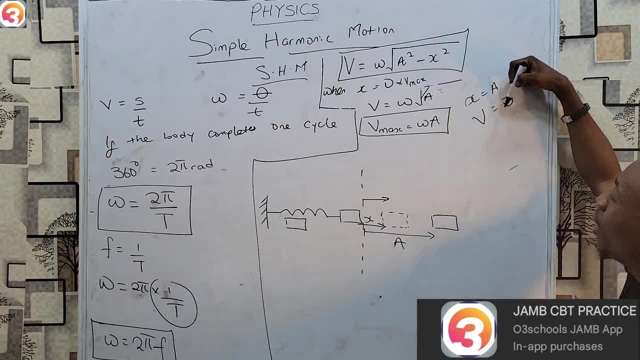 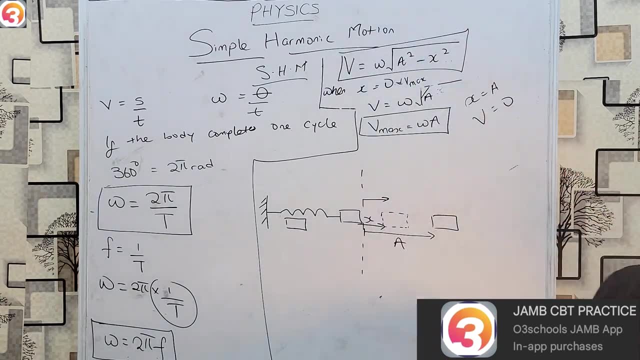 a, v becomes equals to zero, Because if x is a, that would be a squared minus a squared, which is zero. square root of zero is zero times omega is zero. So this is when it is minimum, when x is. 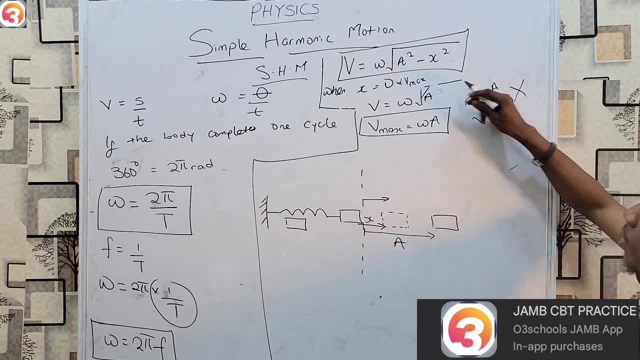 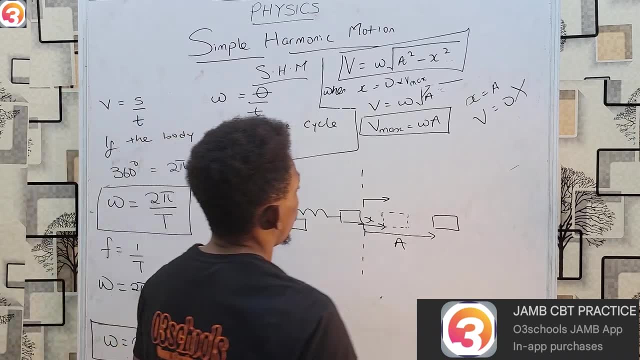 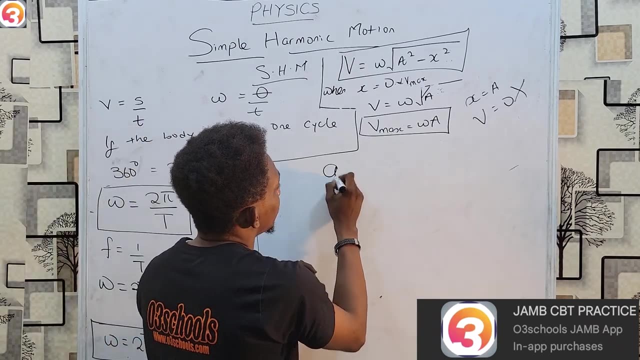 a and it is maximum when x equals zero. That's for velocity. What if I want to get the acceleration? Well then, for acceleration, all I simply need to remember is that the linear acceleration 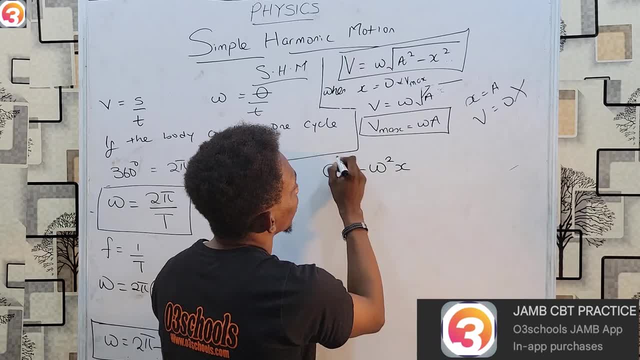 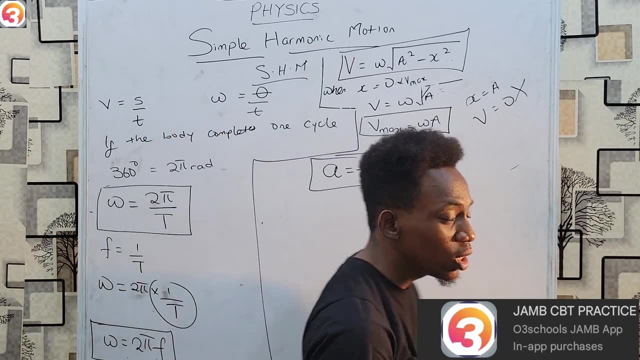 equals to minus omega squared x. Please just look In SHM. all we have mostly is a lot of formulas. The terminologies are few and far between. Just remember your formulas. So a equals to minus. 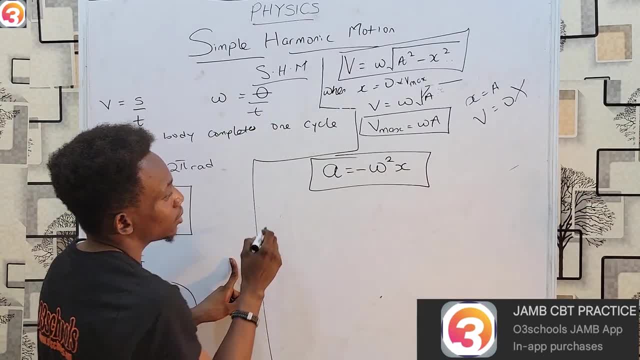 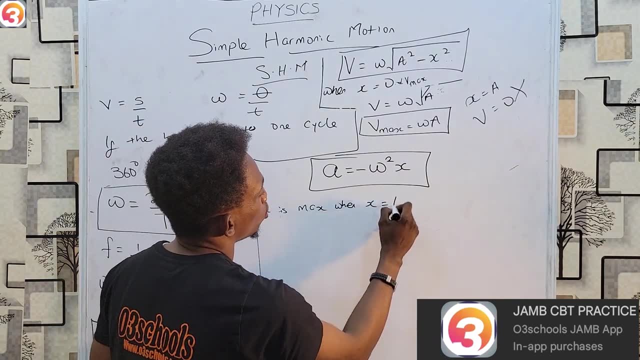 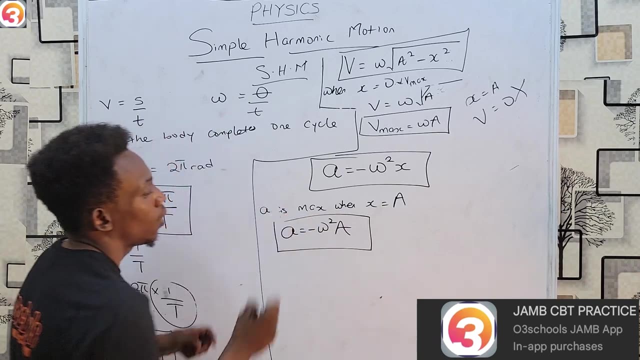 omega squared x, And for this one I would then notice that a is maximum. when x equals to amplitude, That means it will be equals to minus omega squared a. Then, obviously, if x becomes zero, 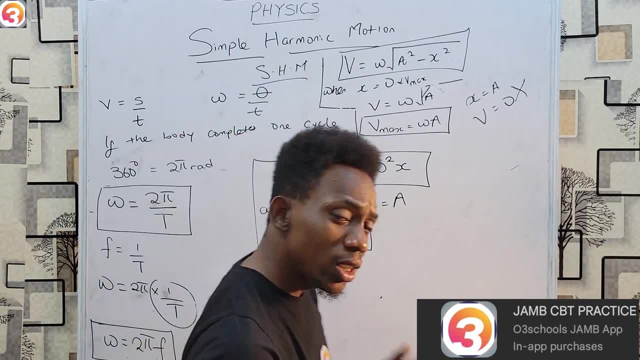 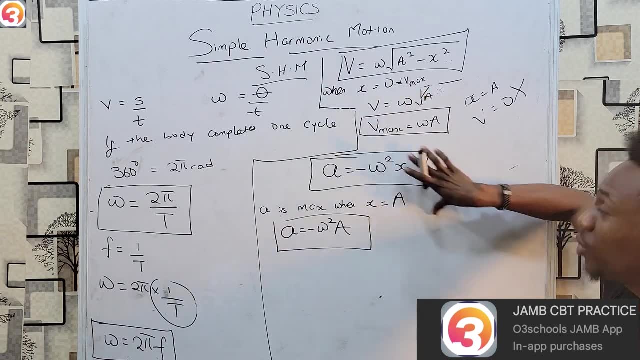 a becomes zero. So you notice velocity and acceleration are doing different things. When velocity is maximum, which is x, equals to zero, acceleration will be zero. So when velocity is minimum, which is zero, 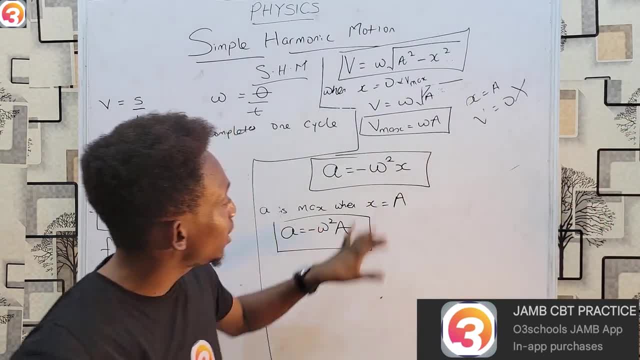 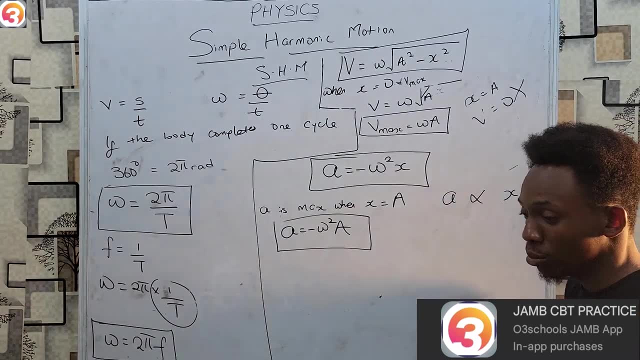 acceleration becomes maximum. And for those of you that may be asking how do we get this formula, It's because, as we said on the definition, acceleration is proportional to the displacement from the first point And it's always directed towards that point. 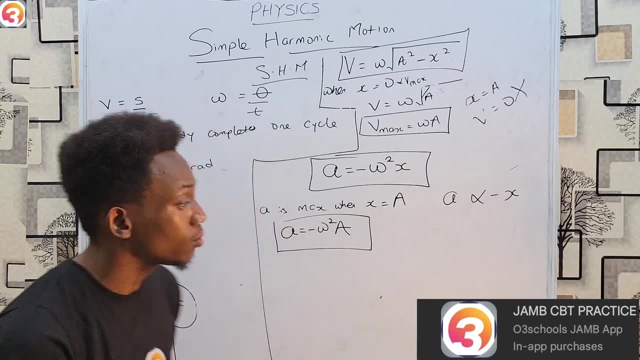 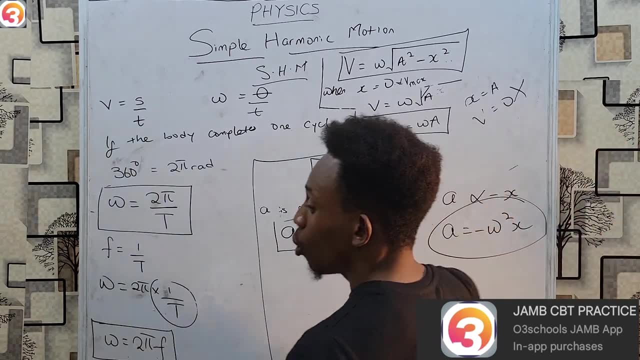 Plus, it's directed towards that point, Hence the minus. Then, from here, the constant was taken as minus omega squared, And that's how we got that Very, very, very simple. So these are the few formulas you must know. 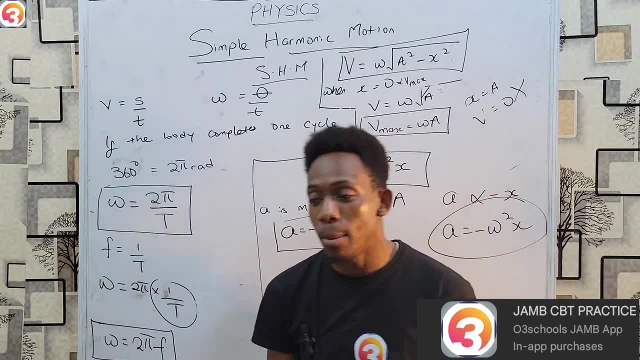 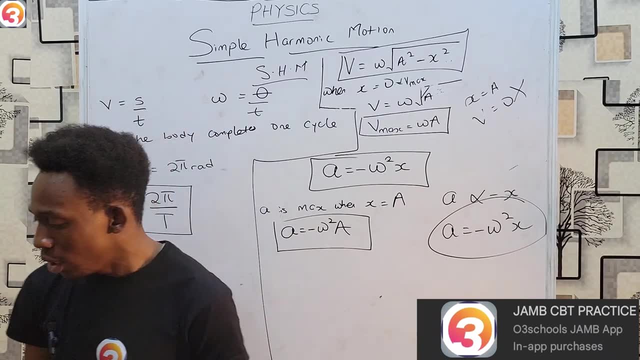 first off, generally for any simple harmonic motion problem You might have the question: you must know this problem. But now there are now some specific problems that can come up. The first one has to do with: 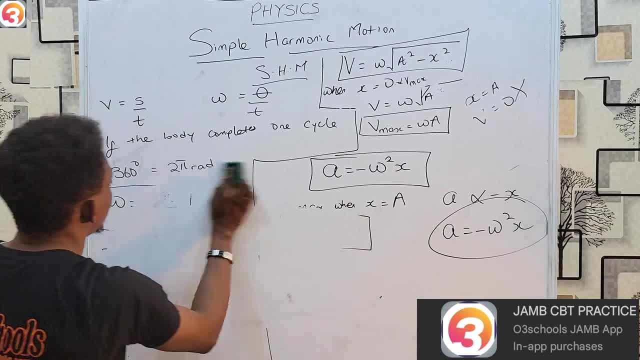 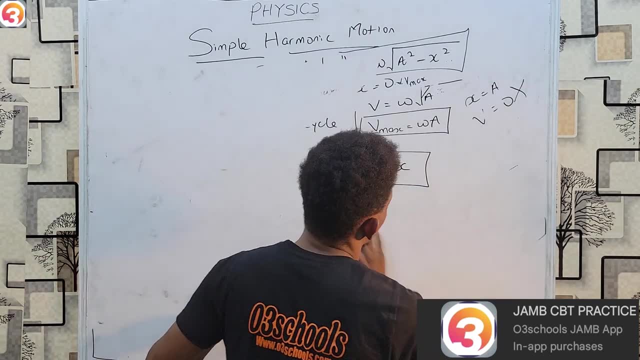 something we've been mentioning over and over again, which is the simple pendulum. Now, in the simple pendulum, there's a special problem that can come up, And that is what if you have a pendulum? 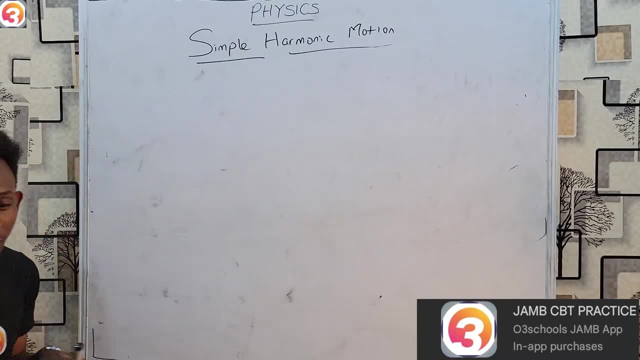 you know the length and you want to swing it. How many times or how long should it be swinging? What affects how long it takes to swing? What you should know is that the period in simple harmonic motion for a pendulum. 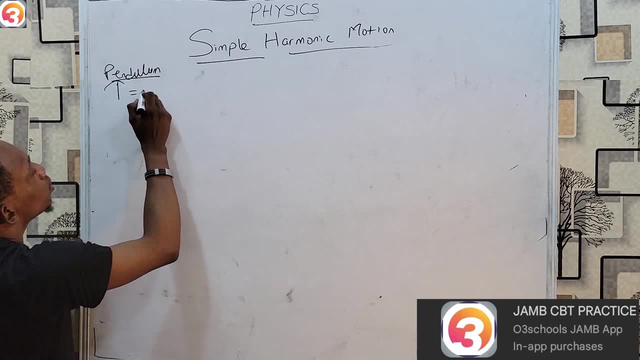 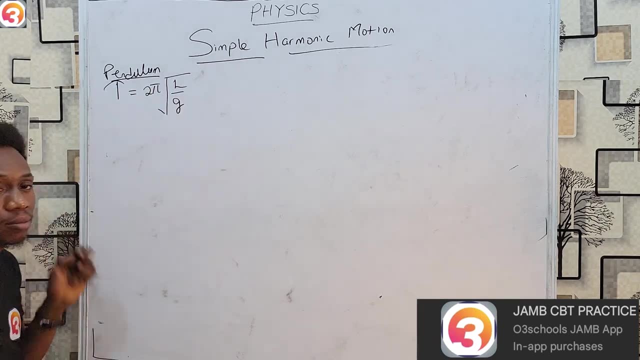 let's notate, for a pendulum period equals to 2 pi square root of L g. Please take note. This is your simple formula affecting the period and the length. 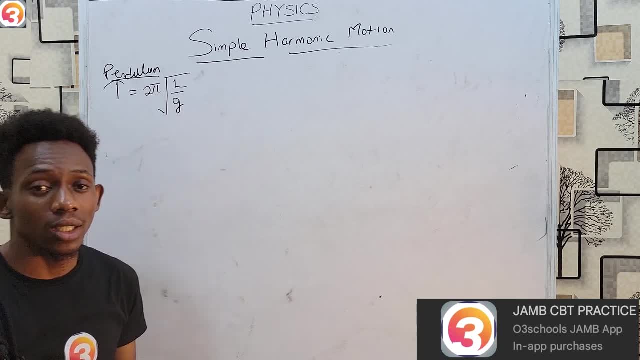 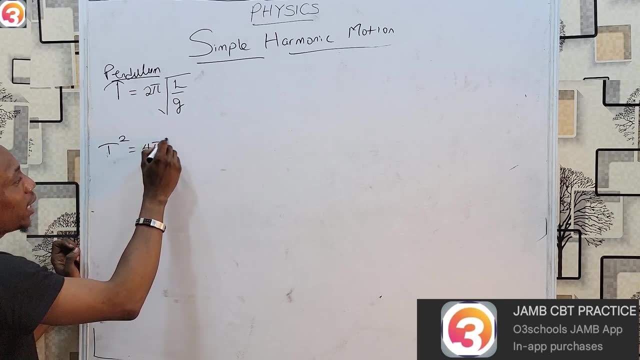 Now this g is supposed to be constant, indicating that because this formula is simply gotten from by saying c squared equals to .4 pi squared L over g. This is from experiments which simply know that these two are what vary. 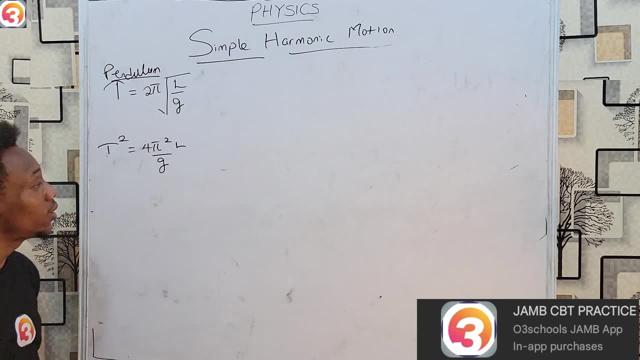 because in a certain location g is constant. The one found square root of both sides it got this. So please take note: As long as g is constant, then the period varies with the length. 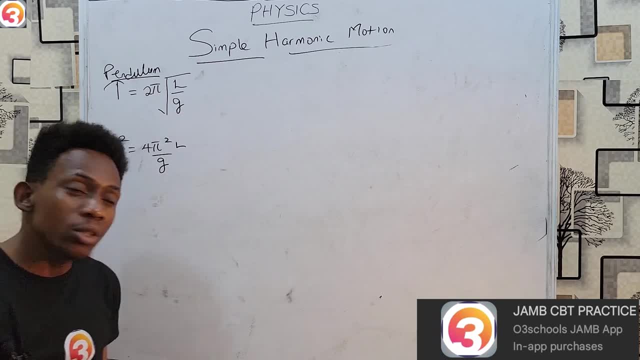 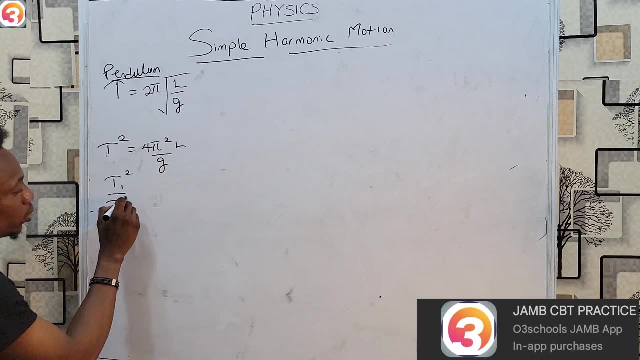 not just the period, the period squared. So in a question, if you are comparing just period and length, the formula is going to be: t1 squared over t2 squared equals to L1.. 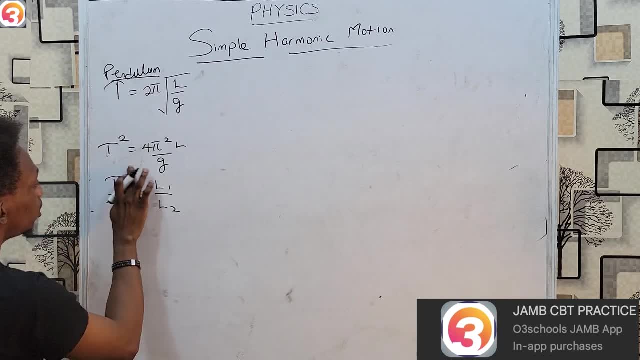 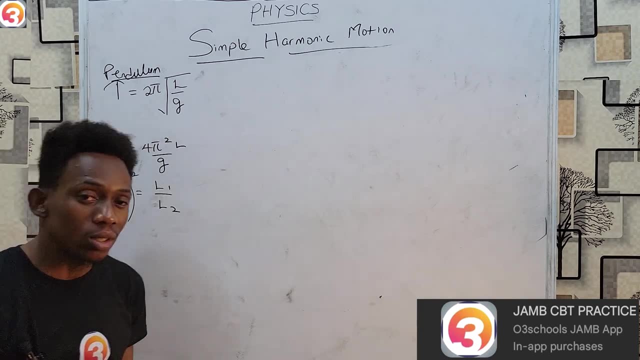 over L2.. But, if you like, in some cases put the square in the brackets. t1 over t2 squared equals to L1 over L2.. Either one works, So it's only if you are comparing two. 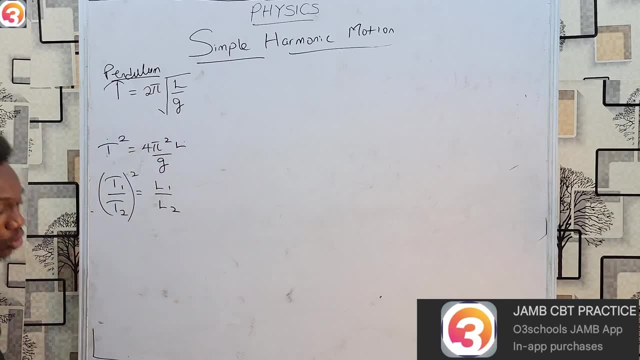 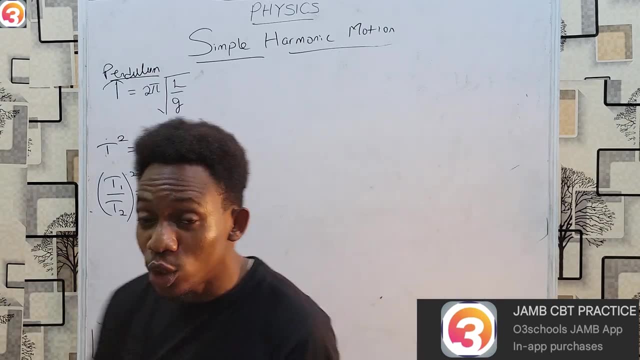 If you are comparing in a particular location, period and length, Because in some questions they will tell you the length is increased or the length is shortened, and so on and so forth. That becomes your easy, simple formula Now. 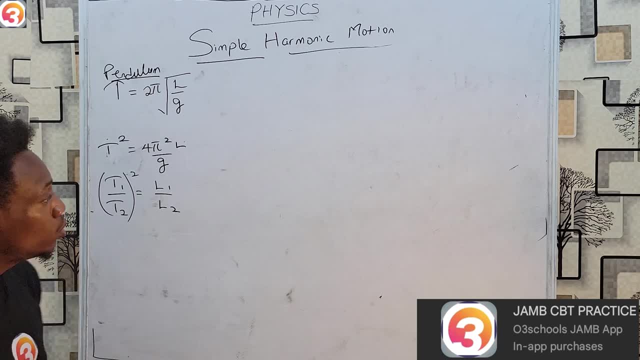 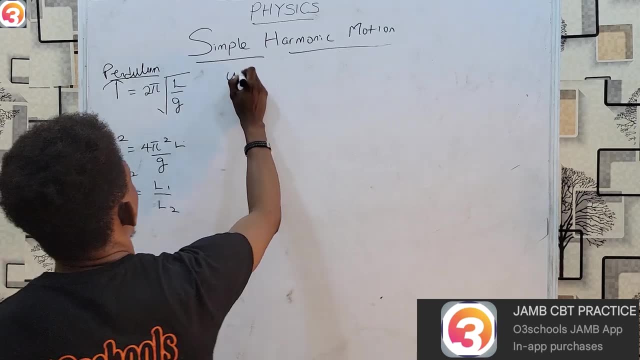 once I have this established for this particular scenario, one more thing must come to mind. I have this right now, But I should remember that angular velocity equals to 2 pi over period And that, if I rewrite this, 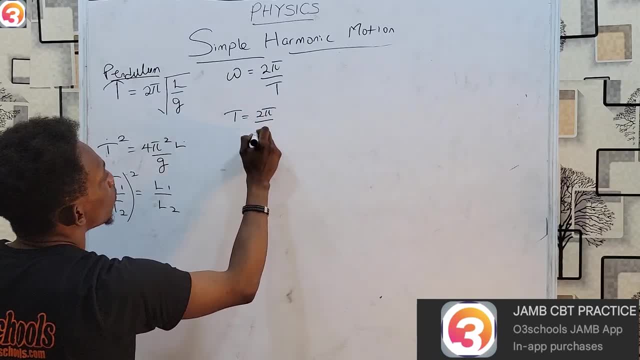 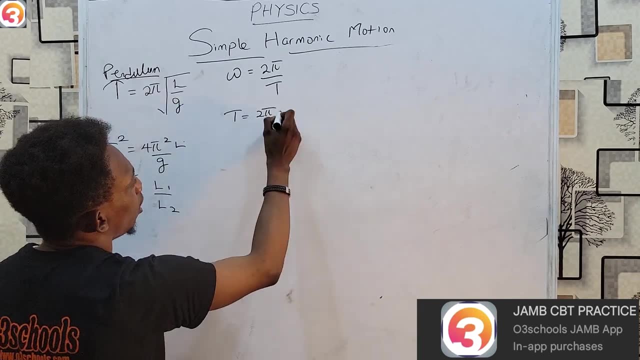 it seems to have told me that c equals to 2 pi over angular velocity. Now, this and this seem to look alike Because, for example, this is the same thing as saying times 1 over angular velocity. 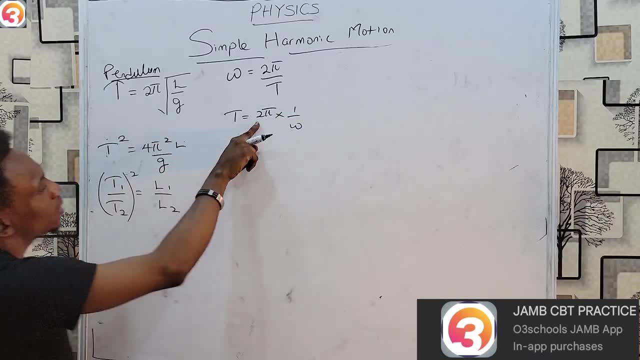 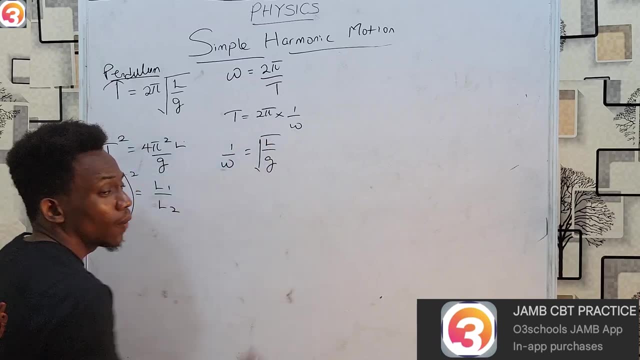 c is t, 2, pi is 2 pi. I'm left with the fact that omega equals square root of l over g. What this simply means is that I'm now able to get my angular velocities by saying: 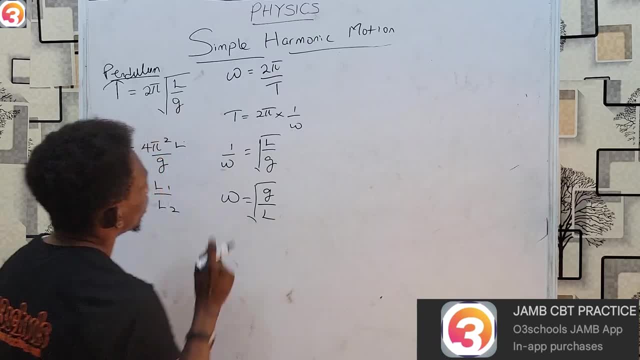 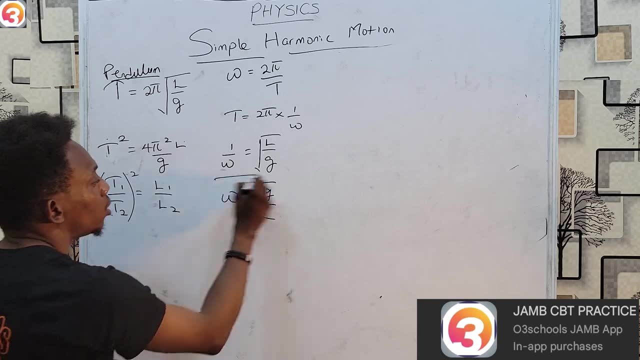 square root of g over l. Now I know some of you may be looking at this and saying the formulas are too many. Well, please note the formulas you need to remember here are this this: 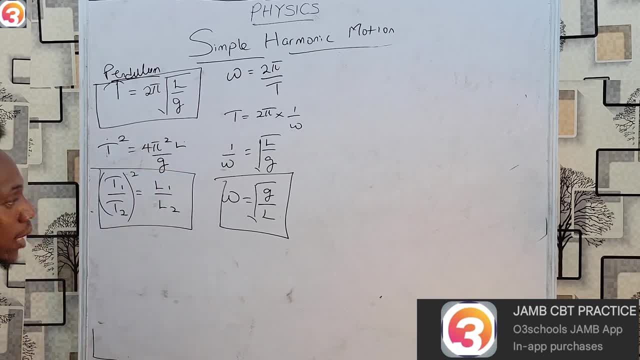 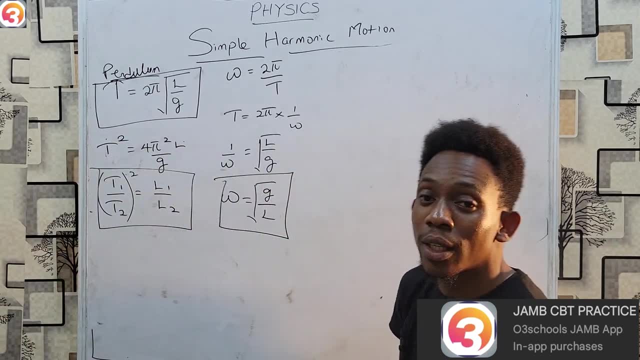 and this. Those are the key formulas. Some of them are simply just proofs to tell you how we are going from one to the other. Like I said, there are two things. we are looking at Two special scenarios. 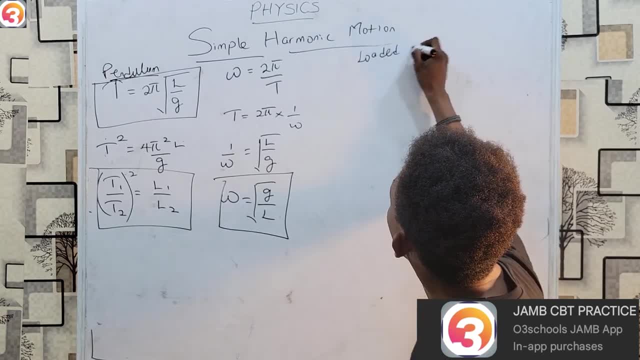 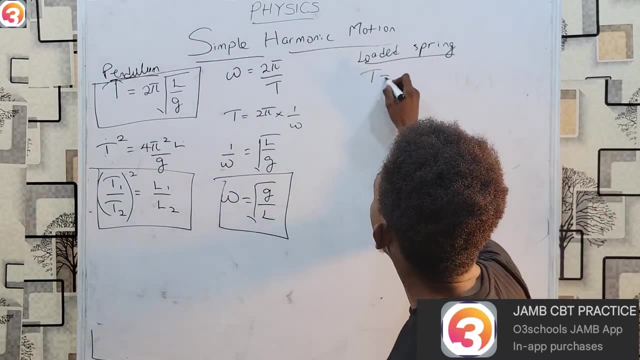 One is the pendulum. The second one is the loaded spring, And your spring behaves just like a pendulum, but in its case the formula becomes: c equals to 2 pi square root of m over. 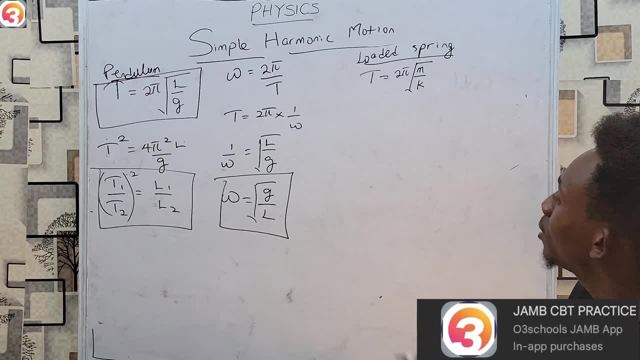 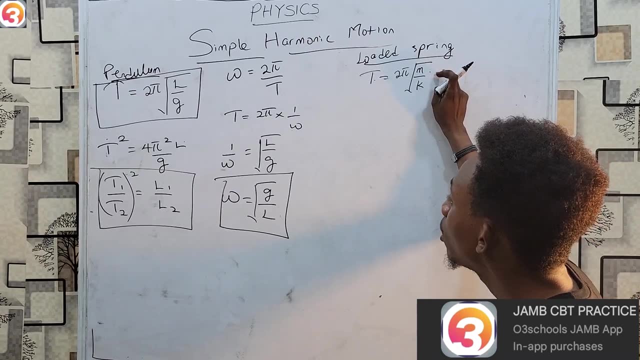 k. That's it, And in this case, that simply tells you that your period depends on the mass. Depending on the mass, your period depends on that as long as you are using a particular spring. 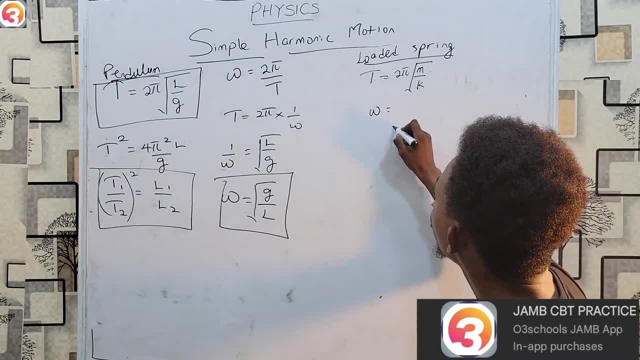 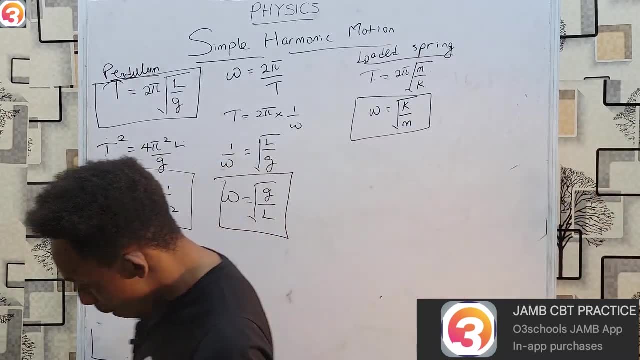 And therefore, just like this, omega will be equal to the square root of k over m. So these are basically some of the things you should be looking at in this topic. There is one last thing. 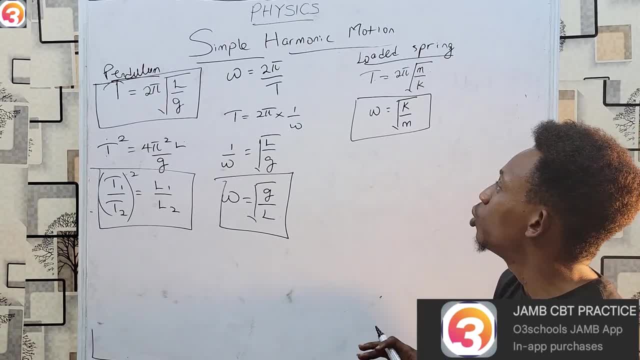 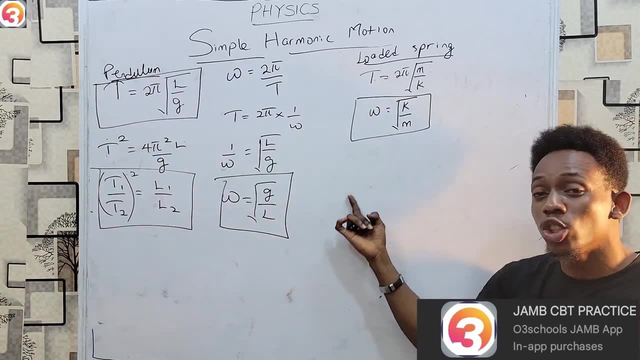 it's a very conflicting jump, but you should know one more thing about harmonic motion, which is the energy. Energy, as you are aware, is getting transformed from potential to kinetic energy. Please note the maximum energy. 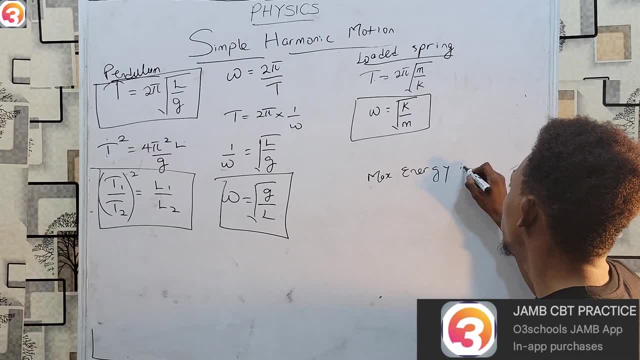 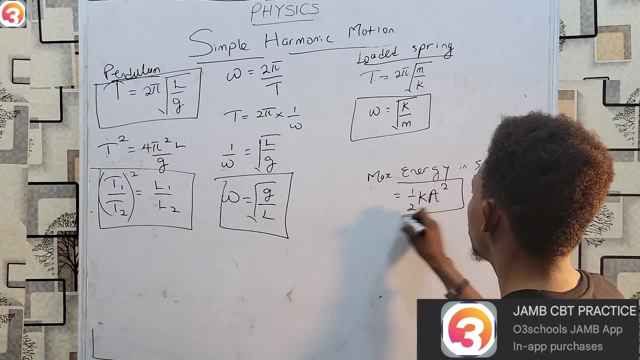 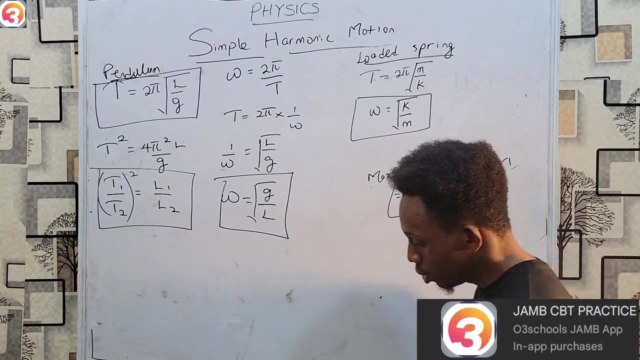 in your system, energy in SHM is equal to 1 over 2.. k a squared. This k, like the k here, is first constant, while a is your amplitude, And I'd like to assume that all these symbols here 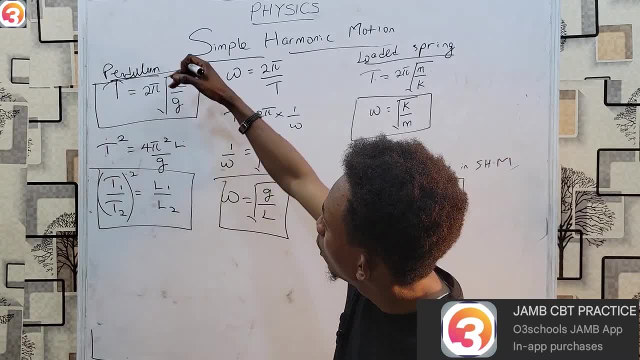 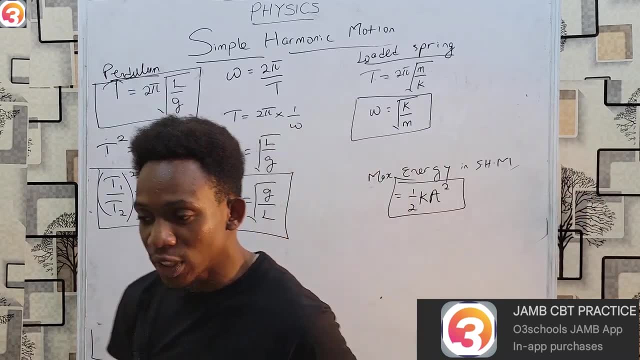 are all familiar, We've seen them before: t is period, l is length, g is acceleration due to gravity and omega is angular velocity, like we know. Now, the last thing, the last key, we should know. 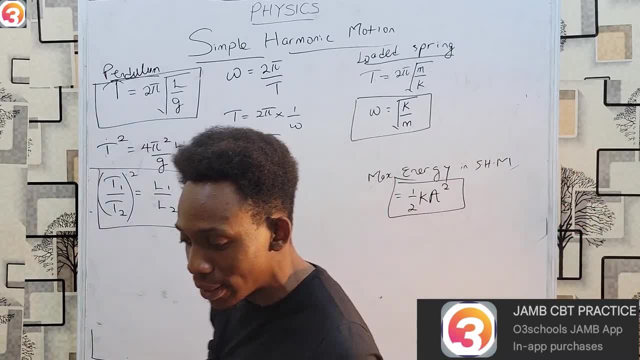 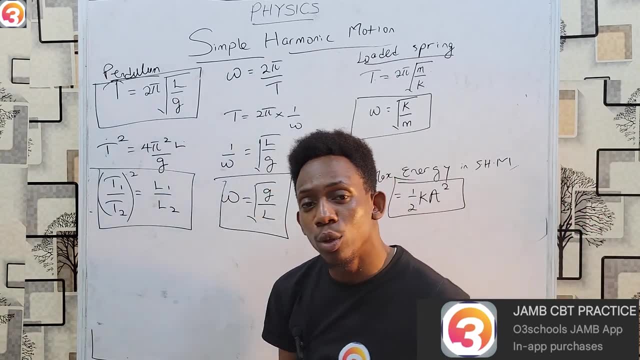 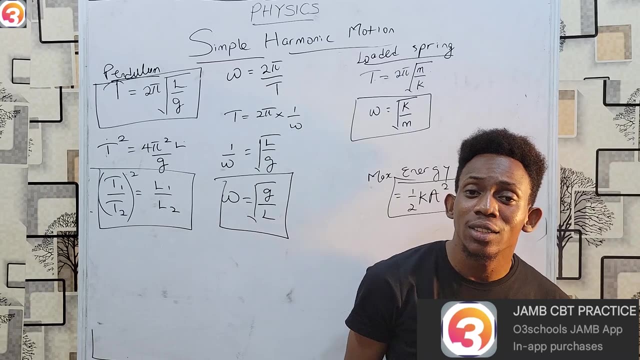 is something known as resonance. What is resonance? Resonance simply occurs when a body vibrating at a frequency forces another body into vibration at its own natural frequency. How does this work? Every single object in the universe. 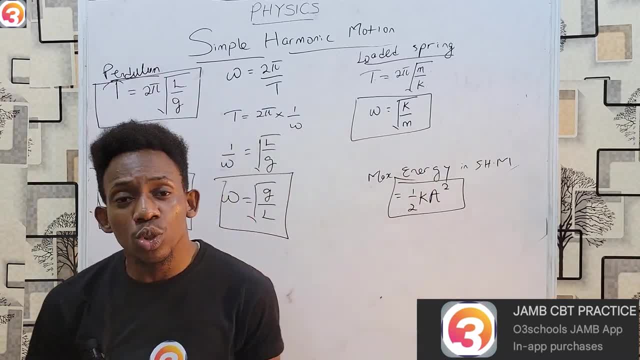 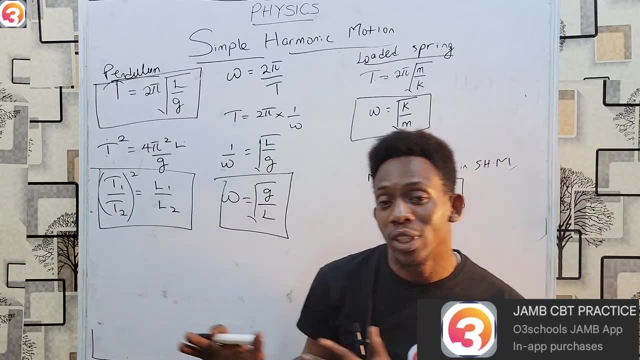 has a natural frequency. That means, if we are exposed to frequency of that exact value, we too will get set into oscillation once we experience that frequency. But what causes it? Something else has to move at that frequency. 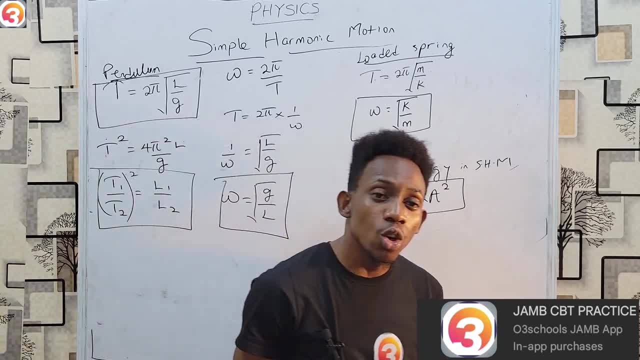 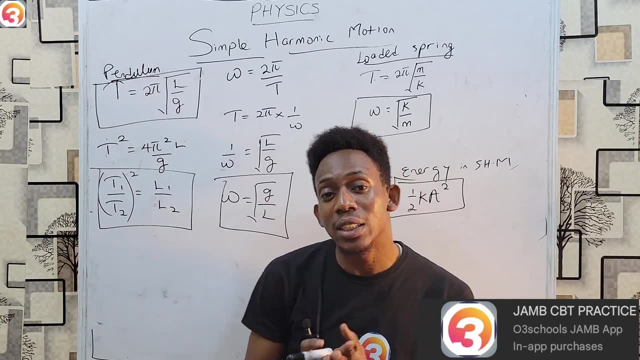 for us to feel that frequency. So resonance occurs when another object is moving at the natural frequency of yet another object and ends up setting that object into vibration as well. A good example is one we see at times. 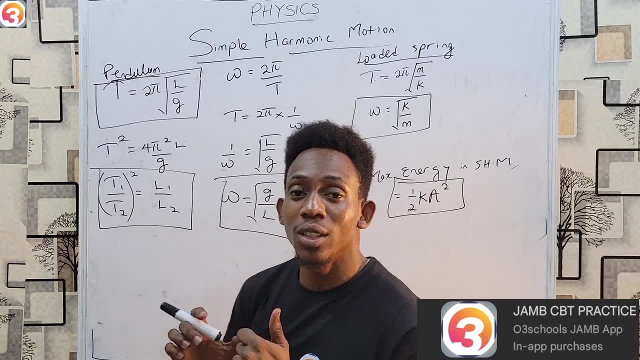 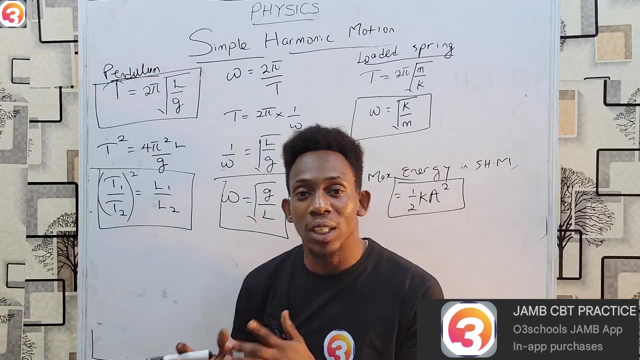 of videos of opera singers breaking glass with their voice. What they are simply doing is matching the frequency of the sound they are producing to the frequency of the glass. When both match, they set the glass to vibration. 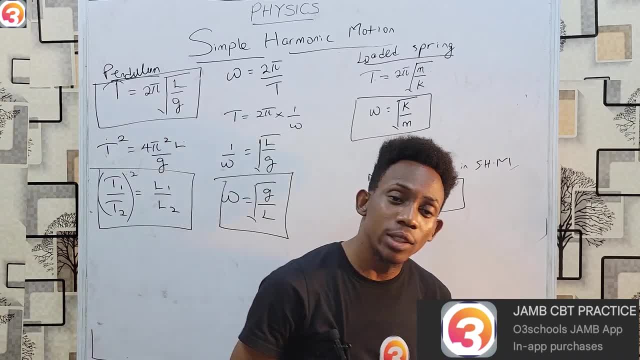 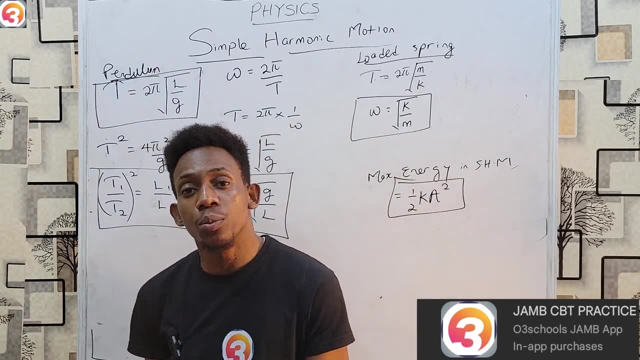 which breaks it, And we will jump back to ask this question. at times It is either in the form of a diagram or in the form of a question, where they tell you that the glass matching on the bridge 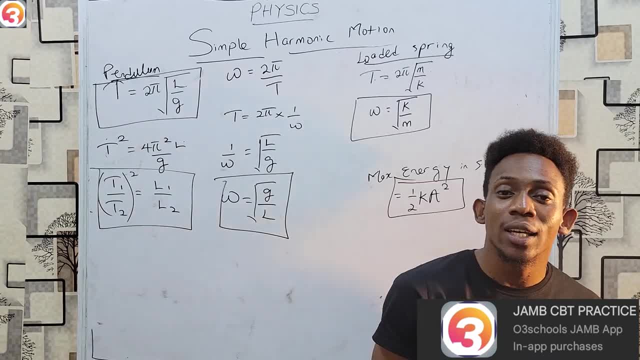 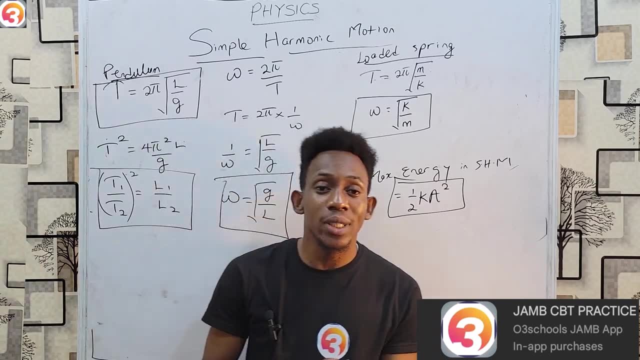 are advised to break their steps because it is simply so that they can avoid mystically getting to the resonance frequency of that bridge. If both the glass are matching uniformly across the bridge, then there is every possibility that they might. 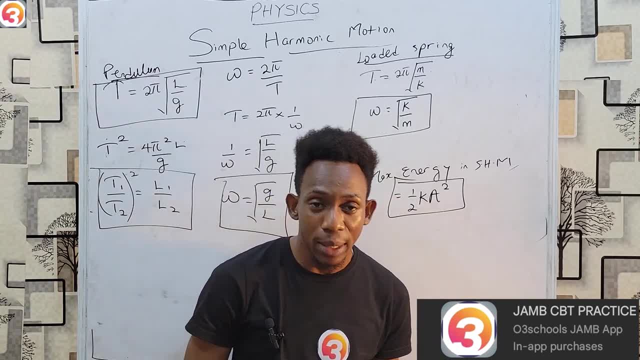 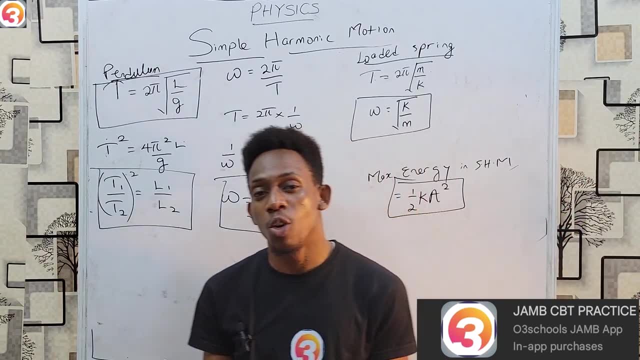 just reach the resonance frequency of that bridge and they end up collapsing the bridge and themselves with it. So instead they are advised to break their steps, so that as one is going down, one is going down, one is going up. 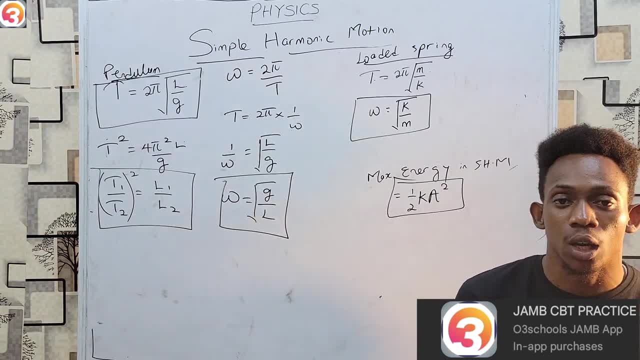 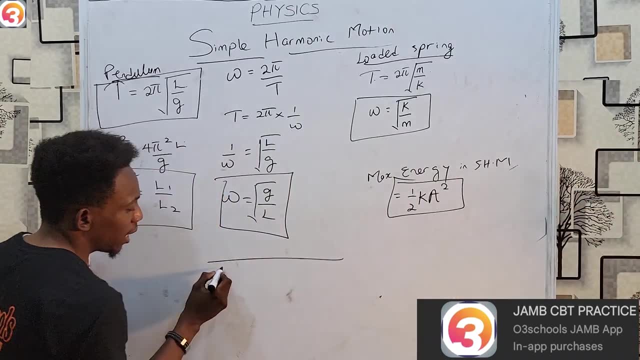 so the frequency will never ever break the frequency of the bridge. Now I said there are two ways, that is, the theoretical way and the diagram way is the most simple. It can simply be a diagram with several objects. 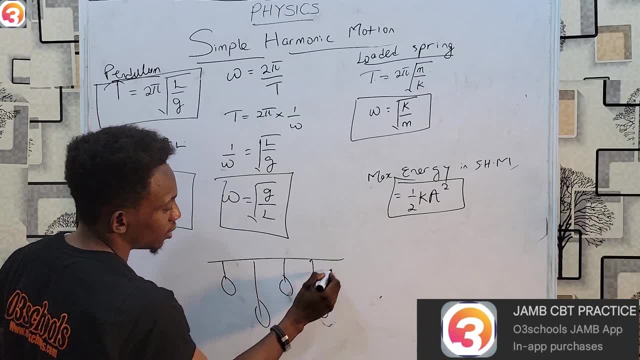 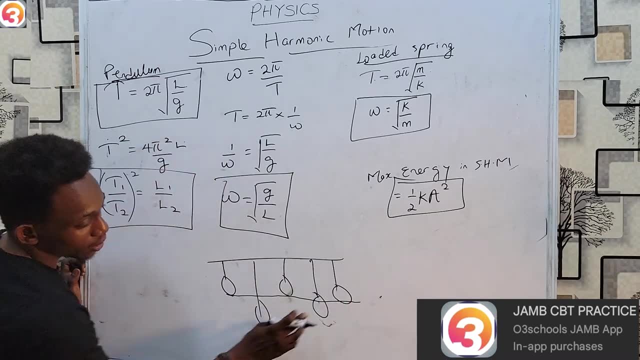 and tell you which of them can set anodine to vibration. It simply does of equal lengths, Like in this case. now, if these two are the ones that are equal, then these two can set each other into. 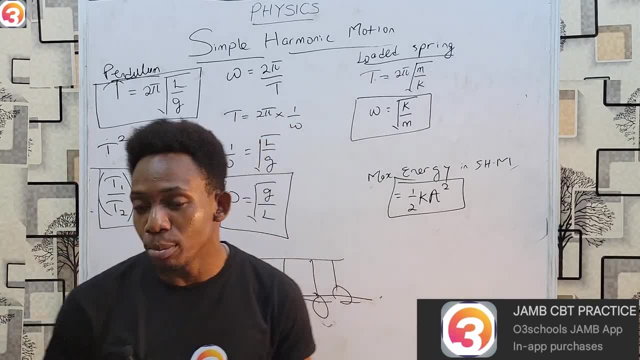 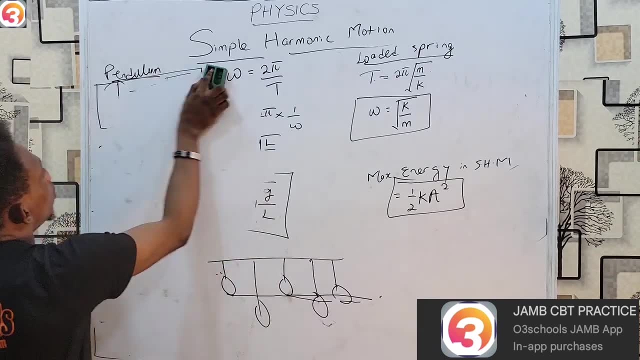 resonance. The others can't because they do not match. So with these, I believe it is time for us to do what we always do, which is we are going to open our Old Three Schools Jam app. 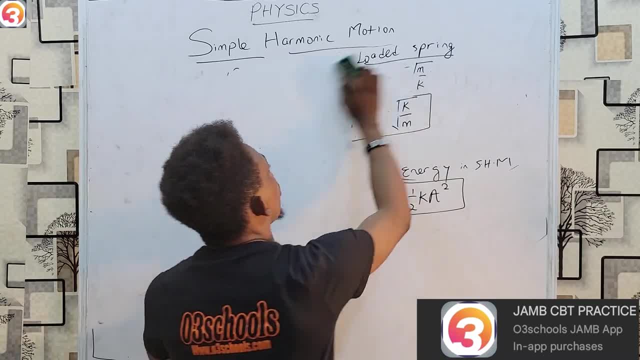 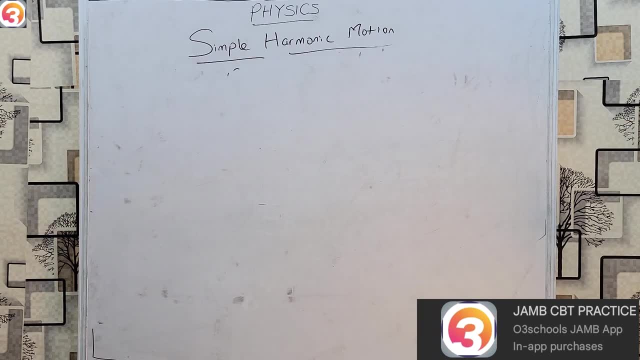 and apply all these formulas and knowledge we have gained towards solving past UTME questions. So just to get my phone here and open my Old Three Schools Jam app and our very first question. 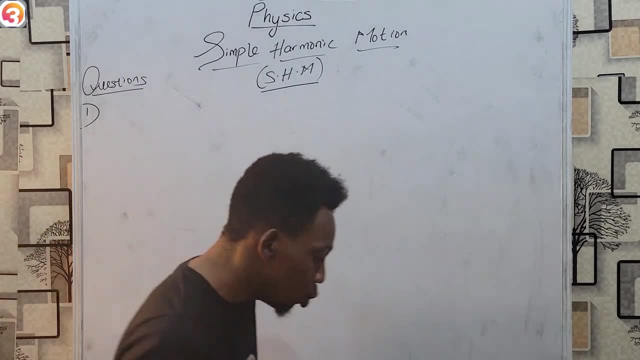 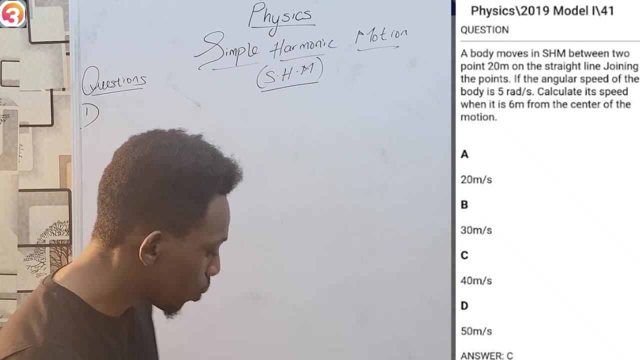 comes from the .2019 Model 1.. question 41. on our Old Three Schools Jam app, The year is 2019.. Model 1.. question 41. A body moves in simple harmonic motion. 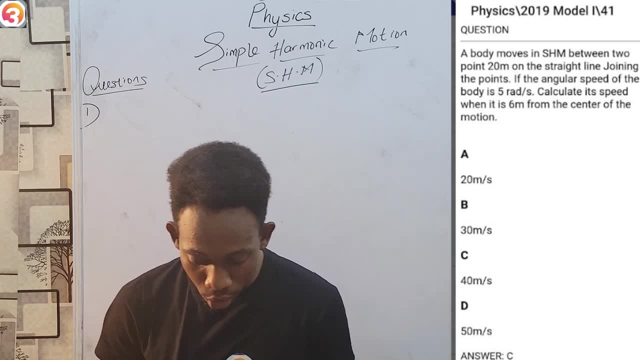 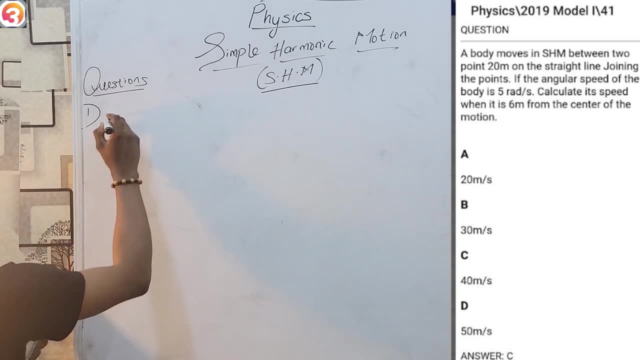 between two points: .20 meters on the straight line joining the points. If the angular speed of the body is .5 rad per second, that's 5 radians per second, we have to calculate its speed. 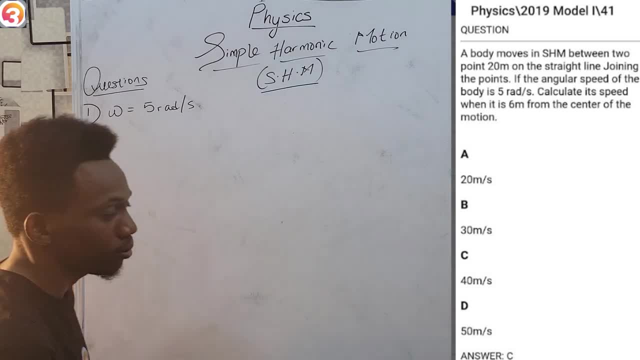 when it is 6 meters from the center of motion. Now here are features we have to figure out here Right now. I know that this is one equilibrium point, or one point, and the distance from here to here. 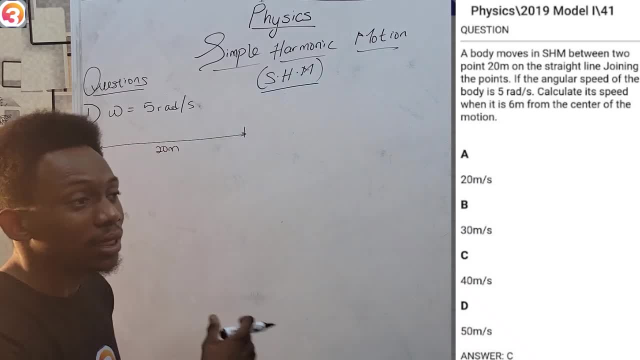 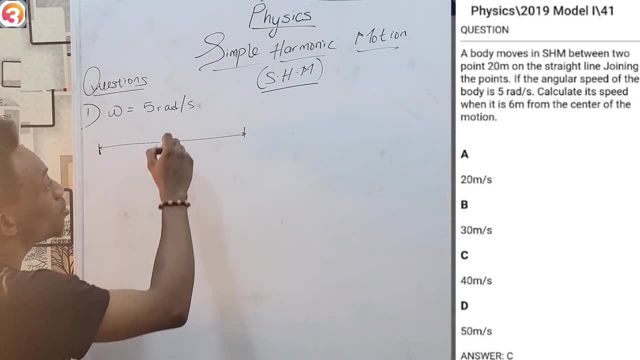 is 20 meters And our body is oscillating across this 20 meters. Now, what I must know is that if the body is moving this entire distance, then my equilibrium position must be somewhere in the middle. 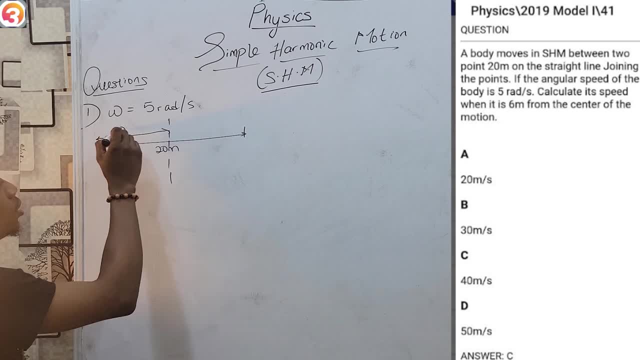 which is going to be half of 20.. distance of 10 meters. Therefore, I know that my amplitude is this middle distance, .10 meters, And I am being asked to calculate the velocity when it is. 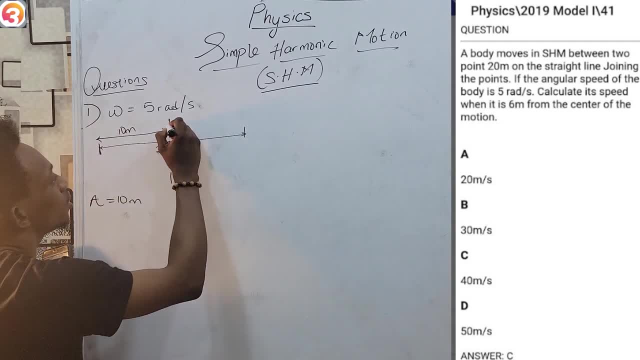 .6 meters from the center. Now, if this is my center, as my body wants to start moving. it starts in the center and moves either left or right. it moves rightwards a distance of 6 meters. 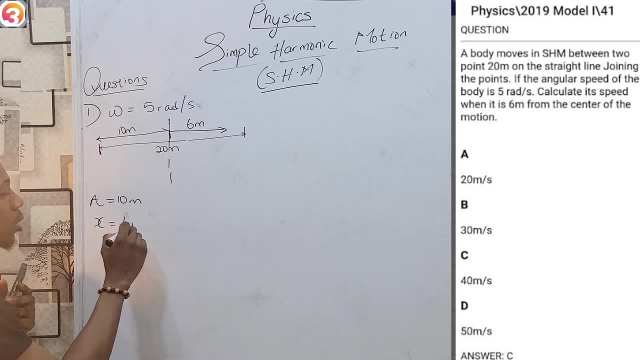 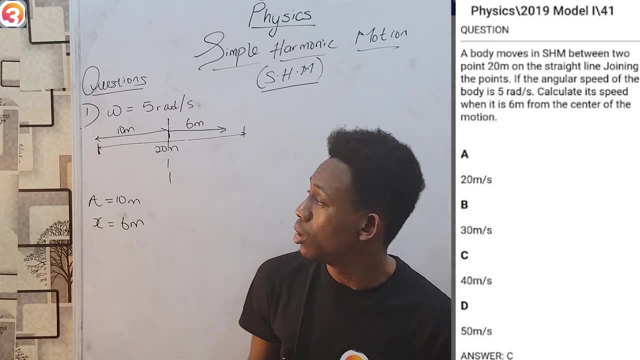 Therefore that means x must be .6 meters. So you see how we did the analysis. If this body is moving a total distance of 20 meters, then the amplitude must be half of that, because the equilibrium position must be. 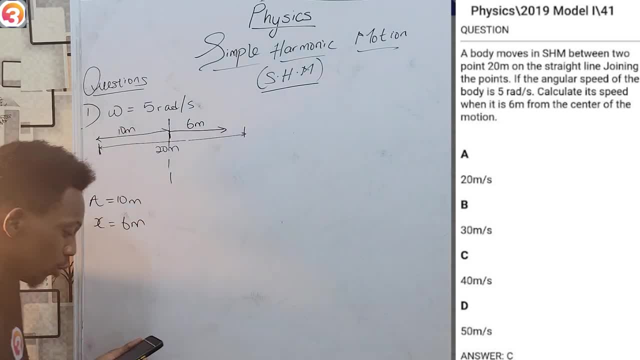 in the center plus 10 meters, While we are finding this velocity at a distance, or when it is 6 meters from this center. that is my displacement from center to the left by the letter x. 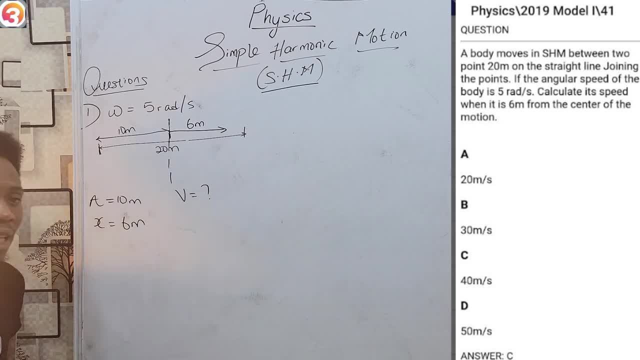 So I want to find v, And if you recall from the formulas we have for this kind of equation, this is my best formula to apply: v equals to omega square root of a squared minus x squared, And that gives me that. 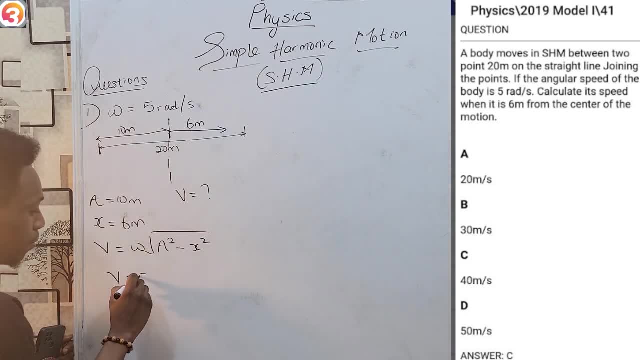 v equals, my omega is 5.. square root of a is 10. and x is 6.. So that becomes .5 root. .10 squared is 100.. .6 squared is 36.. 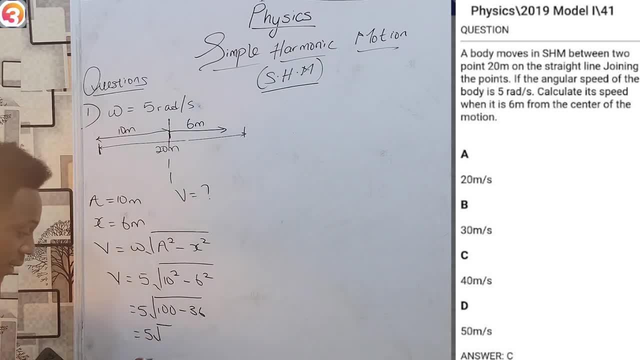 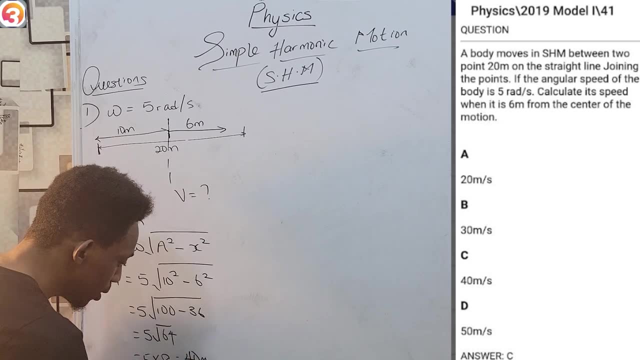 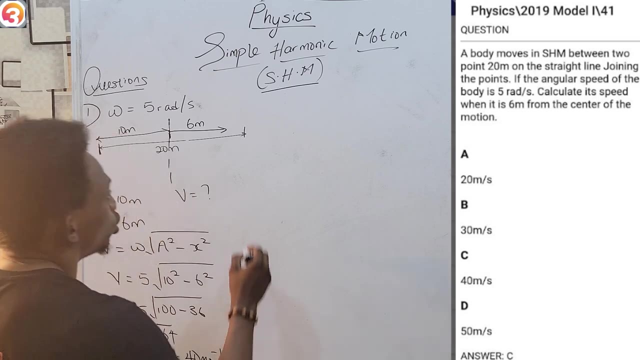 And .100 minus 36 is .64.. That becomes 5 times 8. which gives us .14 meters per second, And if I look at my options, that is very obviously option C. 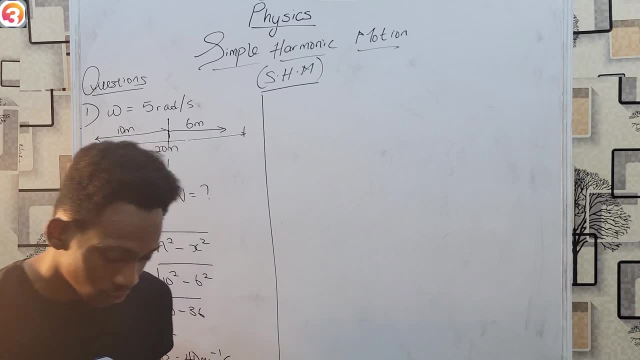 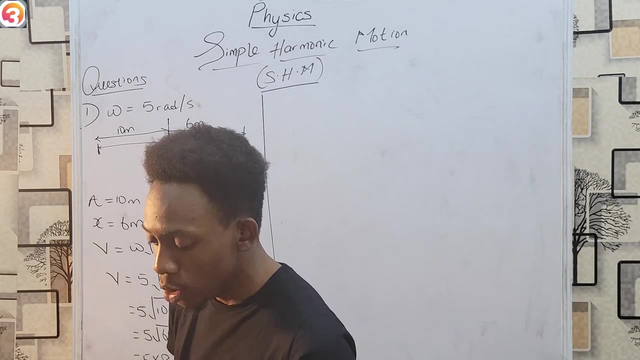 So you see, our methods are simple and precise. For our next question, still on an old three schools jam back. we are now looking at question from the year 2018.. model 3. question 19.. 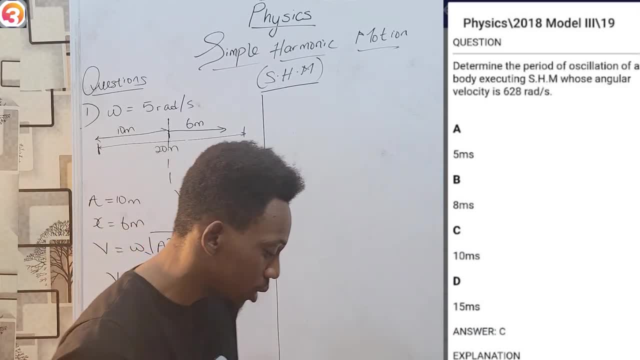 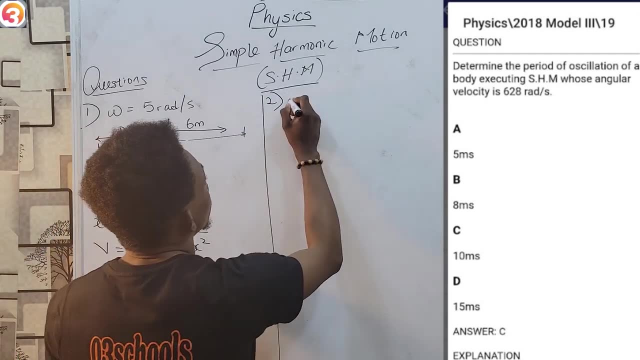 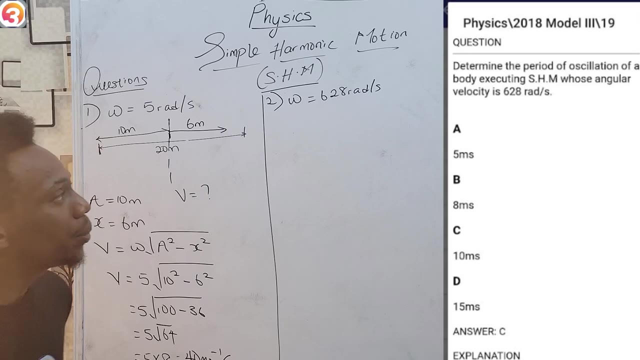 In this case, we have been told to determine the period of oscillation of a body executing SHM whose angular velocity is .628 rad per second. Right to determine the period. 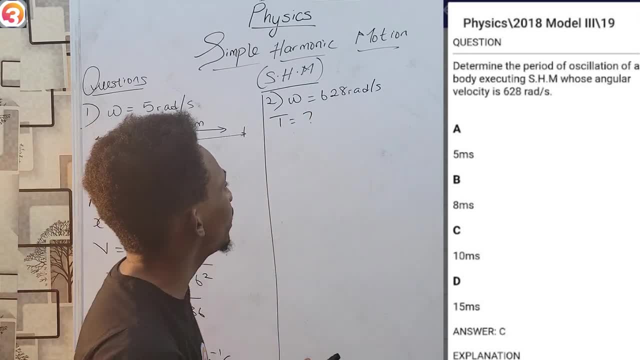 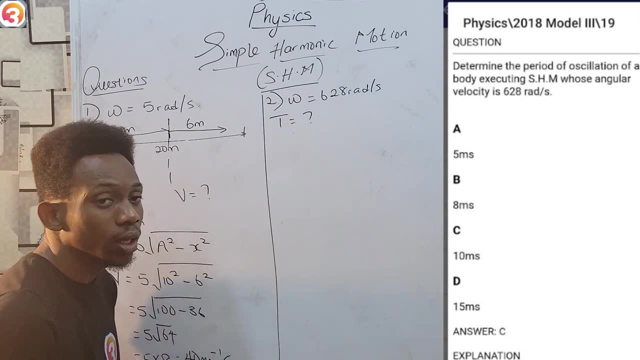 of oscillation. Now, based on what I know, Omega and C. I ask myself: is there any formula that relates Omega and C together? And I should remember that angular velocity is 2 Pi. 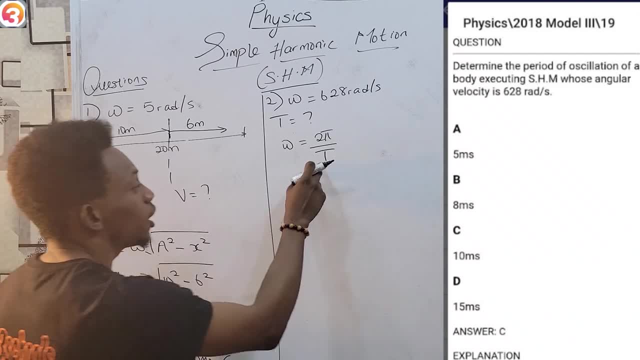 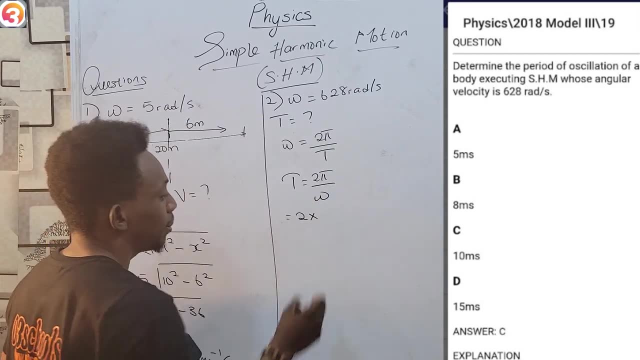 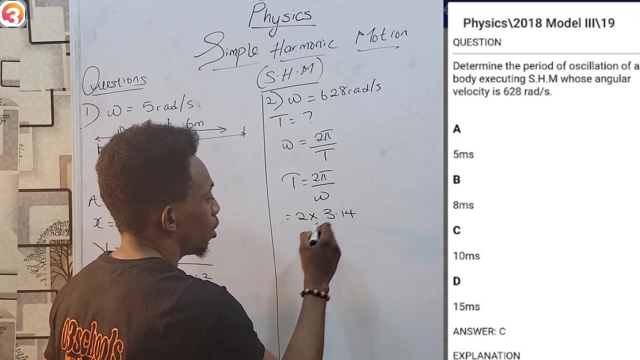 over C. Once I know my formula, I should remember that C must be .2. Pi over Omega, That becomes .2 times .3.14.. so I could just work with .3.14.. 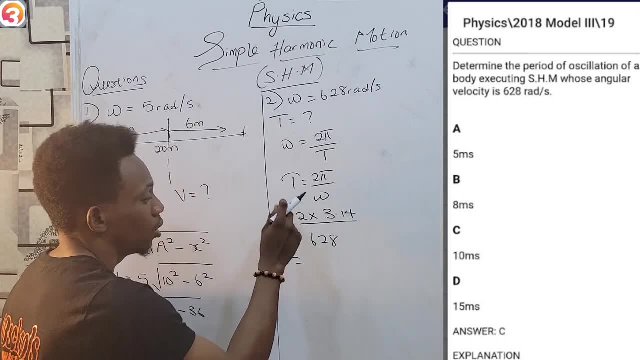 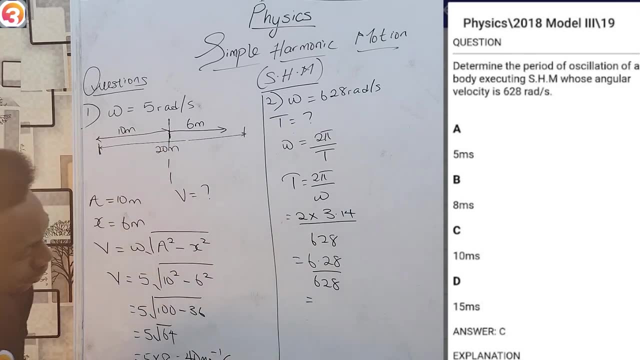 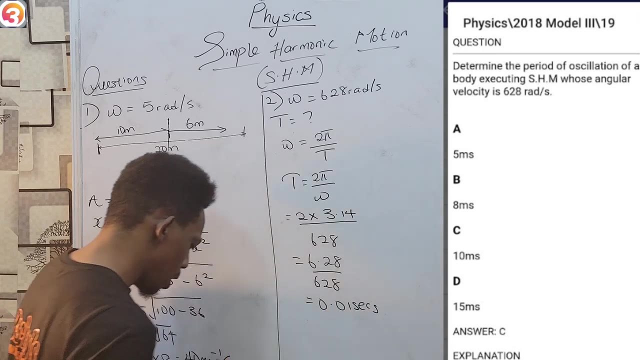 all over 628.. 2 times 3.14 is .6.28. over 628.. And if I divide this I get 0.01. seconds And I'm done here. but when I look at my options, 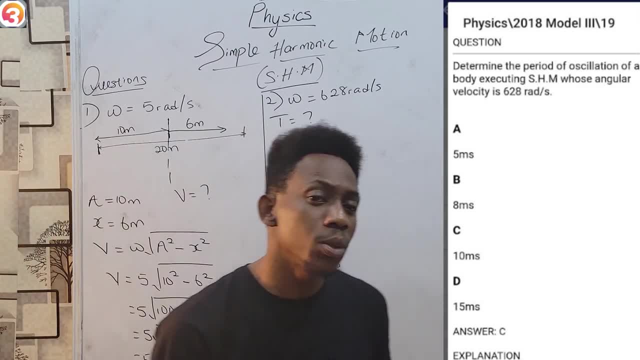 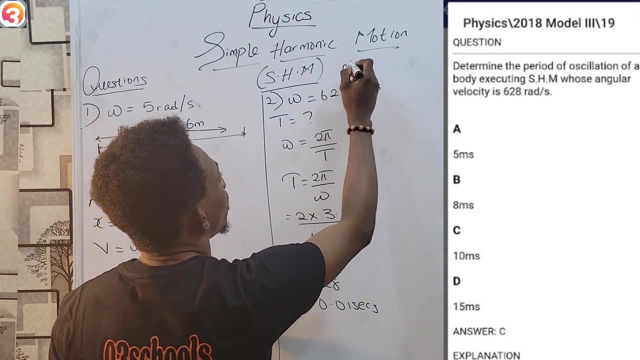 I notice my answer is not there, So what could be the problem? When I can spot my units, I realize. all my units, instead of just being in seconds, seem to be like this. MS Now, obviously I'm solving for time. 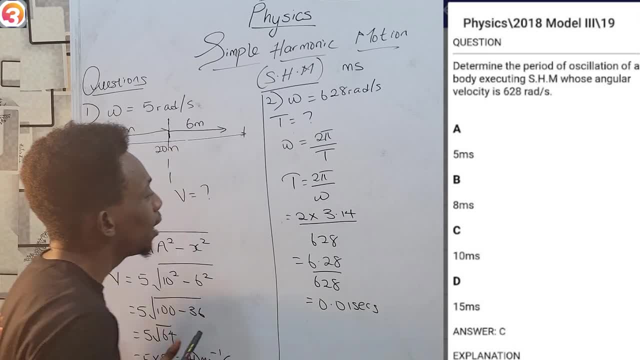 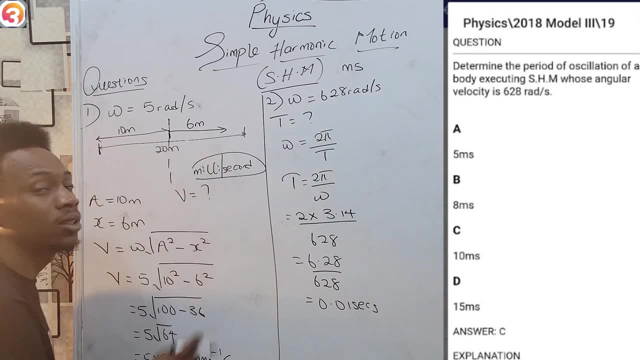 so this cannot be meters. second, instead, this must be millisecond. That means they gave me my answer in milliseconds and not seconds. That's why I have to ask myself: how do I convert this, my value, from seconds? 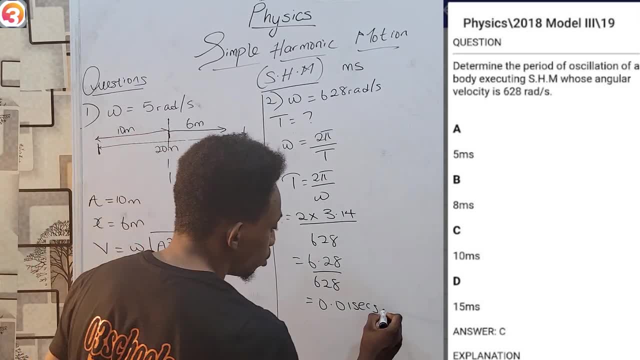 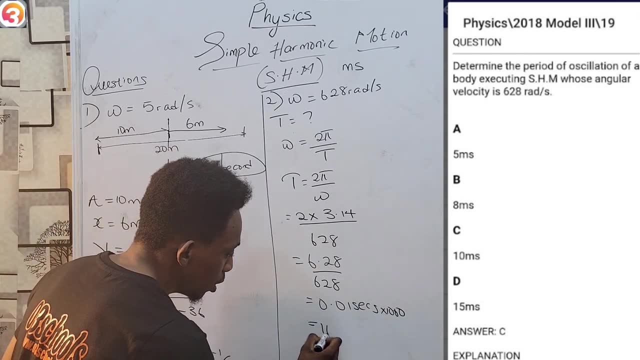 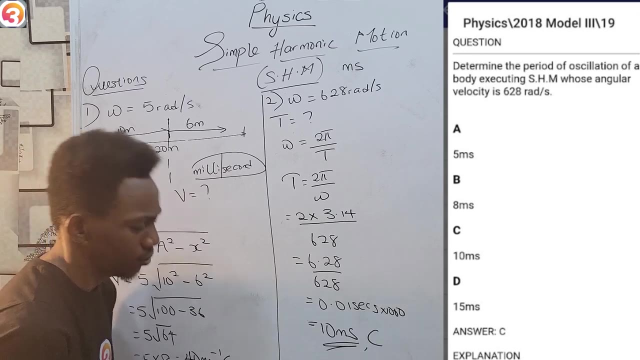 to milliseconds. And to do that is very simple: you multiply by .1000.. So 0.01 times 1000.. gives me 10. milliseconds, And that would be option C. So you see. 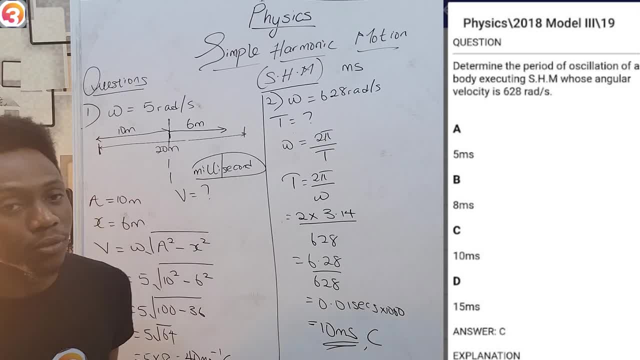 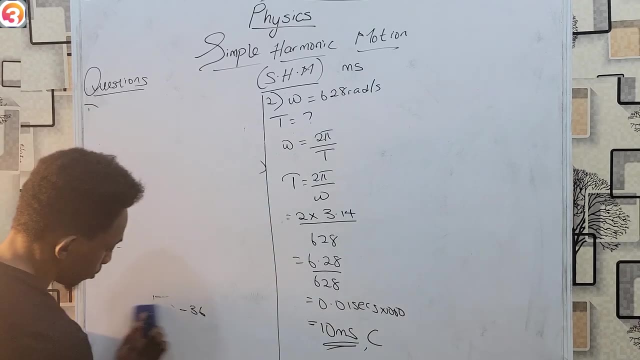 questions are simple. all you have to do is have a good handle of the many formulas in this topic and your solving is very simple. Okay, We'll move on to the third question Now, this one. 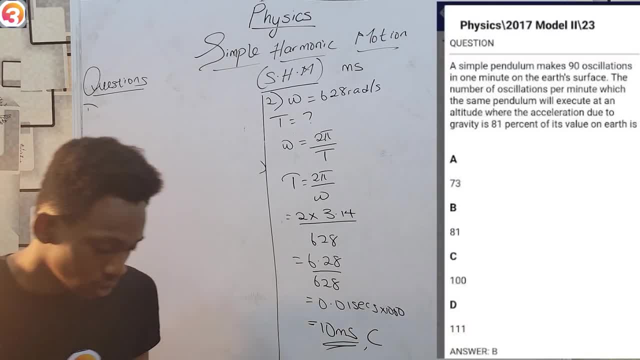 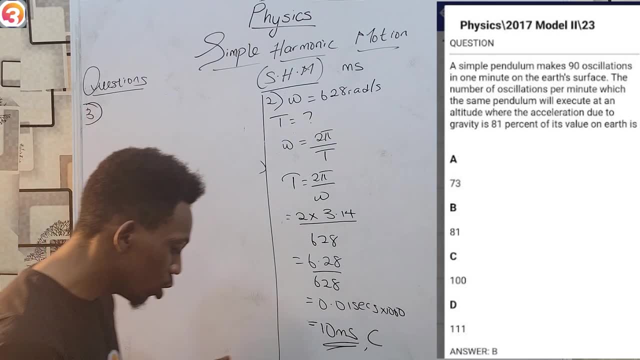 comes from the year 2017.. model 2. and the question number is 23.. on our old 3Schools jump app. So the question goes: a simple pendulum makes .90 oscillations. 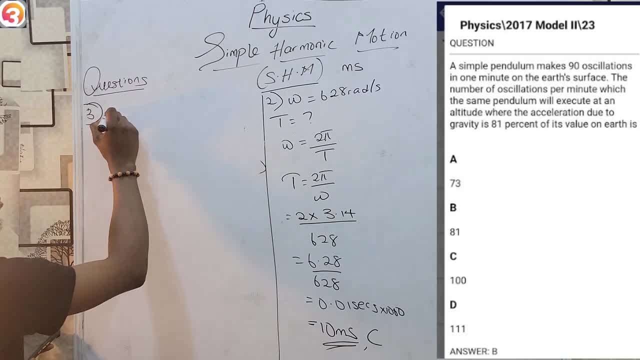 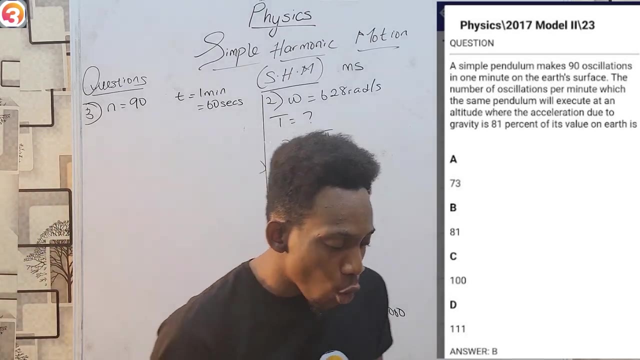 in 1 minute on the X surface Makes 90 oscillations in 1 minute, And we know already that a minute is 60. seconds. Okay, Then the question goes: the number of oscillations? 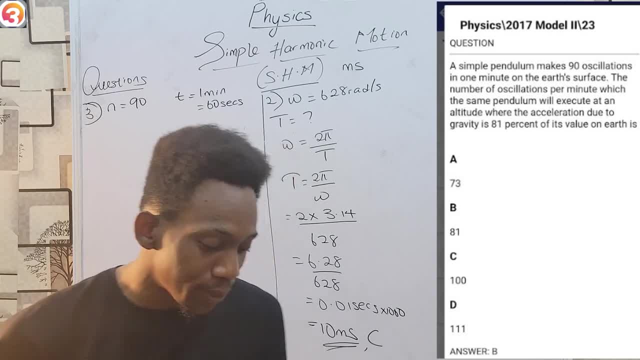 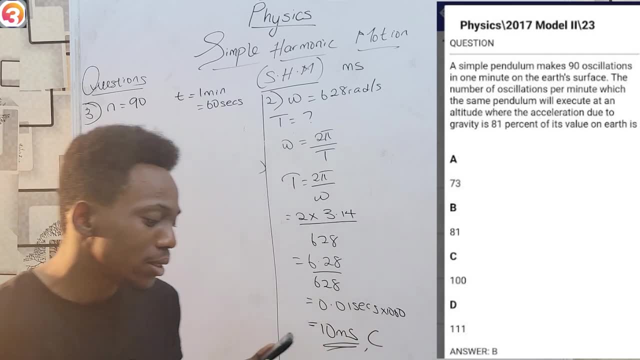 per minute: the number of oscillations per minute which the same pendulum will execute at an altitude where the acceleration due to gravity is 81% of its value on Earth. 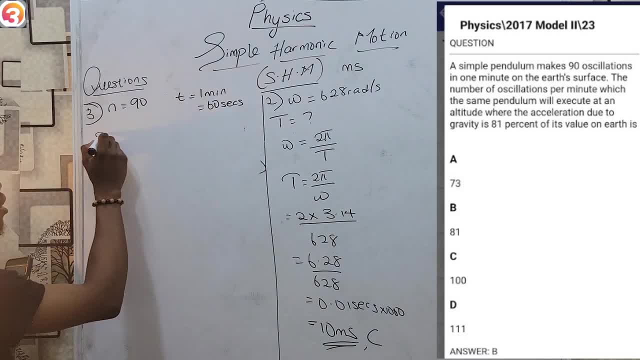 Now I'm just going to represent the ending of this question by saying: attention due to gravity at a certain altitude is 81%, that is, 0.81.. of the normal value on Earth, and write that as simply. 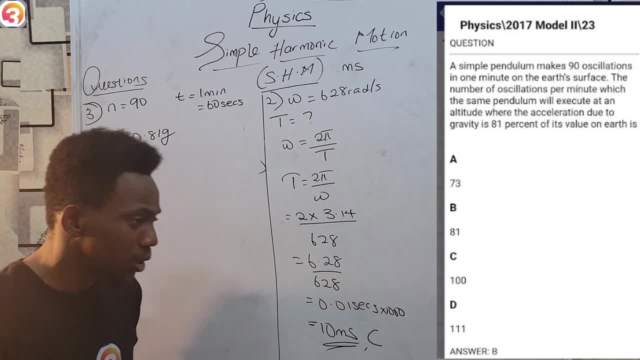 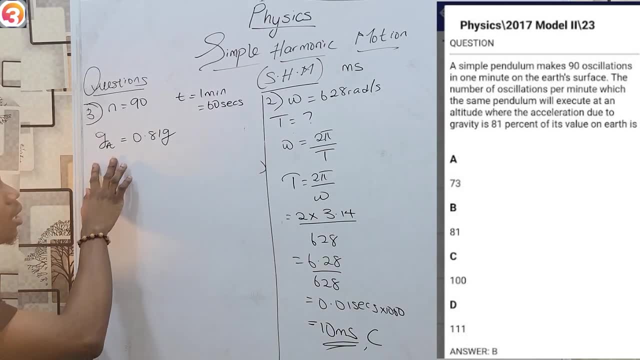 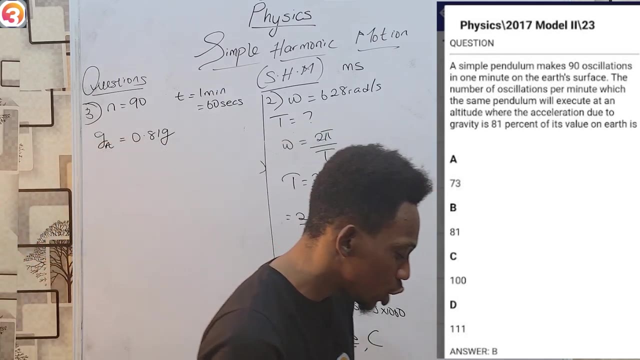 G. So that simply tells me one thing: that my pendulum is the same, but something is altering, and that is attention due to gravity. Now, before I go too far, if I look at the question, 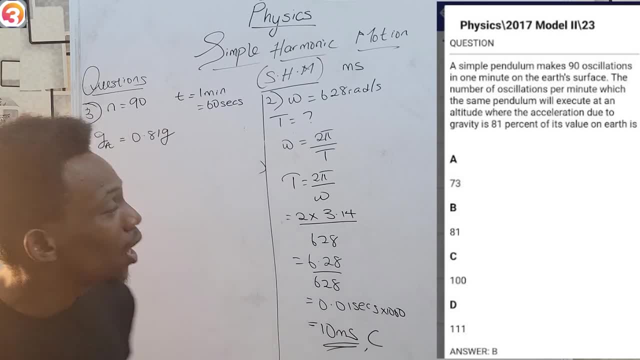 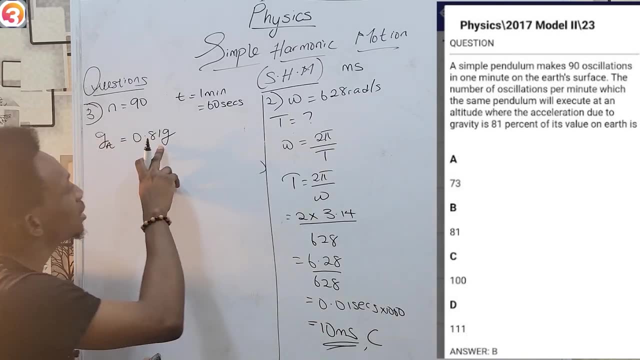 per minute, oscillations per minute. I could simply tell myself which of my terms can I relate to: attention due to gravity, based on what I have, and then I should be able to remember. 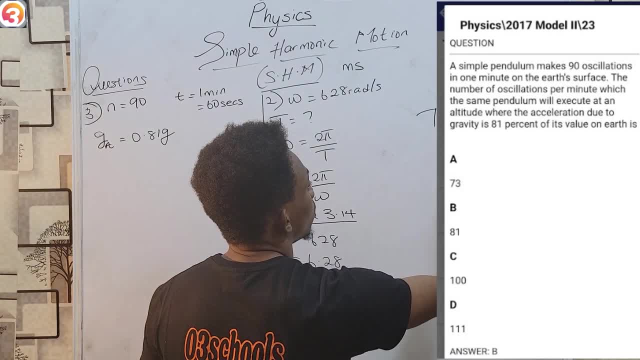 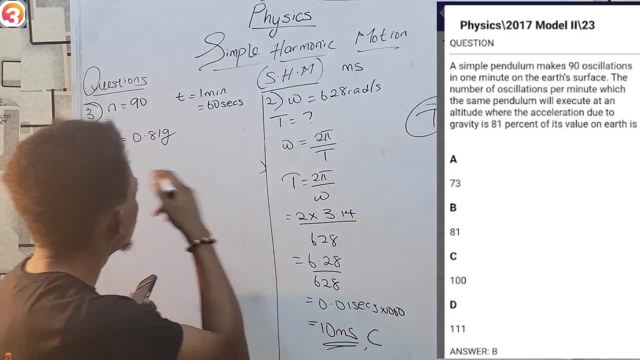 that period C equals to 2 pi square root of L over G. so you can say the relationship between period and G. when is that knowledge of value? I can saylet me get my period first. 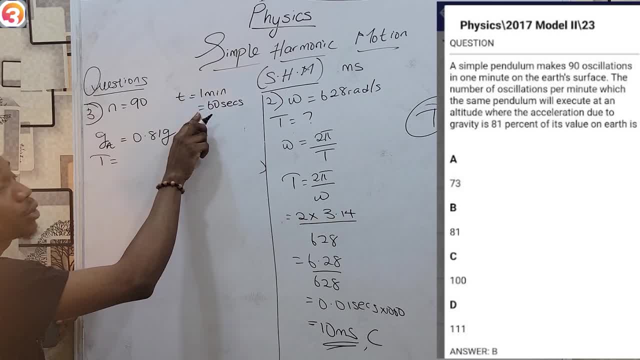 my period here would be. period, as you are aware, is time taken to complete my oscillation. it would be time 60 seconds over 90.. and that gives .0.67. seconds. 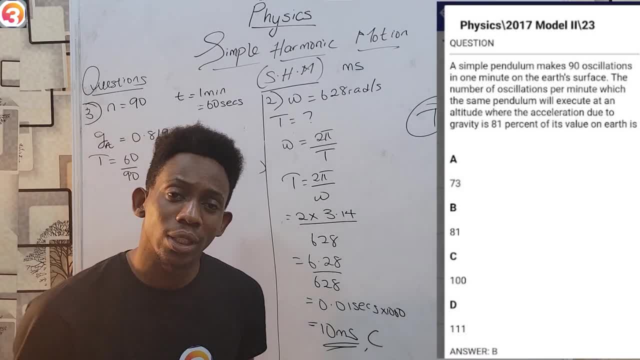 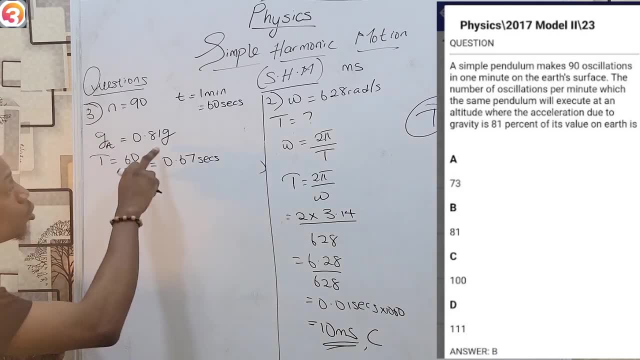 so that's my period and then, if you also analyze this, you can realize that things are changing. I have two different. I'm going to find another period because I have two different values. I have normal G. 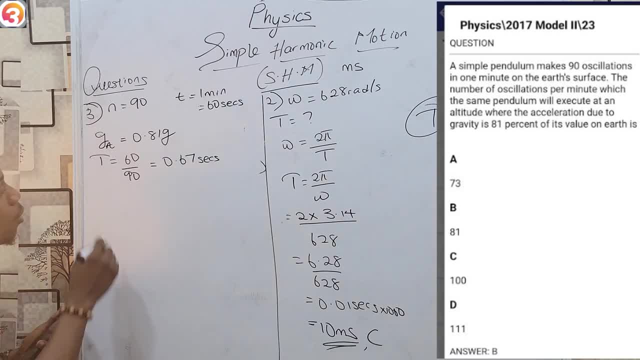 and I have G at this altitude. so, to be clear with everything, I will call this one C1. and my normal G G1.. so that I want to find C at that altitude. I'm going to be having C1 and 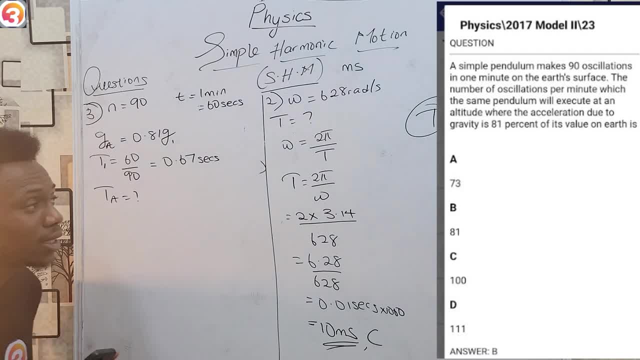 G, or rather C1 and CA. now let's look here at this formula and ask ourselves: can we try a bit of manipulation to get our answer? we realize that .2 pi is a constant. 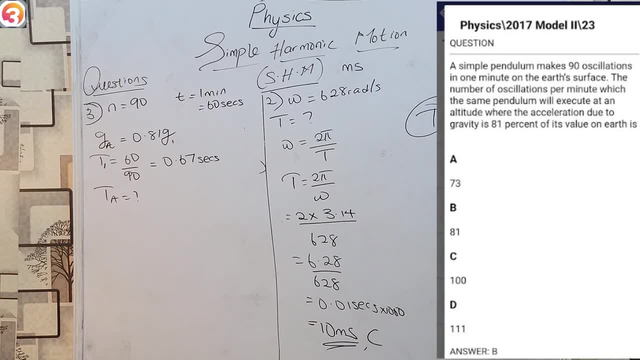 and this square root of L over here is to remain constant as well, because it's the same pendulum. it's really changing location. that means the only thing I should be having here is C a constant. 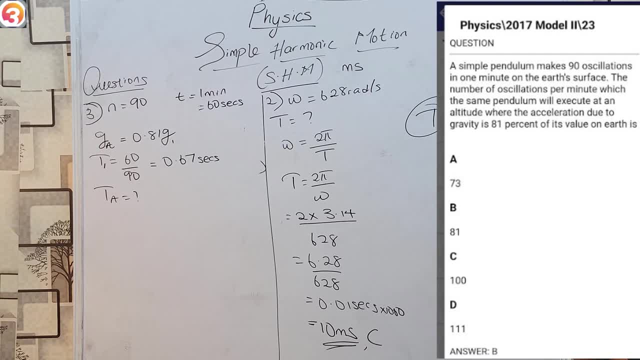 then this square root of G is down and from this I should be able to tell that C1. square root of G1. should be equal to CA square root of GA. 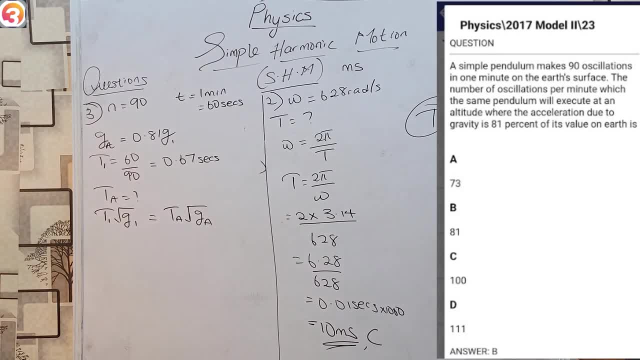 because, as you can see from here, if I cross, multiply my constant case T square root of G, that means any T that has any period and the square root of its gravity should always come back and give me the same value. 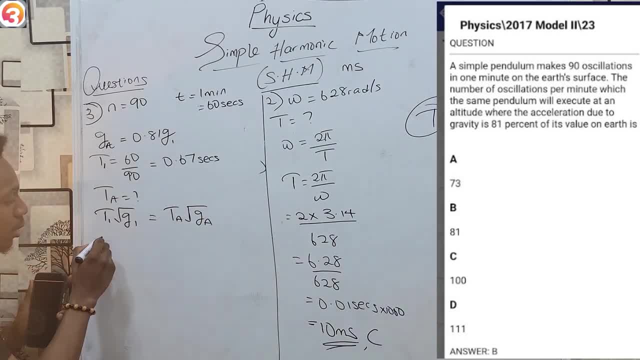 so from here, my T1 is .0.67.. then my G1.. to the gravity. but just because I notice that I have a relationship between these two, I can leave G1 like this: 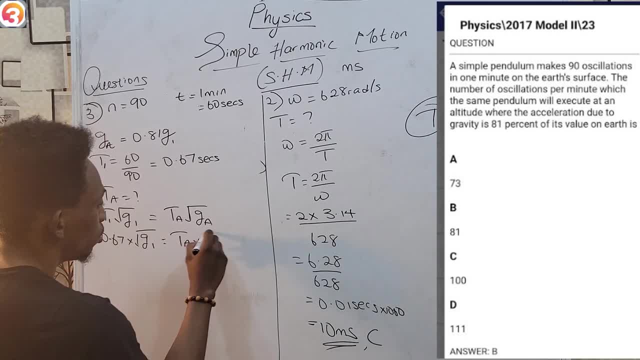 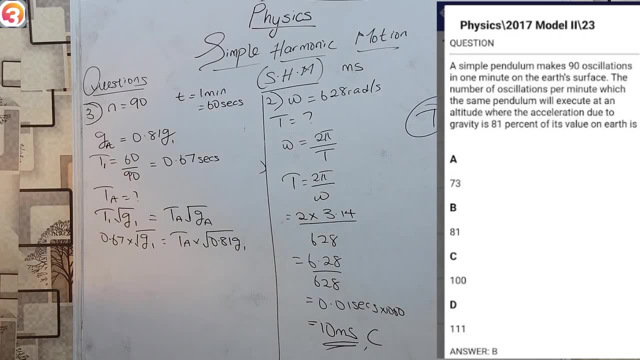 because I'll be having CA times square root of instead of GA, I can put in 0.81. G1.. and why did I do so? because I know to get CA deviable sides by square root of 0.81.. 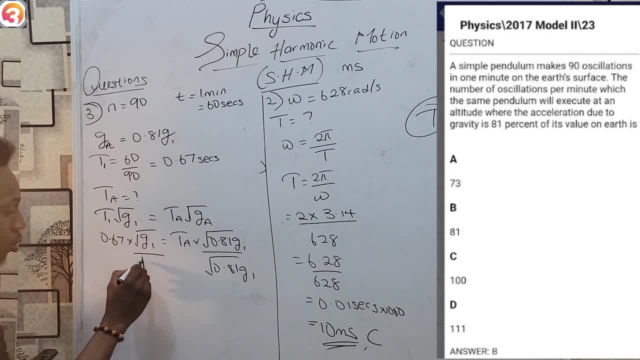 G1.. divided by square root of 0.81.. G1.. this cancels out CA, becomes equal to now. this square root of G1 here is affecting both, so if I separate it, 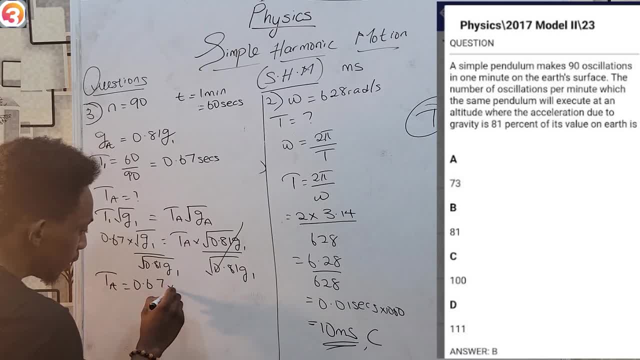 I can have 0.67. times square root of G1. over. let's put them under the same square root over 0.81. G1.. this G1 cancels G1.. 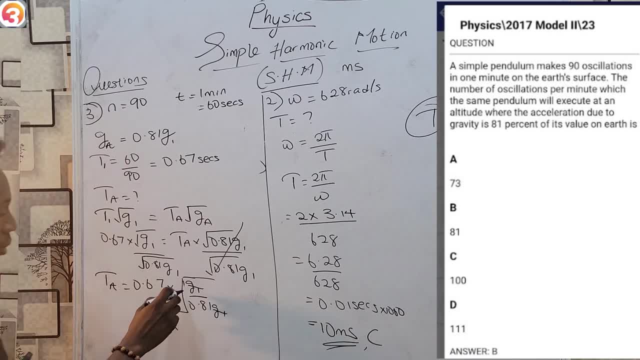 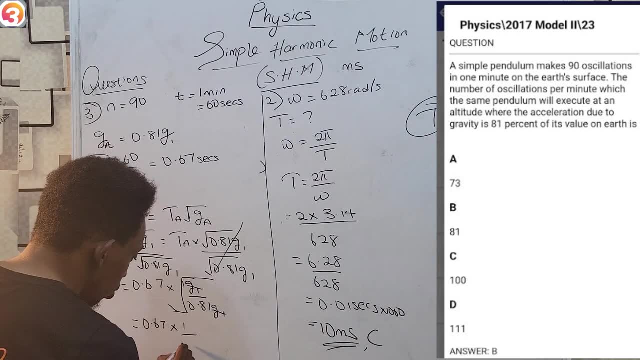 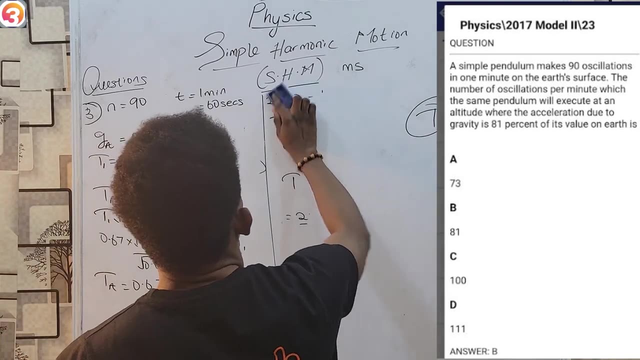 that becomes 0.67.. times square root of 1., which is what is left as the numerator. square root of 0.81. is 0.9.. okay, so cleaning this up so we can have some extra space. 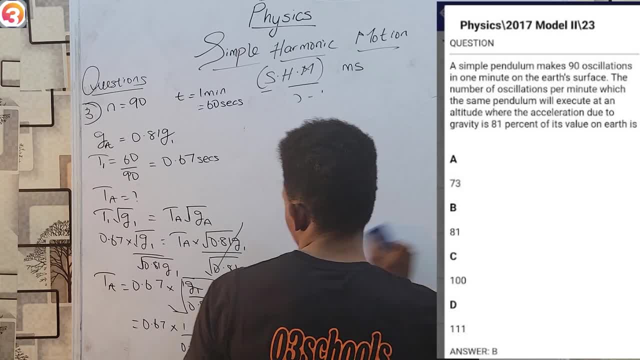 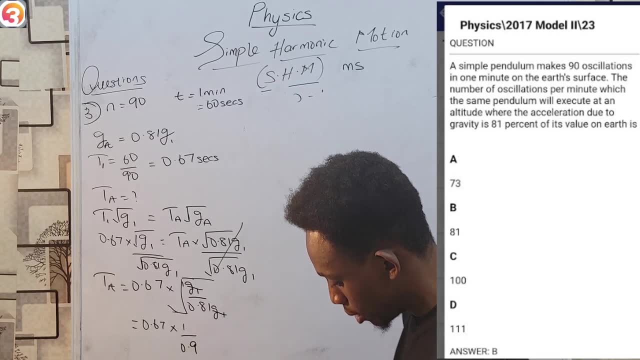 to solve. we can deposit that using our calculator. let us find .0.67. times 1 over 0.9.. so over 0.9.. so 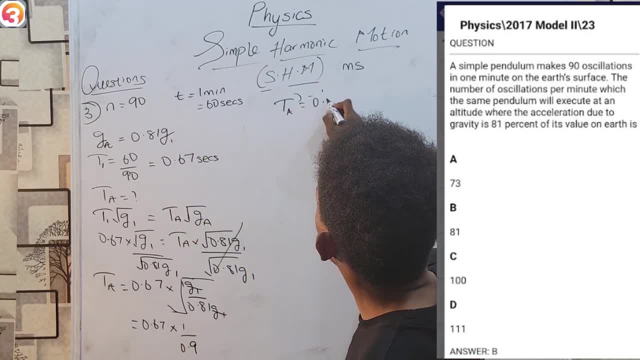 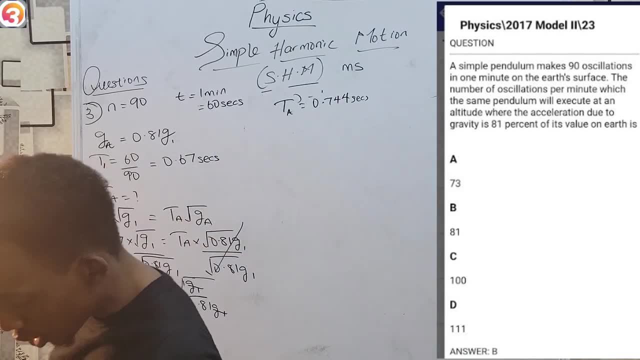 Ca should be equal to .0.744. seconds. but please always be careful with what we are asked. what we are asked to find in this case was number of oscillations per. 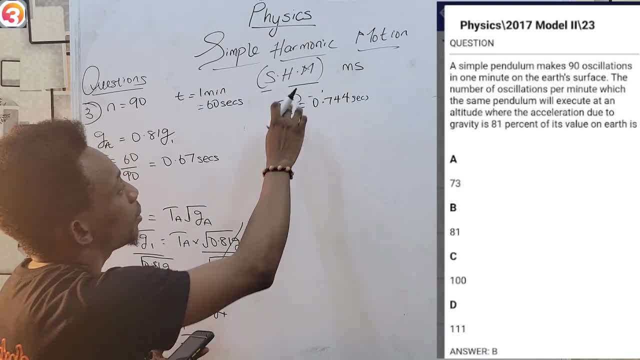 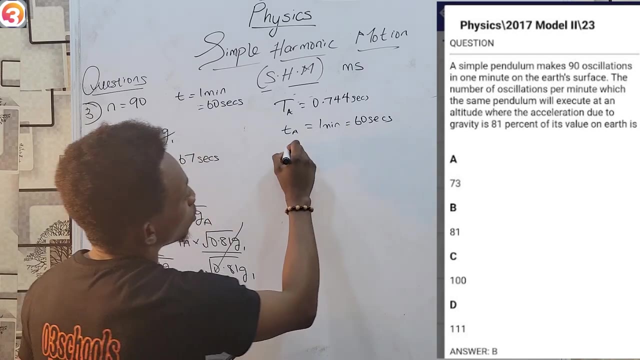 minute or number of oscillations. that means in this case, Ca is this, and then this time to be taken for these oscillations here is 1 minute, which is 60. seconds. 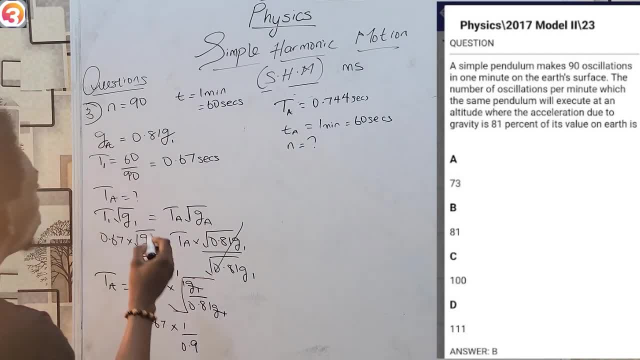 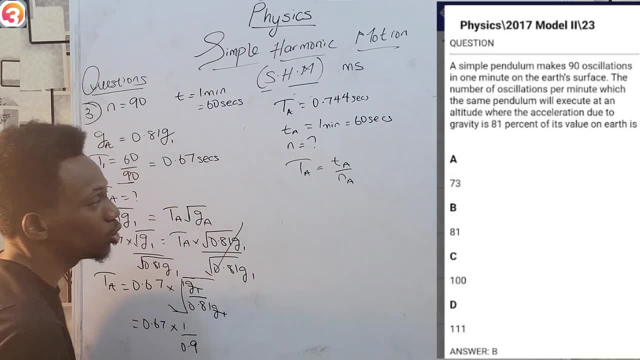 we want to find how many oscillations there will be and, as we are aware, the same formula we used here, Ca, will be equal to time over number of oscillations. that becomes 0.744.. 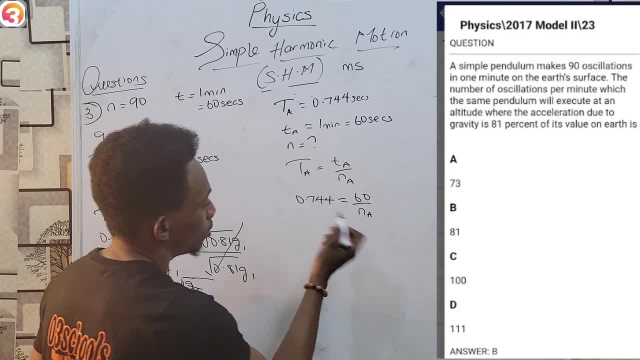 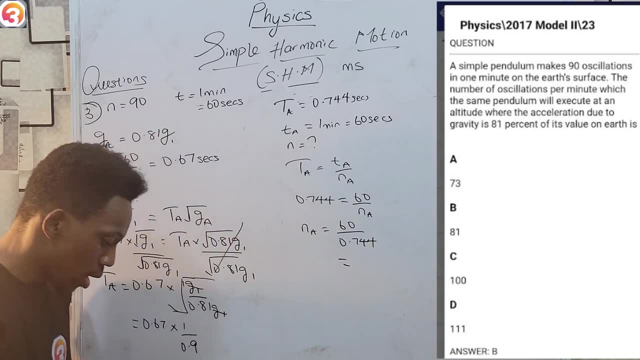 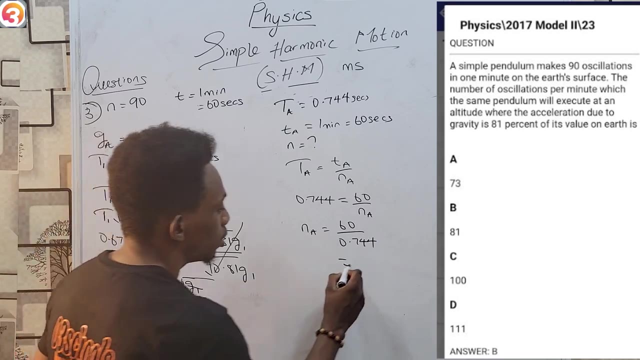 .60.. over Na and Na becomes 60. divided by 0.744.. and simply pressing that into your calculator, .0.744. gives you .80.645.. 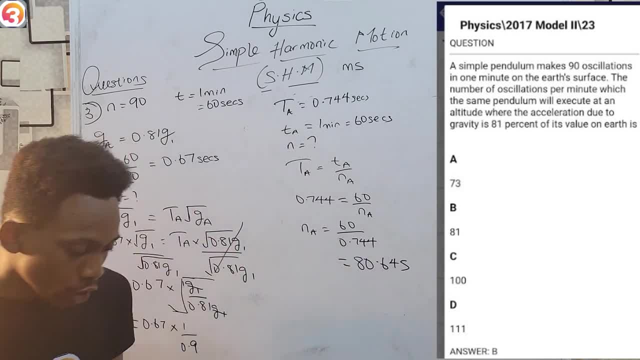 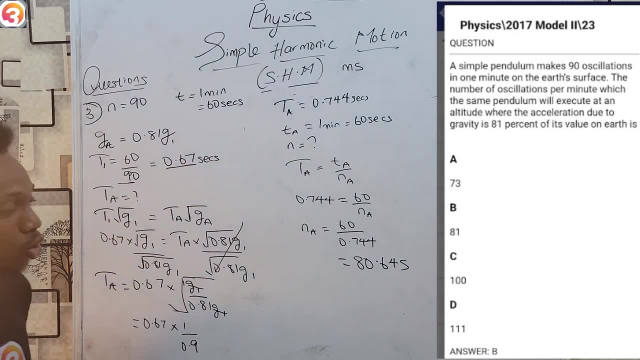 now, if you look at your options, this answer is not quite there, but only the third bit of approximation, if you can remember here. as such, we are also free to approximate this to the nearest whole number. 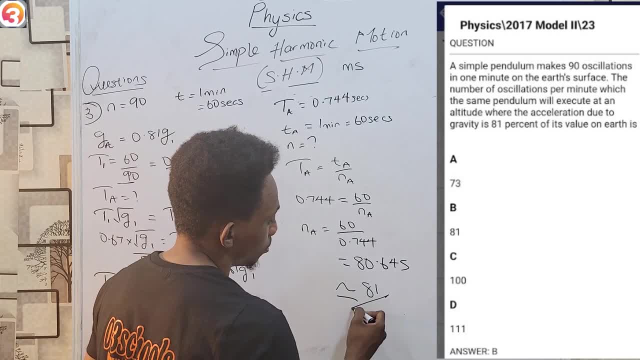 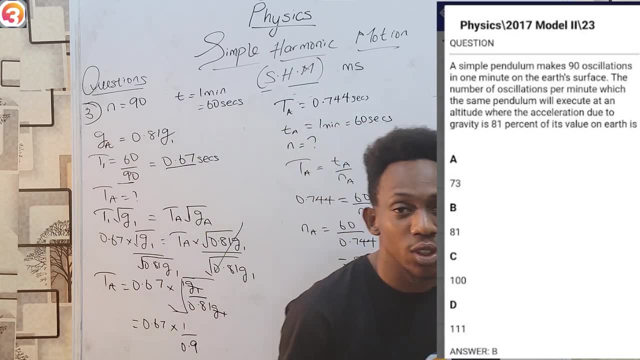 since my options are all in whole numbers, and that would be .81.. that simply means that this body completes .81 oscillations in 1 minute when it is now at this new altitude. 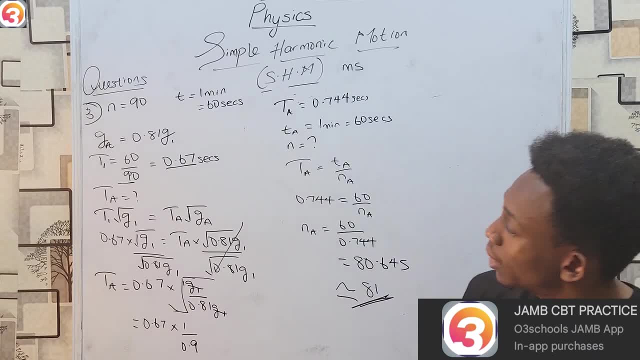 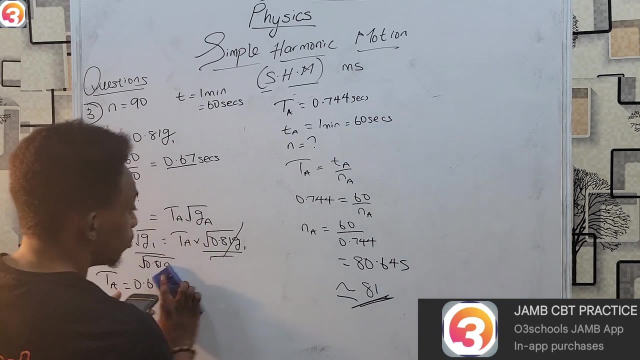 so you see, my question is not complicated. I'm just dragging out the steps here so you can solve it clearly. obviously enable to be faster with this. okay for our next question. 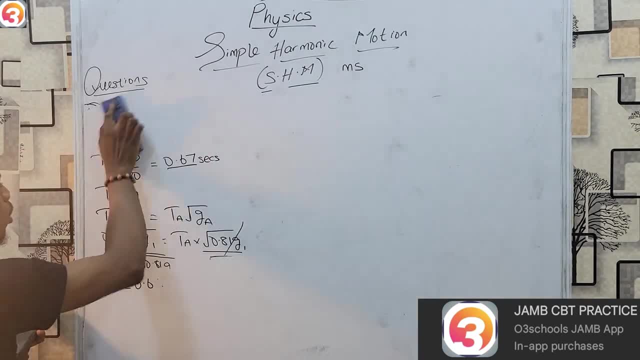 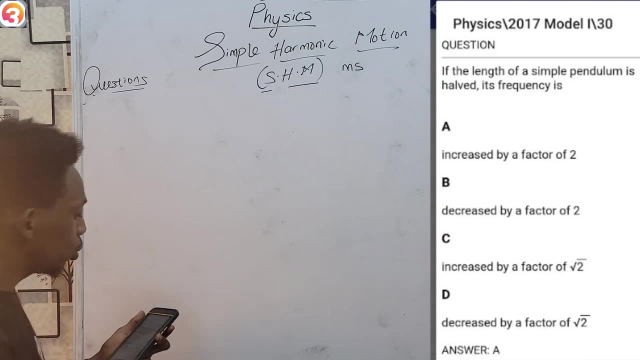 still using our old 3 school jam app. this one comes from the year 2017.. model 1.. question number 30.. .2017- model 1.. question 30.. so this is question 4.. 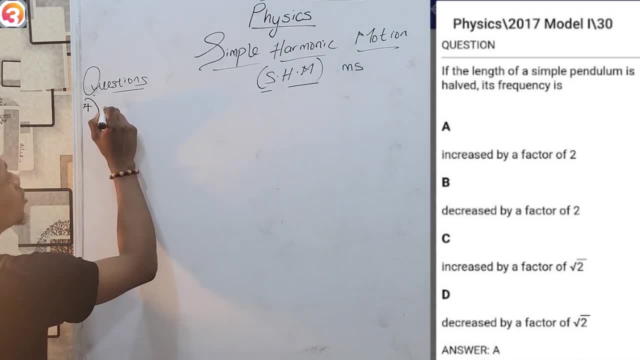 the length of a simple pendulum is halved. that means initially a halved one pendulum, let's say L1.. and then the length is getting halved. so let's say L1 equals to L. 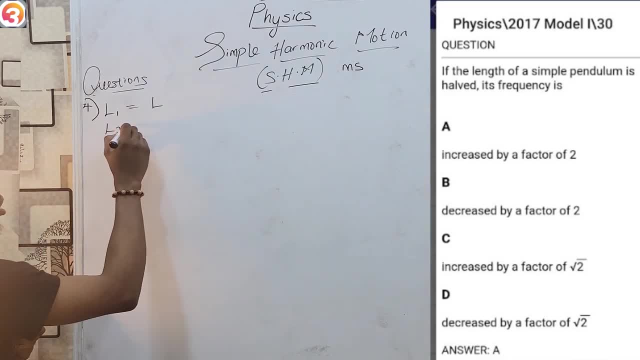 initially, then L2. equals to half of L1. which is simply L over 2.. so when the length gets halved, its frequency is what. the question now is: what happens to the frequency? 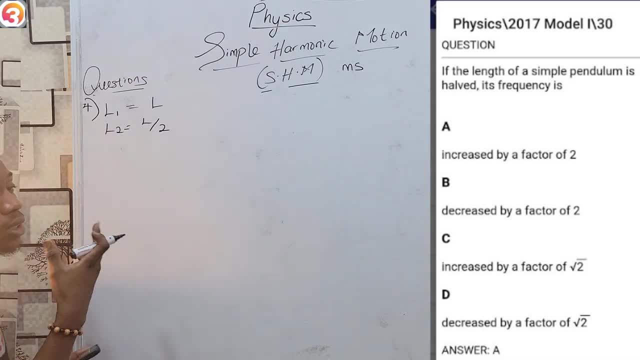 one more time. how do we look at this? we ask ourselves: is there any formula that relates frequency to length? and, as you are aware, typically we know that C equals to 2 pi square root of L. 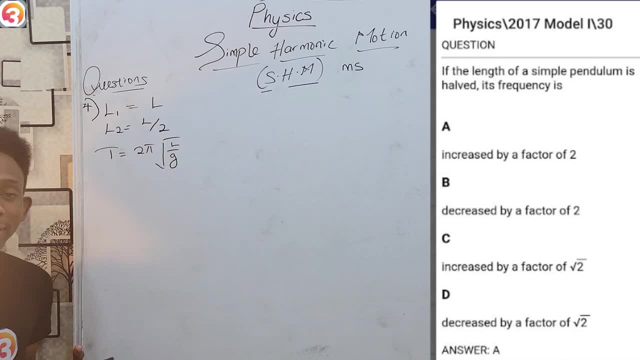 over G, but we also know that C is 1 over F. therefore, here is 1 over F. now, in this case, as you are seeing, unlike the previous one, G was constant and G was changing. 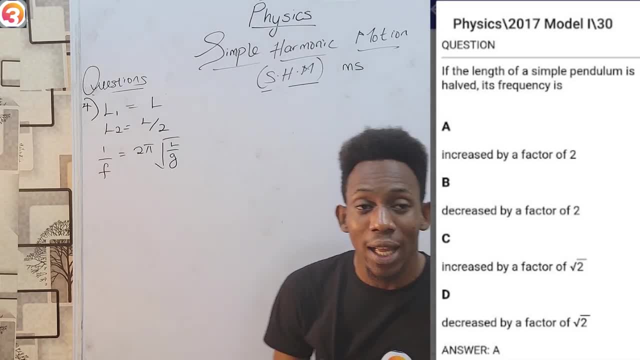 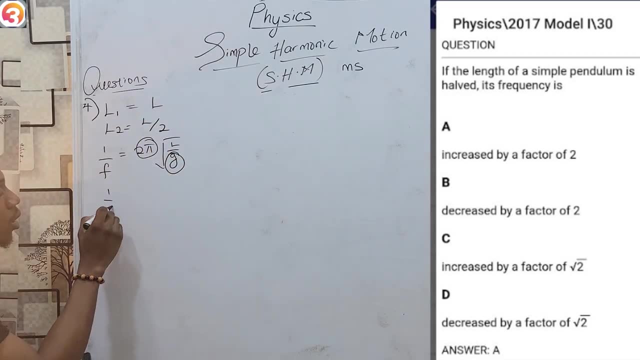 in this case, I am taking G as constant and L is changing depending that this is constant. this is constant. I am left with 1 over. F equals to K root L and. 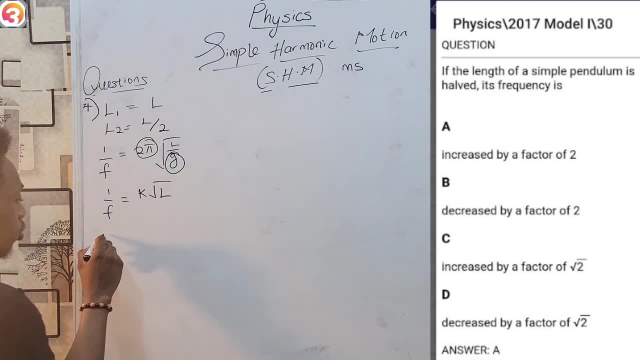 if I cross multiply, this gives me that F K root L equals to 1.. and because I actually want to see what the constant will be, K will be equals to .1 over F root L. 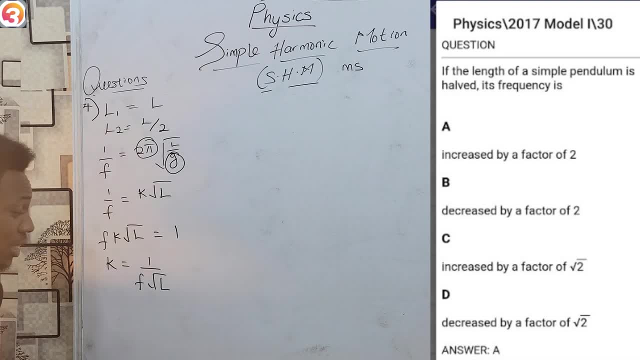 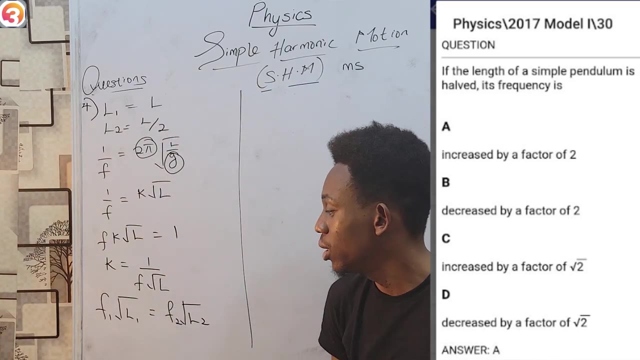 and just because I rather solve it linear, I can therefore say that F1 root L1. equals to F2 root L2.. now one more time. please note if this was your exam. 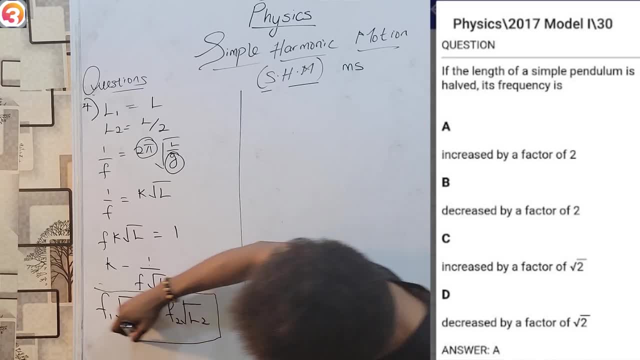 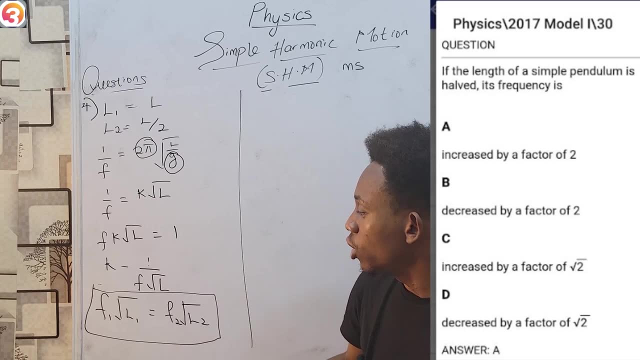 all you would need to remember is this part: that if you have an equation here, the length is changing. I want to see what happens to the frequency. you can simply do this, so you don't have to solve. 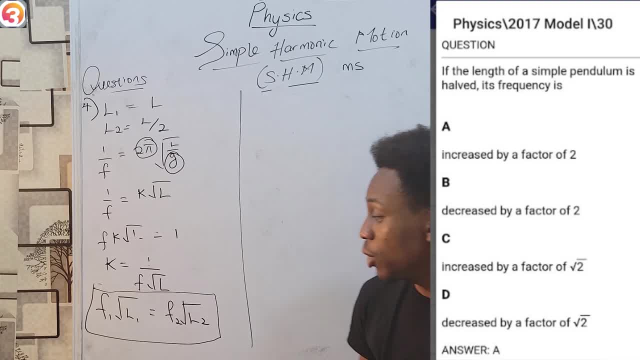 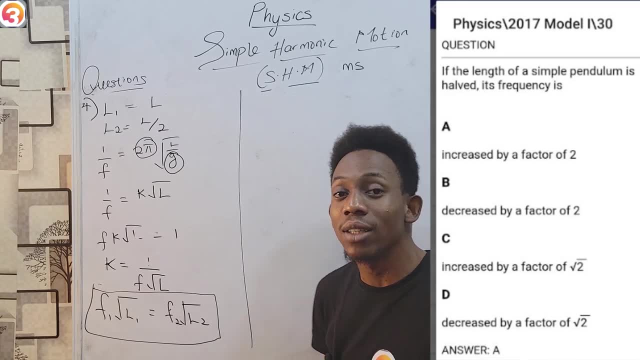 all these parts in every question. you should simply try and remember this, except for those of us who don't like memorizing too many formulas. in that case, as long as you are fast, you could still do this in exam conditions. 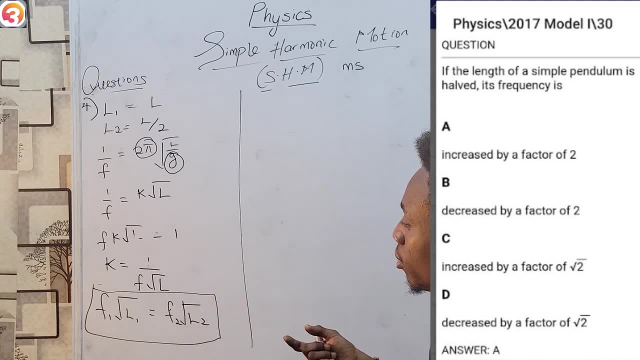 but once I know this- this is all I need- I can start my question, because you want to know what happens to the frequency. you want to know what happens to F2.. in terms of F1.. 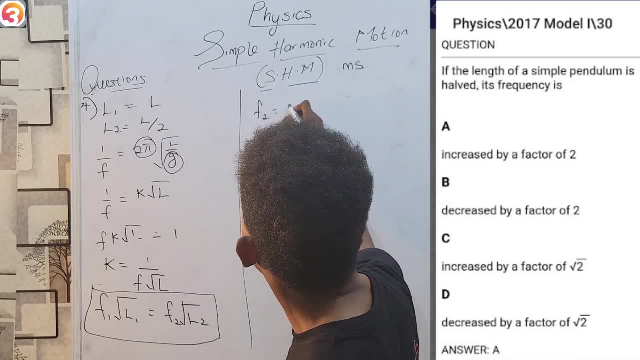 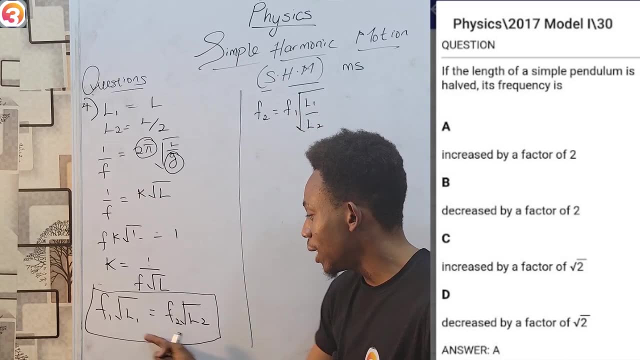 you can find F2 here and see that therefore F2 must be equal to F1.. square root of L1. over L2.. that will be divided both sides here by L2.. and therefore 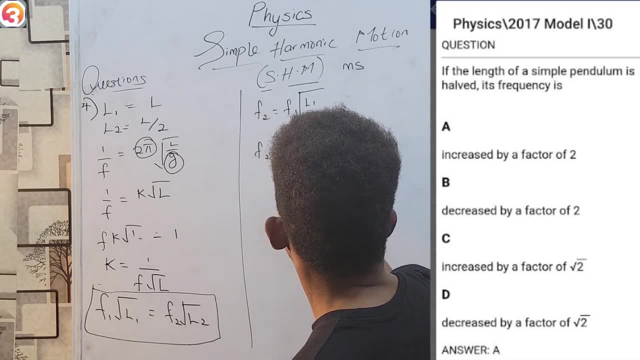 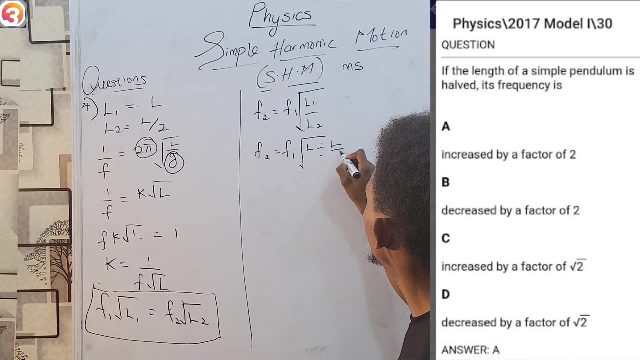 F2 must be equal to F1.. then in my square root L1 is L and L2 is L over 2.. so this is L divided by L over 2.. or, if you prefer, 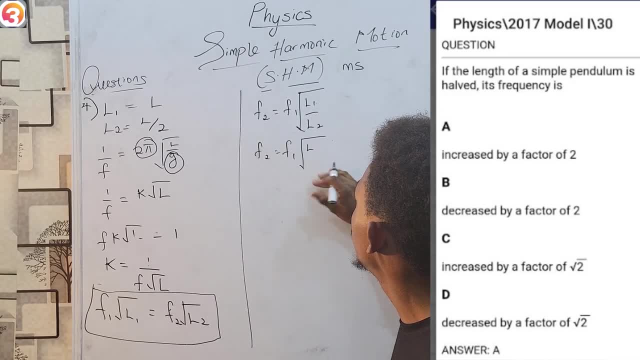 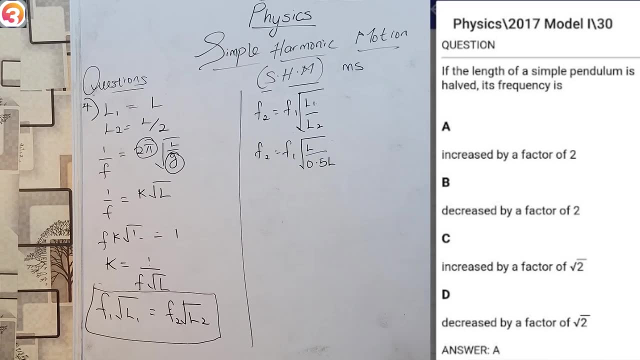 to make this solving much faster. you know that L over 2. must be 0.5. L, so that will go with division of fractions which may be a little bit longer. reason why is because I know here. 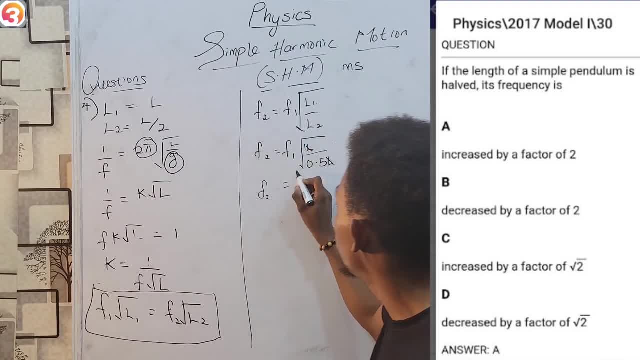 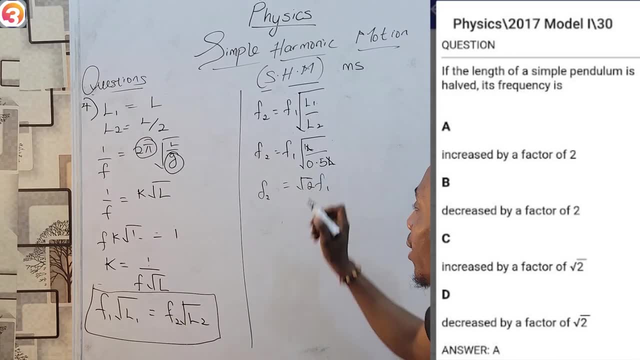 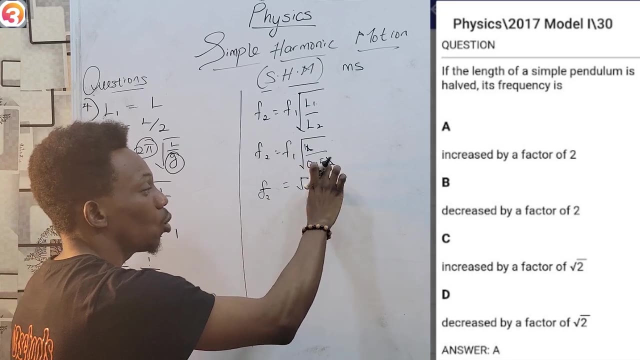 L can cancel L, then F2 becomes equal to .1 over 0.5.. is root 2.. so root 2.. F1.. indicating that my second frequency becomes a root 2 factor. 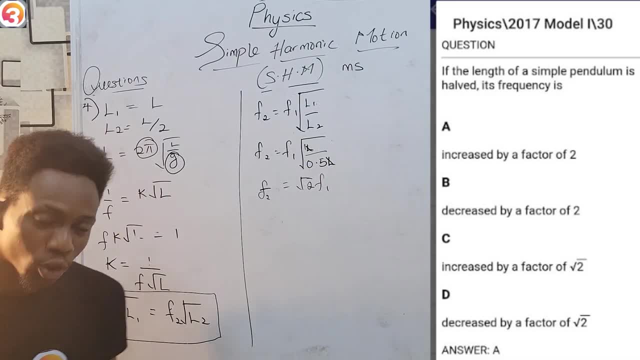 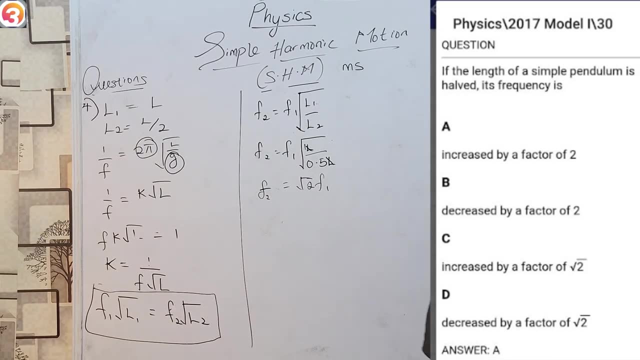 of the first frequency. so option A says increased by a factor of 2. wrong. B says decreased by a factor of 2. wrong. option C says increased by a factor of root 2. 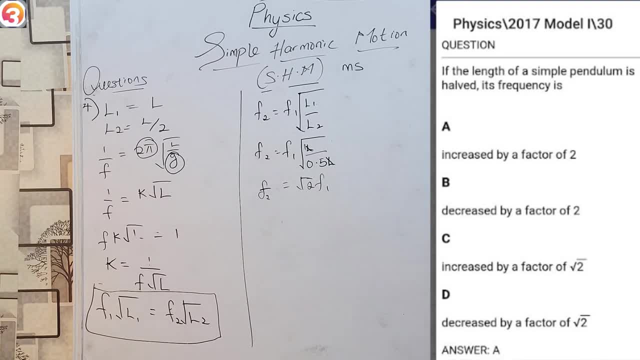 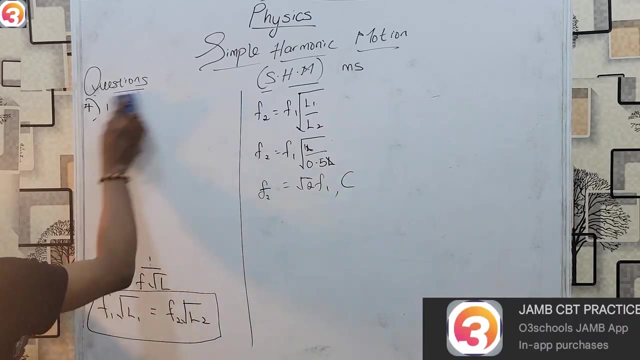 obviously it is being multiplied by root 2.. that is my answer, option C. these are all very, very, very simple. let's proceed. now we are going to the year .2013.. 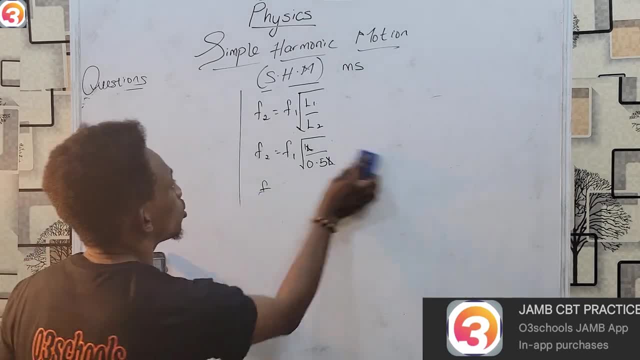 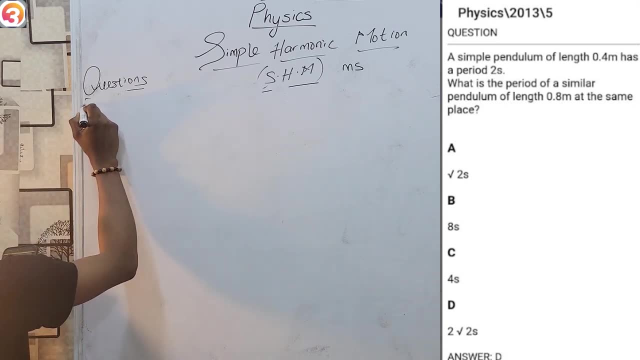 the year now is 2013.. and we are looking at question number 5.. from 2013.. this one says this should be our fifth question. a simple pendulum of length, 0.4 meters. 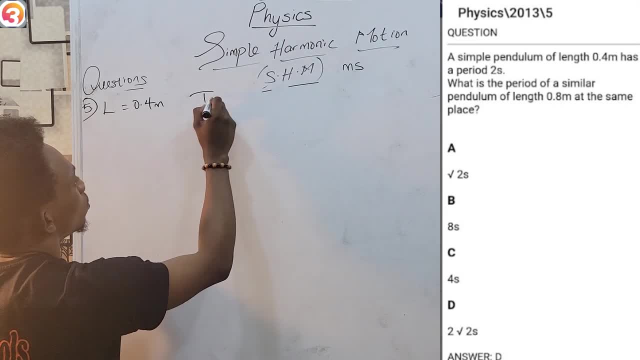 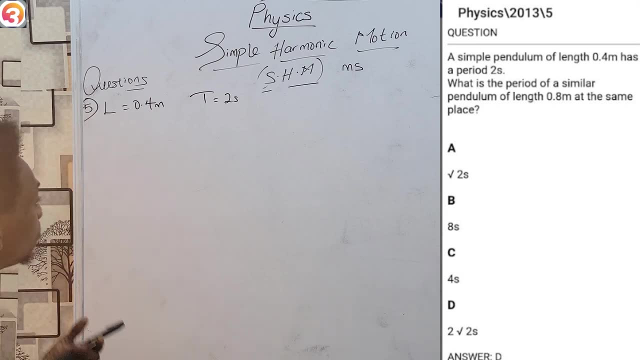 has a period of 2 seconds. what is the period of a similar pendulum? once I am doing a similar pendulum, then I have to number L1, T1.. of length: 0.8 meters. 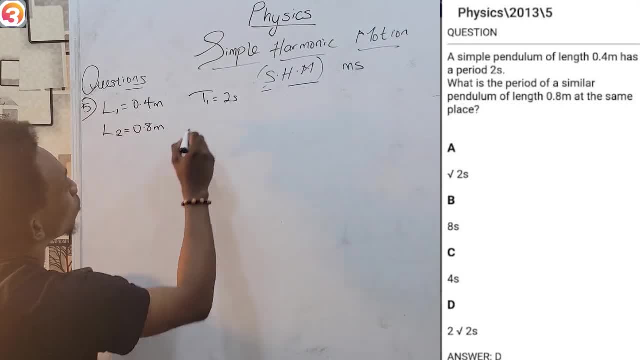 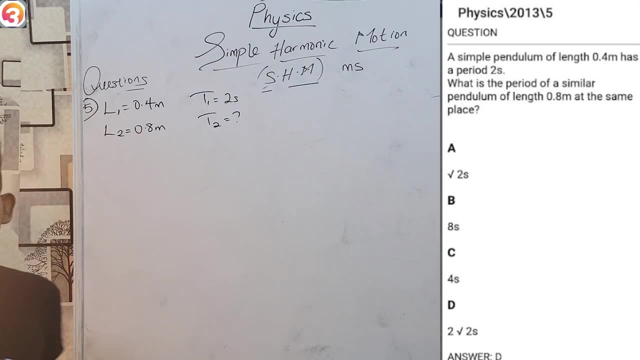 so my new length, L2., is 0.8 meters. I want to find the period of this new pendulum, therefore the relationship between T1 and L1. and so in this case, we know that. 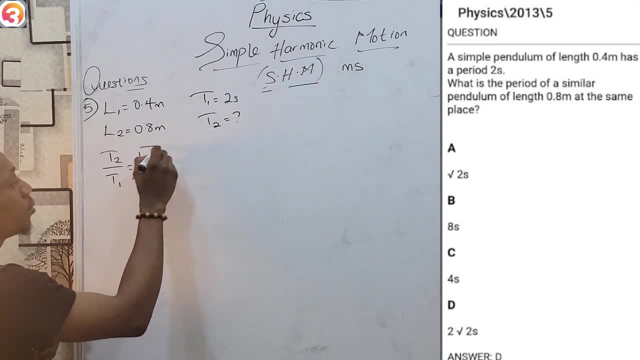 T2 over T1.. equals to square root of L2 over L1.. if you do not know how to go this, all you have to remember is this guy again: .2 pi, square root of L over G. 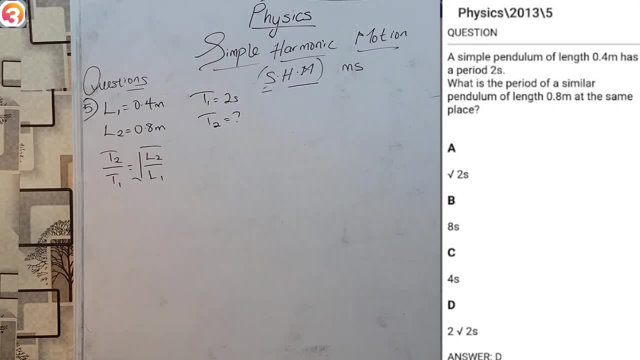 and knowing that in this case we are dealing with T and L, this is constant, so T equals to constant root L over root L over root L, so constant is T over root L. 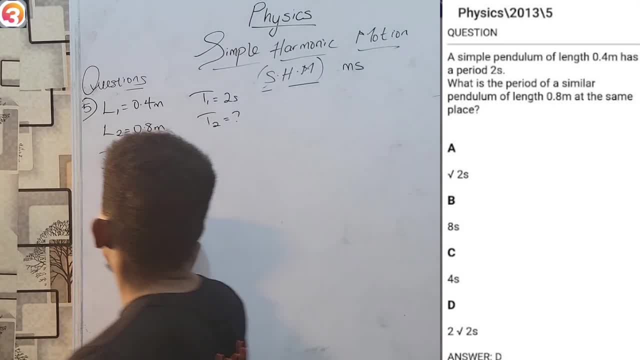 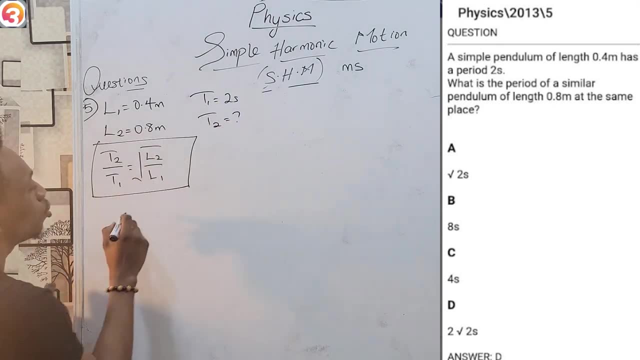 that's all. that's how I got that again. memorize this: you can deal with duration in length and period. so my T2 is unknown. my T1, though, is .2.. then L2 is 0.8.. 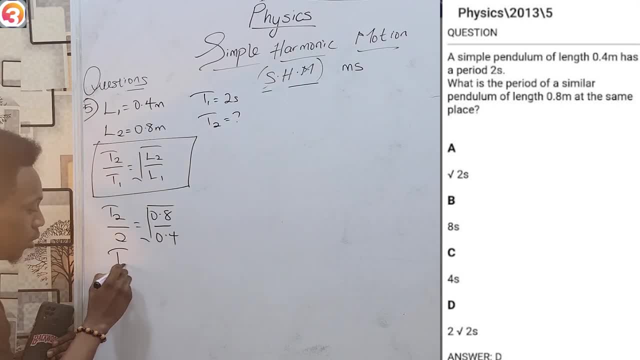 and L1 is .0.4.. so T2 over 2 equals to square root of .0.8.. divided by 0.4. is 2.. then if I cross multiply, T2 equals to 2.. 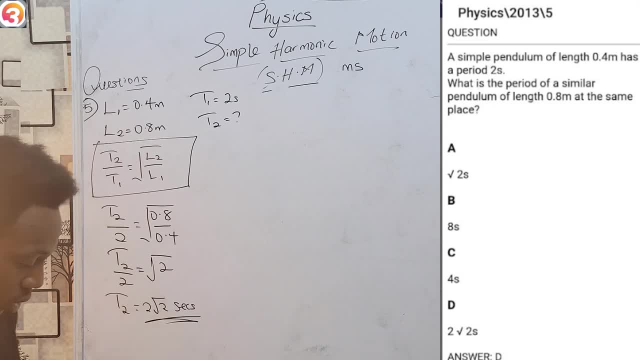 seconds and if I check my options, that is option D. so again you see, in smart money promotion, you just have to know these formulas and your solving will come across quite easily. 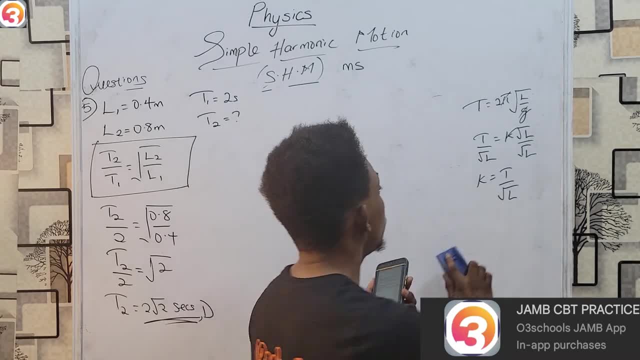 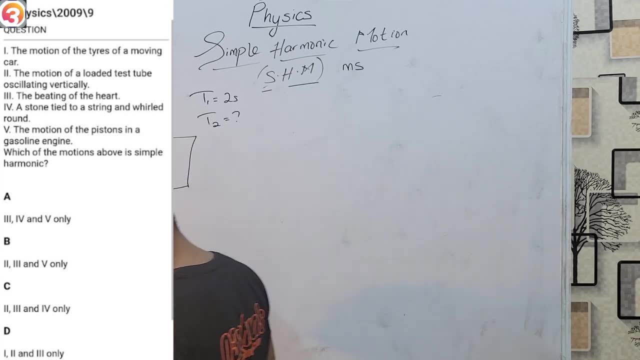 okay, our next question is from the 8009.. question, number 9.. and for this case there is no solving, it's just the theoretical type: number 1. the motion of the tires of a moving car. 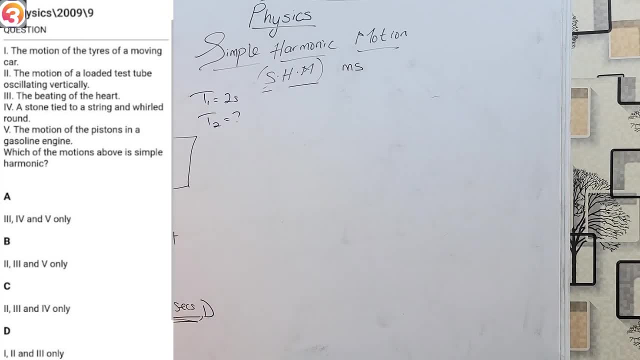 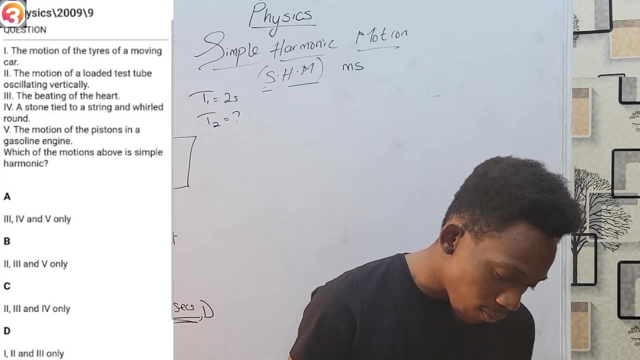 number 2. the motion of a loaded test tube oscillating vertically. number 3. beating of the heart. number 4. a stone tied to a string and whirled around, and number 5.. 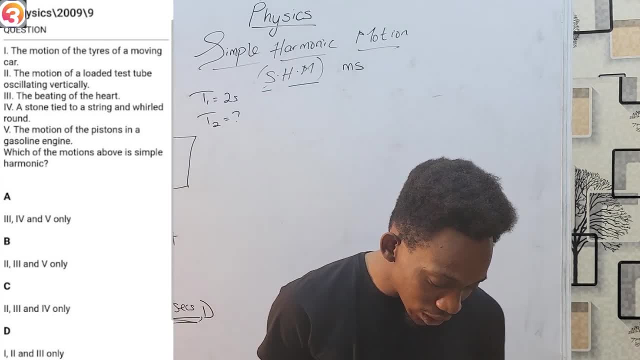 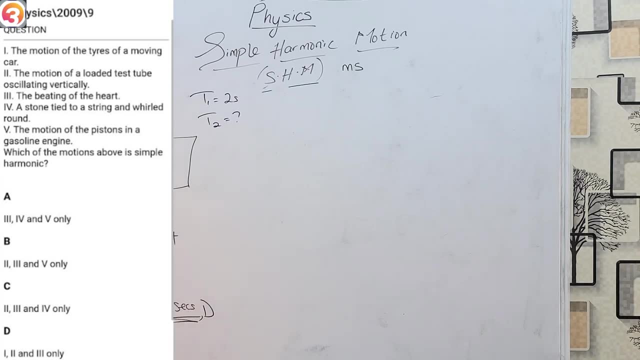 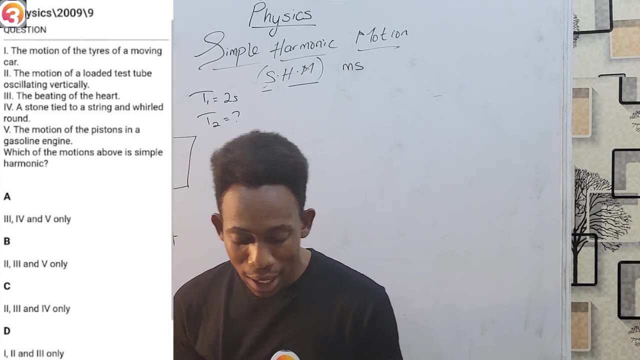 the motion of the pistons in a gasoline engine. which of them, or which of the above, is simple harmonic? now for simple harmonic motion. what do we know about it? it must simply be oscillating. 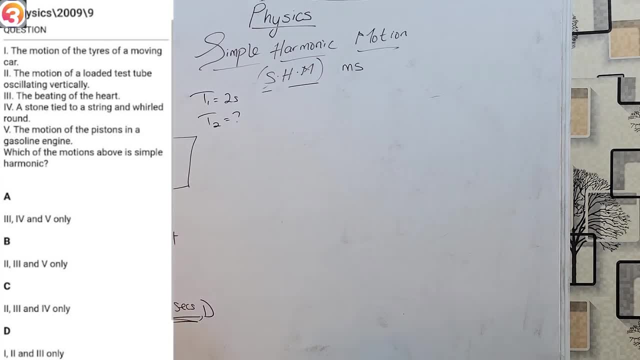 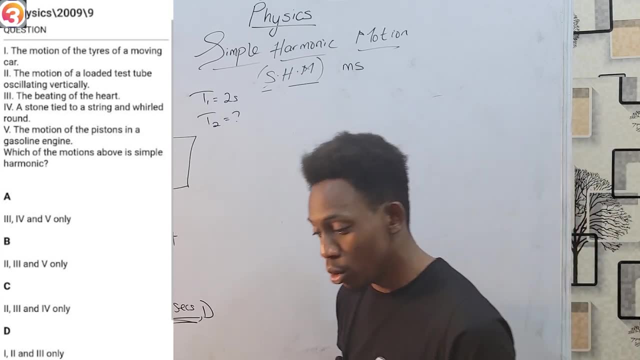 to and through right, and the key thing, though, which means it is not always arbitrary, is because you have now got the acceleration which was in your formula, or your definition, rather being proportional. 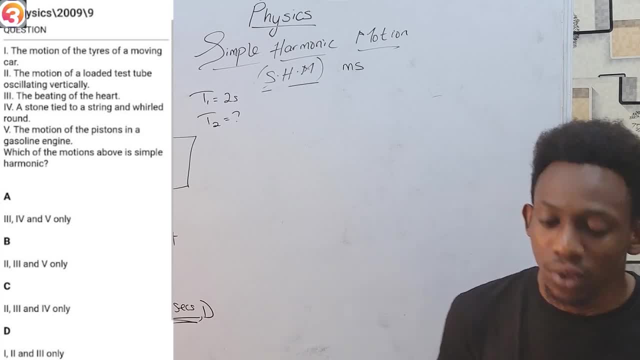 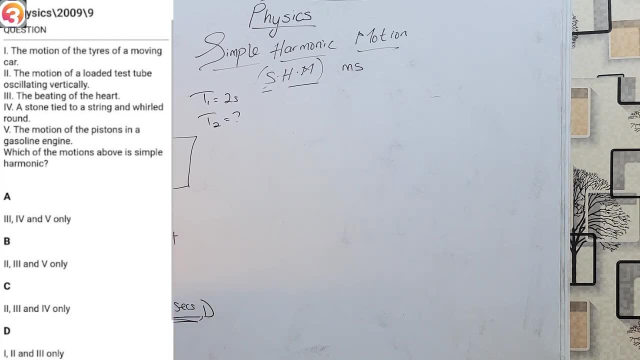 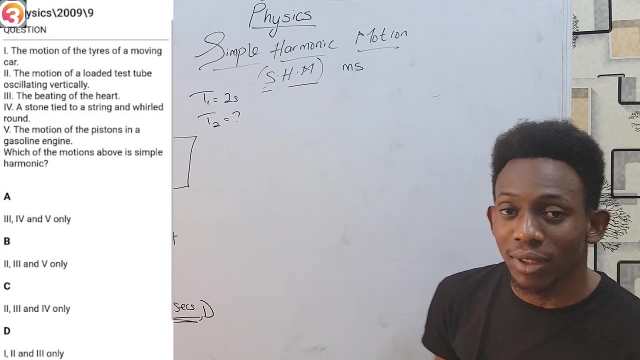 and it's always been directed to equilibrium points. so motion of the tyres of the moving car, that is rotational motion. that is rotational next up motion of a loaded test tube oscillating vertically. 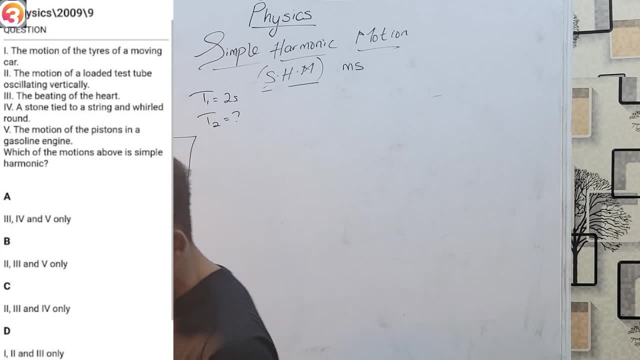 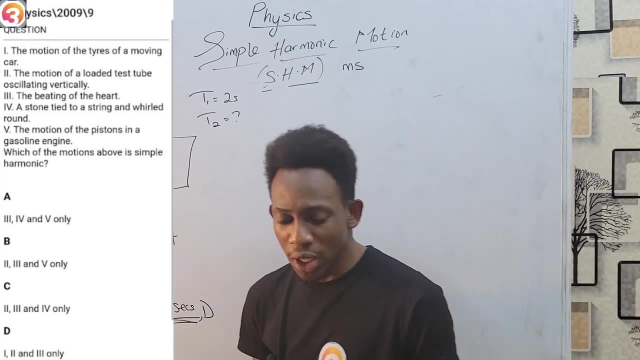 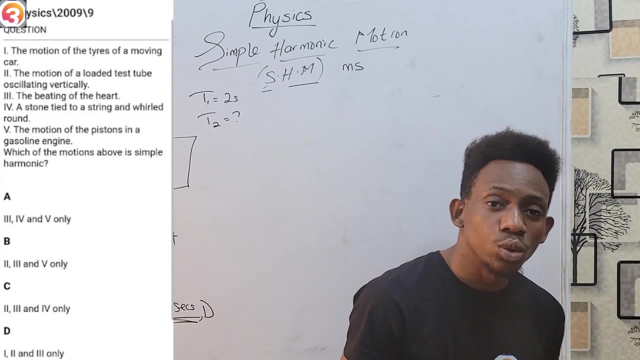 that's the victory motion, then beating of the heart, simple, harmonic. a stone tied to a string and whirled around, that's secular. then motion of the pistons in a gasoline engine. 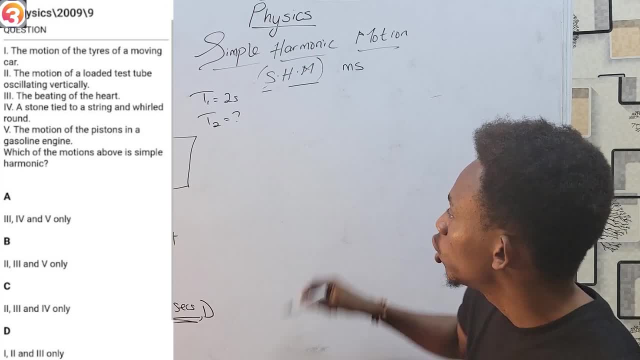 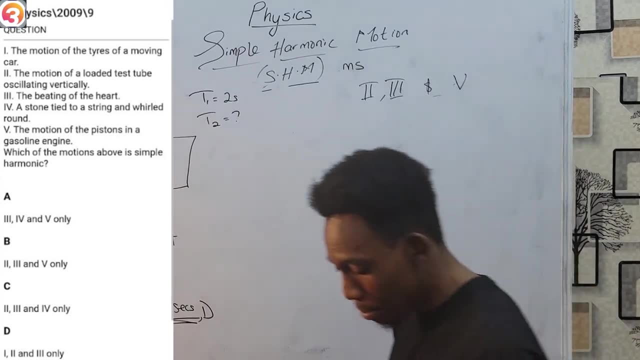 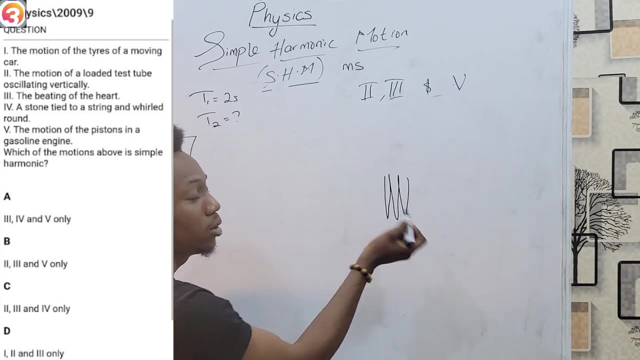 also simple, harmonic and vibratory. therefore, our answers must be two, three and five because, again, a loaded test tube oscillating vertically is going up down, up down. equivalent position is somewhere in the middle. 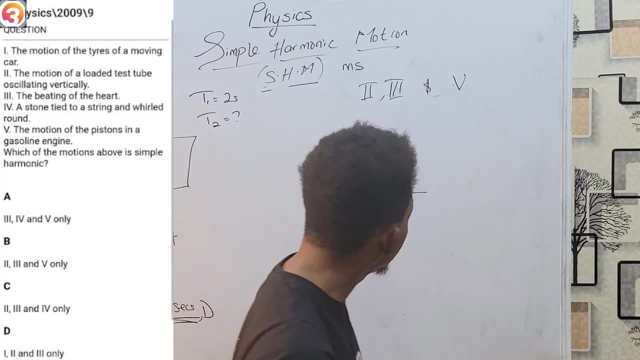 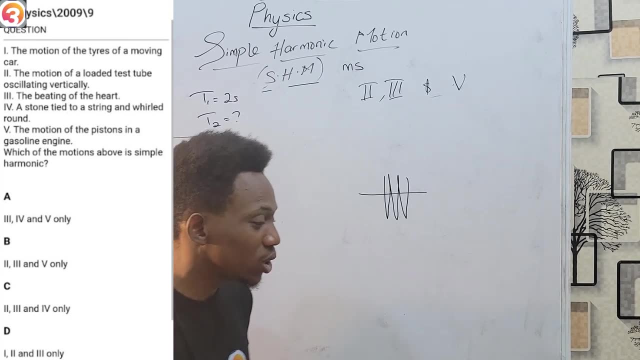 and is oscillating, simple, harmonic beating of the heart, then pistons in a gasoline engine, just like that. so please note, in most cases vibratory motion is usually simple, harmonic. 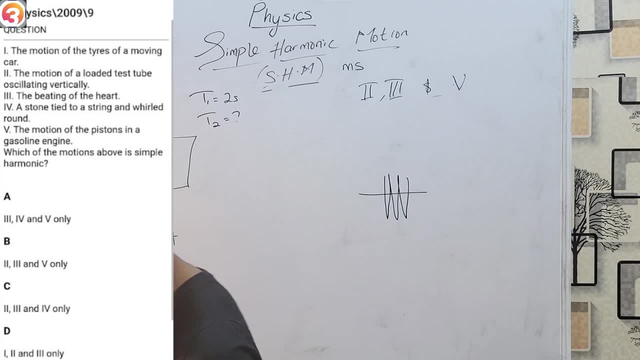 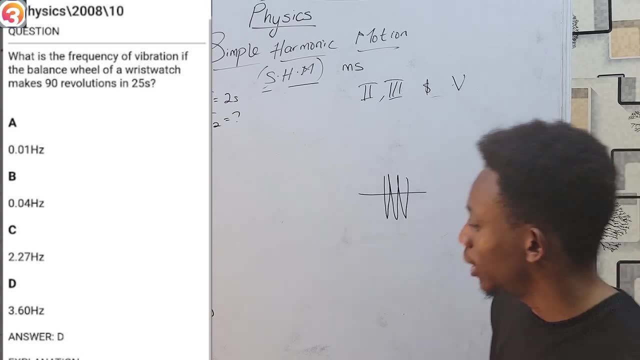 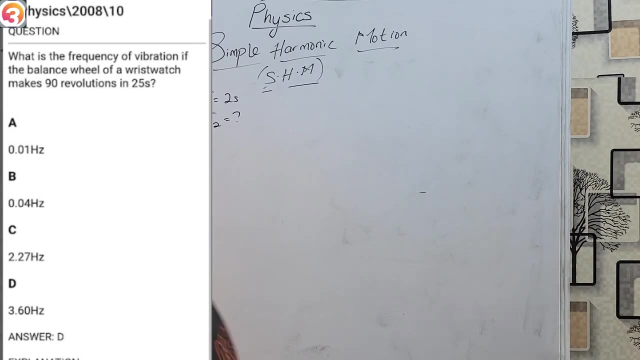 so my answer here- two, three and five- must be option B, see so move on. .2008 question 10.. and for this one there is a bit of calculation. so .2008 question 10.. 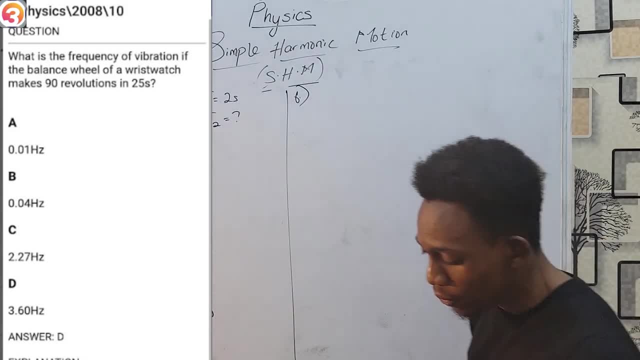 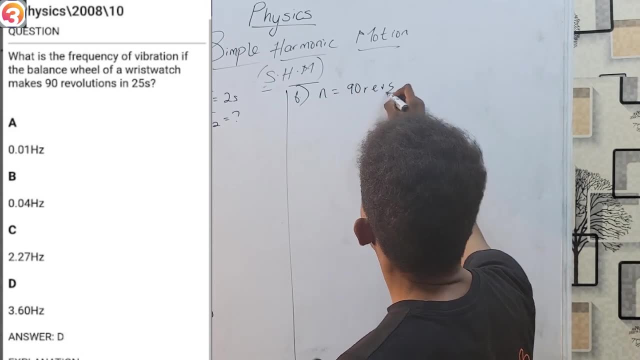 and now i'm going to go more in detail in the sixth solving example. what is the frequency of vibration if the balance wheel of a race watch makes 90 revolutions in .25 seconds? this is very easy. 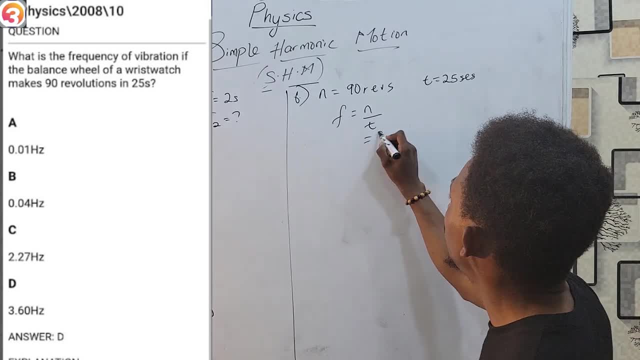 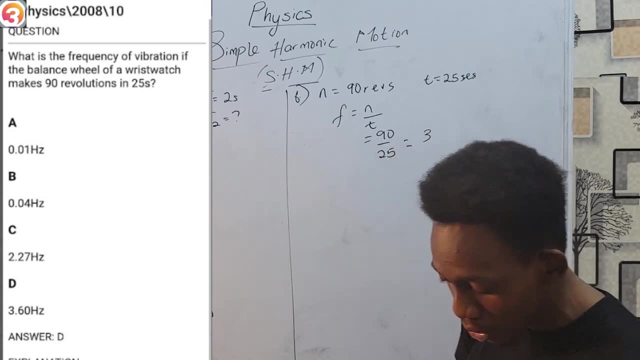 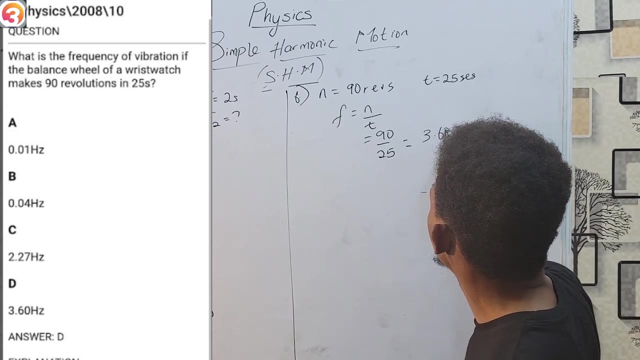 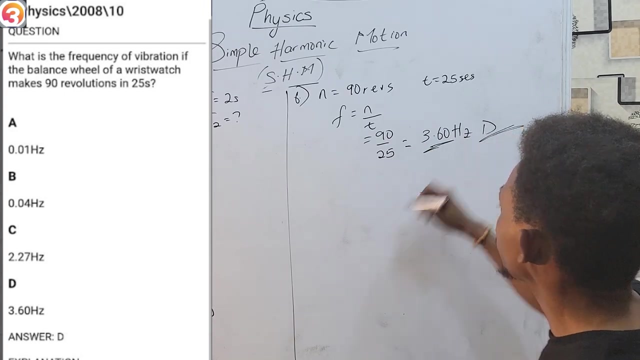 frequency is the number of revolutions over time. so simply 90 divided by 25.. and if you press that you should be getting i know it is three. let's confirm the decimal places divided by 25. three point six, zero, eight. and that if option works, option D see. 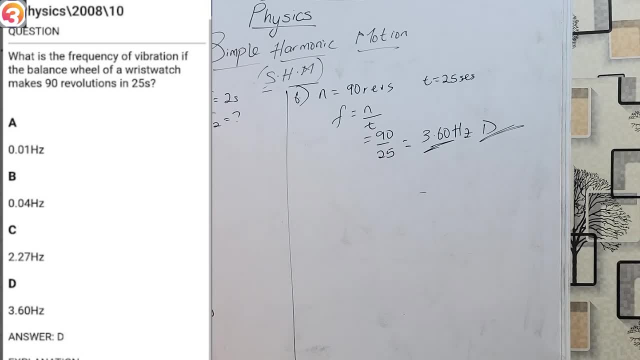 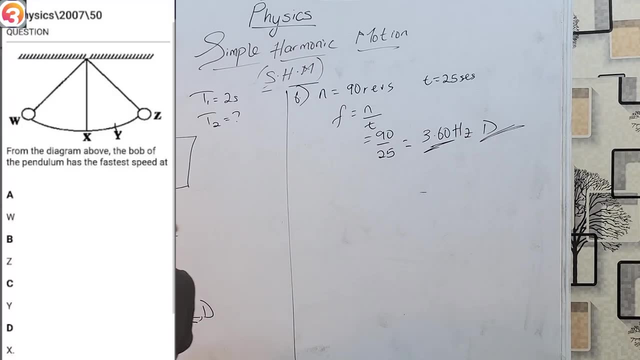 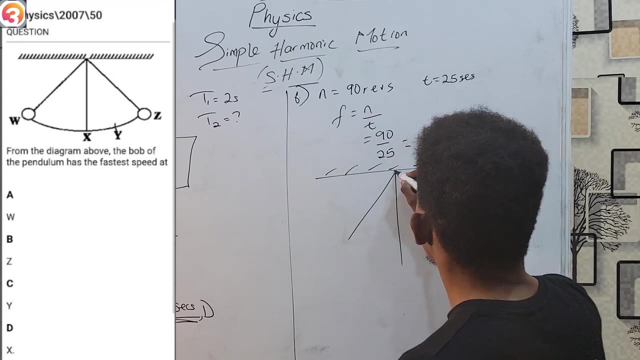 this one is very short and simple: run eight questions in. I will move on to the X 2007, number 50. in this one we have a diagram which we should be able to remember from our explanations. do diagram something like this: and this is Bob, Bob, Bob here. this is Z, this is Y, this is X and this is W. question is: 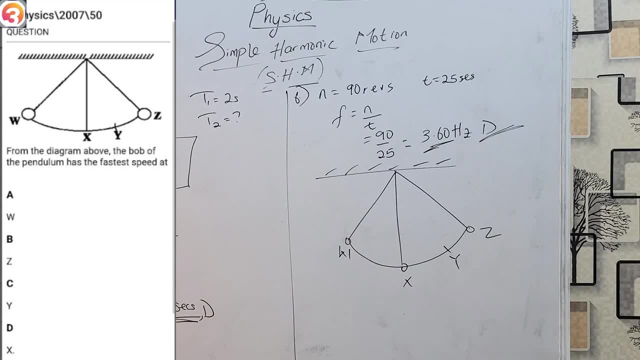 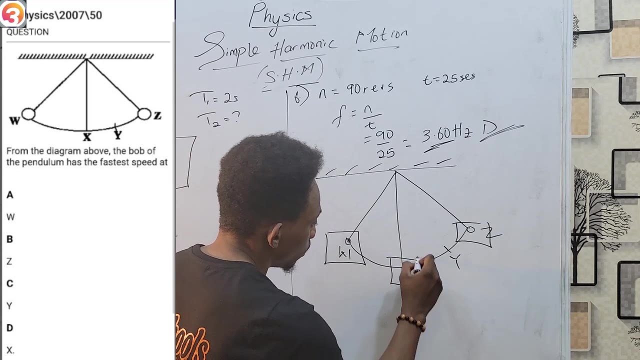 where is the speed fastest? I remember from the explanations we said that point W, right here this guy is not moving, so the speed is minimum. this video is also a minimum. then, right at the equilibrium position is where you have maximum speed. common position: you have maximum velocity. that is what you have maximum. 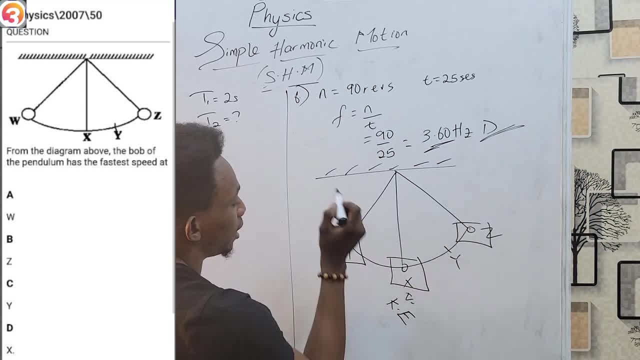 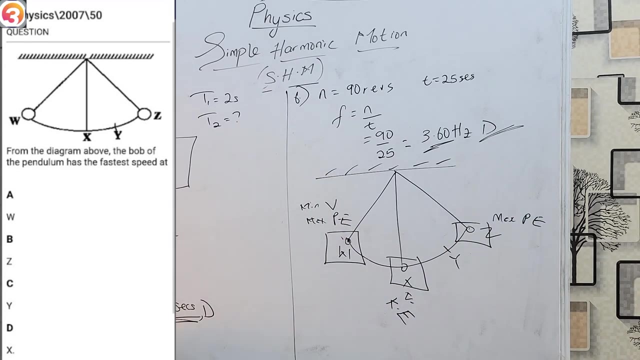 key e, while at these two points, W and Z, you're having minimum velocity and, as such, maximum potential in it. so your point five, not as much Monday, that would potential and and etic energy. okay, next off 2001 question: mine does not. one question nine: 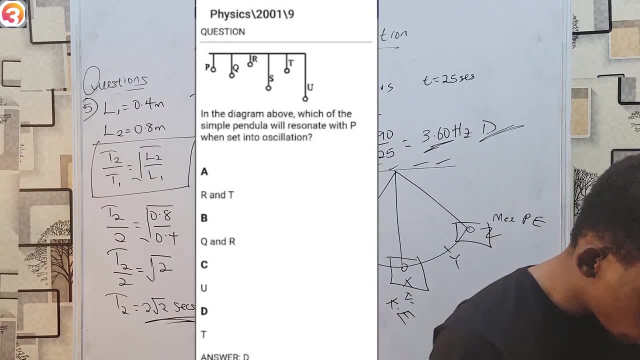 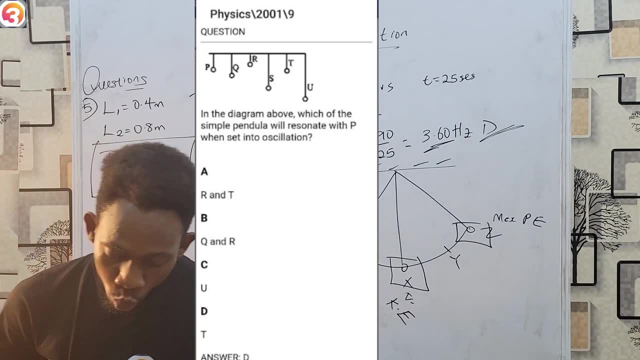 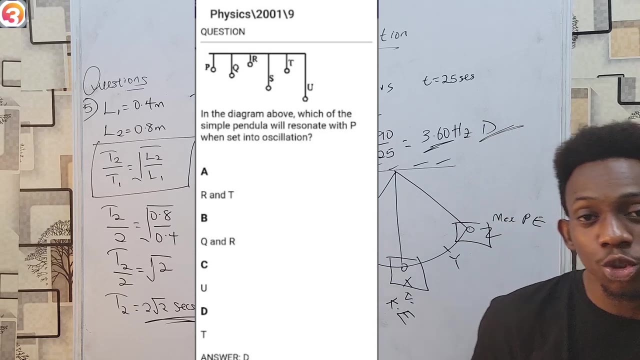 then on you consider diagram on your screen, on your Trees, cruise, jump back and there some even asks in the diagram which of the simple pendula will resonate and with P, when set into oscillation? now, please remember resonance, they should be having the same frequency and, as my way, frequency depends. 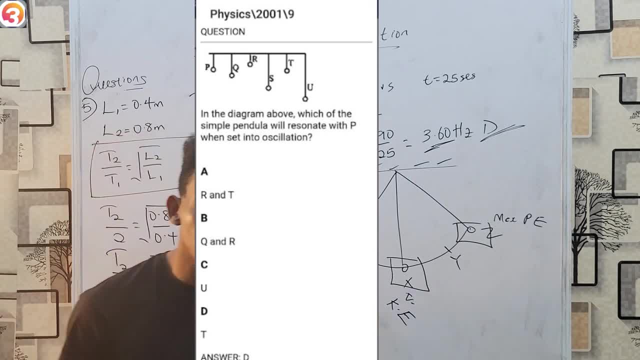 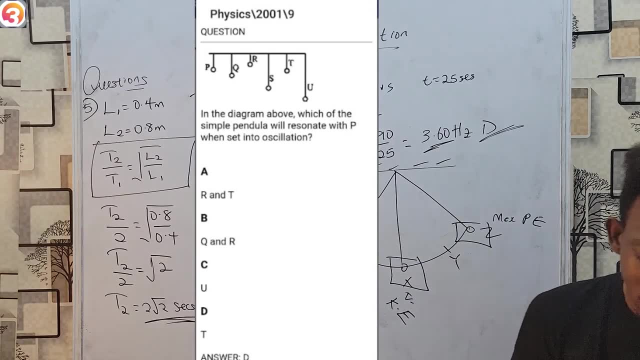 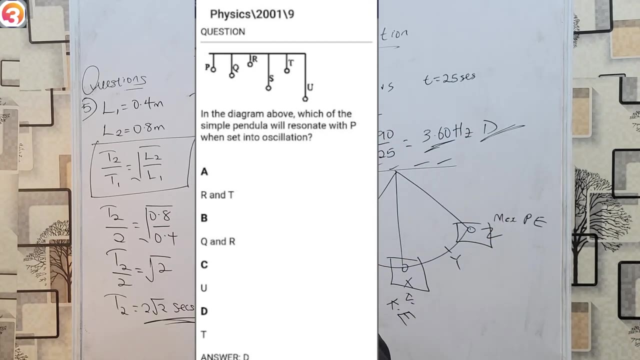 on the length and, as such, they're simply asking you which of them has the same length as p and, looking at the diagram, very simply, you can all see that the only one whose length is the same as p is t. so my answer is simply: d, option d: t. that's all and that is clear. we shall take. 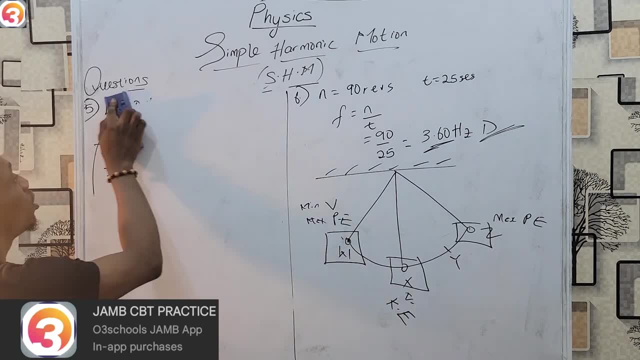 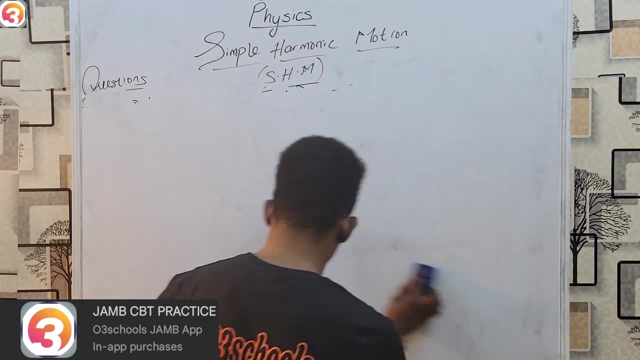 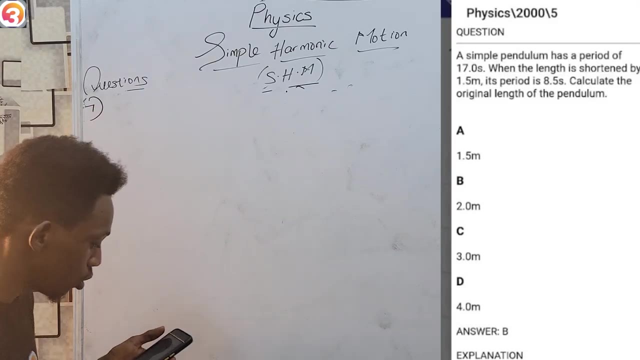 one last question, just one more simple question on super money commission, and we shall be able to call it a day on this topic. okay, this one is from the year 2000, question number five. yes, 2000 question number is five. a small pendulum has a period of 17 seconds. 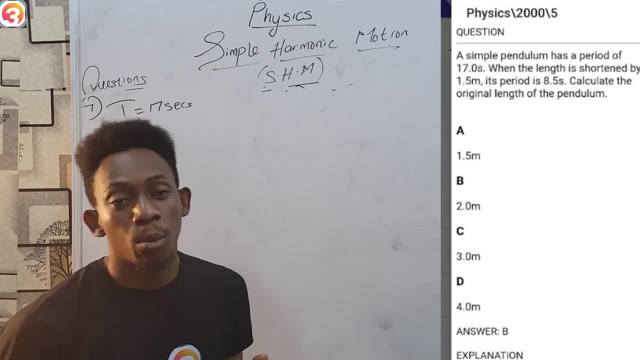 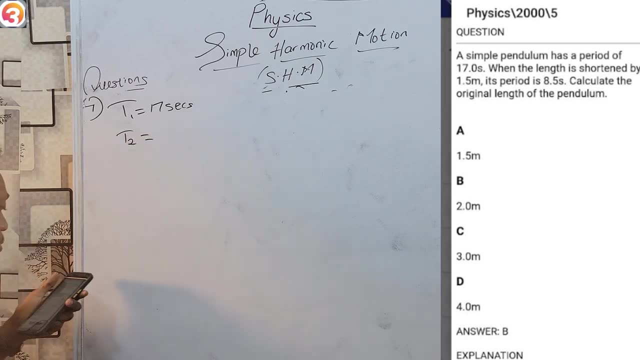 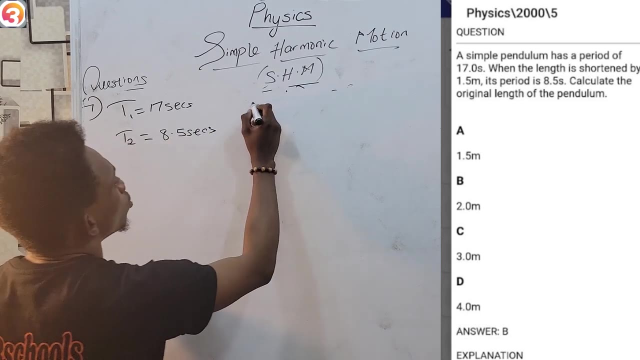 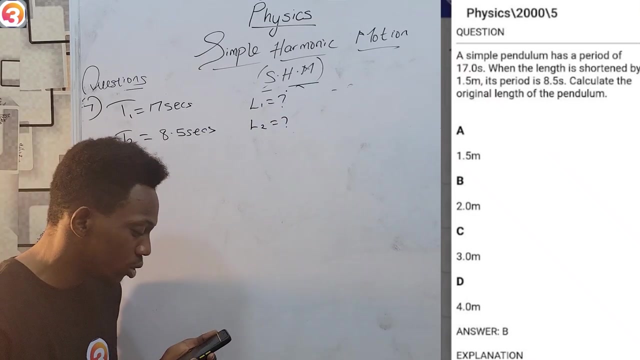 when the length is shortened by 1.5 meters. again now i read a. i'm comparing, so i must have t1, then t2. the period is 8.5 seconds. now, however, what about my l1 and l2? at no place in my question was i told what l1 was. so i can put x there if i so desire, or any. 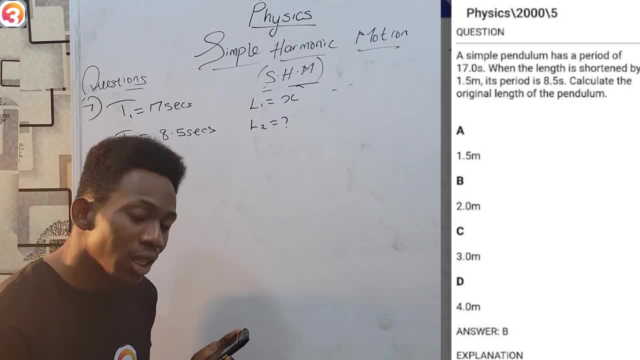 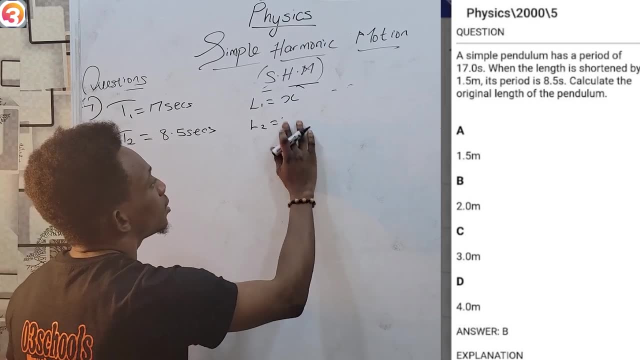 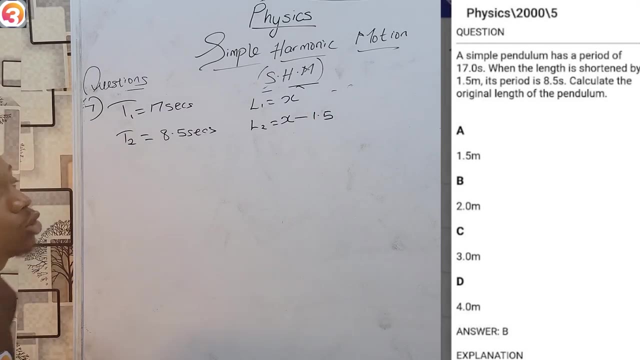 other letter, but i'm down to that. in the second case the length is shortened. shortened means something is removed, minus by 1.5, indicating that i take this length from before and i remove 1.5 meters. so it's t1, t2, l1. 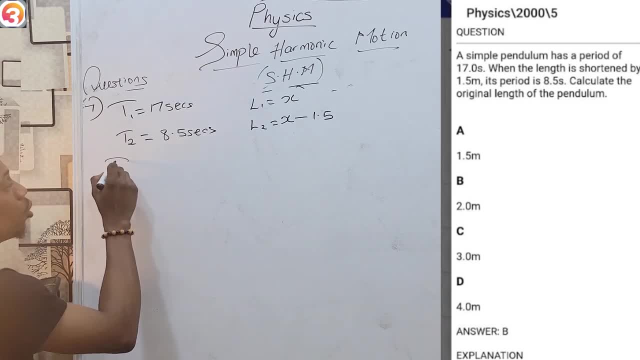 and l2 and, as before, your formula becomes: t2 over t1 equals square root of l2 over l1. um c2 is 8.5 and t1 is 17.. coming on, l2 is x minus minus 1.5 and l1 is x. okay, if i look, hear this can cancel out. 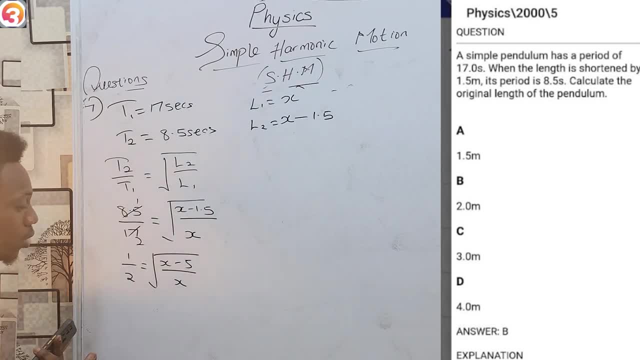 1 and 2, so one over 2 equals square root of x minus 5 over x. now, obviously, what's the next thing i can do after we move the square root from this equation? so square both sides. that gives me loading in SE qu��. 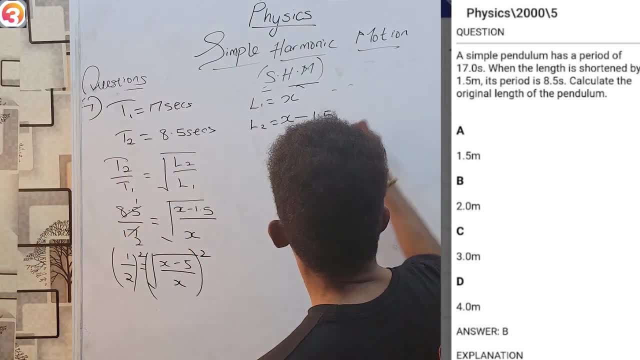 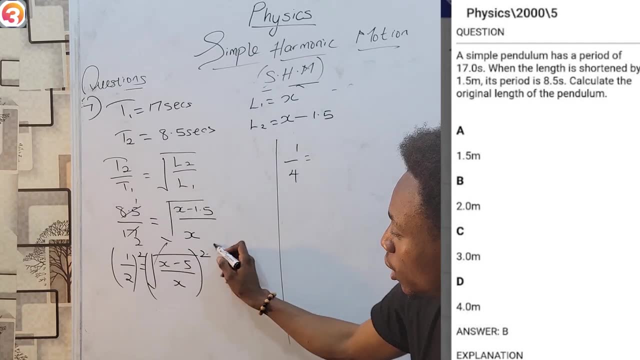 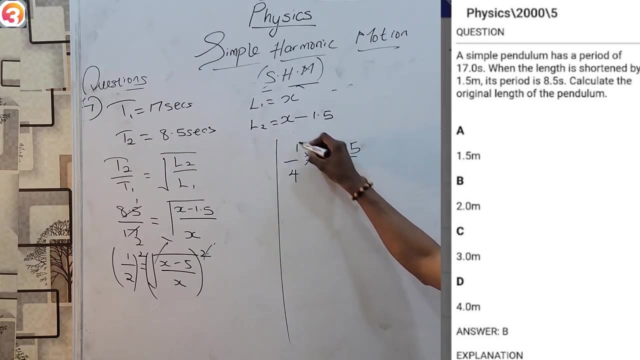 one in SE is pi over 3, One squared is obviously still one and two squared is going to be four. Then this square cancels the square root here: X minus five over X. Of course. multiply X times one, X, four times X minus five. 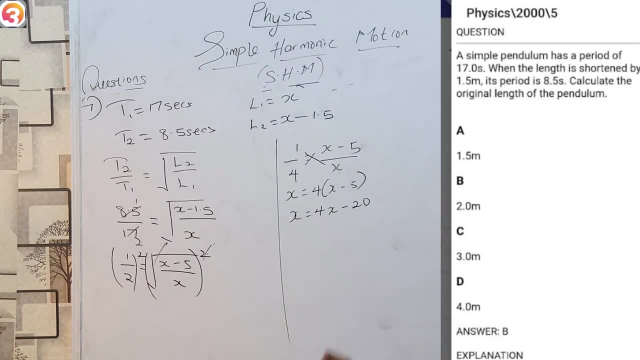 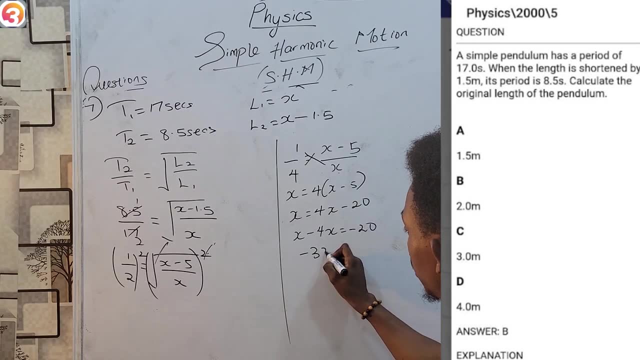 That becomes four X minus 20.. Collect your lag terms: X minus four, X equals to minus 20.. X minus four, X is minus three. X equals to minus 20 over minus three over minus three. And what does that give me? That'll be 20 over three. 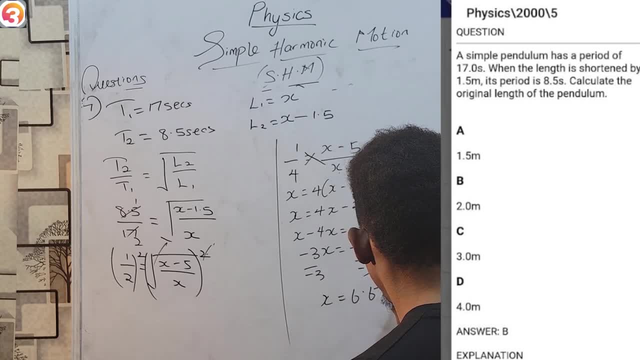 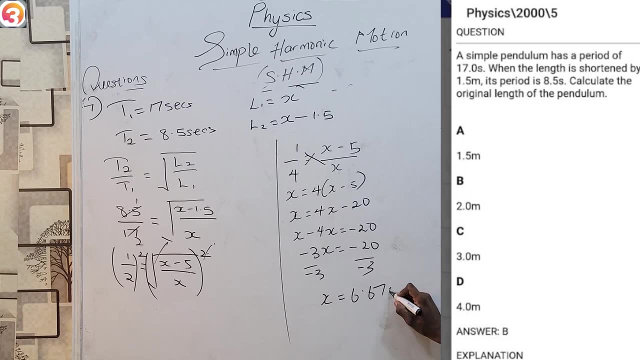 which gives me 6.67 seconds. And now on getting this answer. oh, by the way, please, we're sorry for the distance of the meter, But if you look at the options, you can realize this is not in our options. 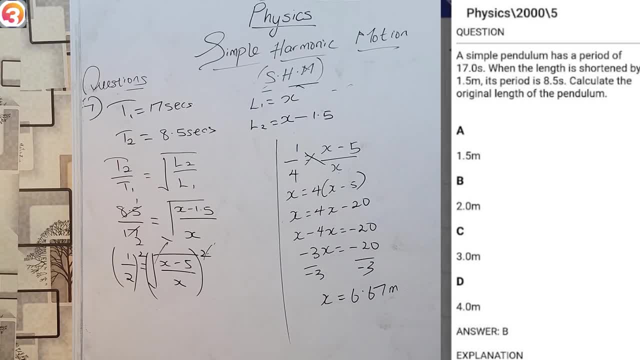 What can we do? This is one of those times. I've always told you: When you make a mistake, do not panic and rush to start over. You can simply look through your question and easily identify your mistake, Like from here: okay, we have a formula, correct.